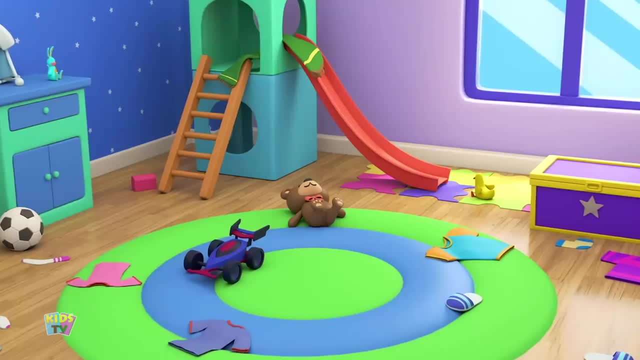 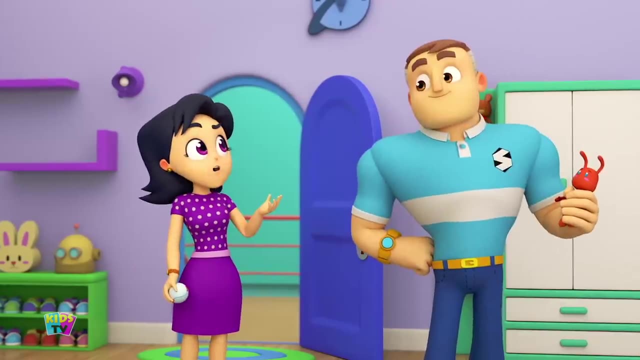 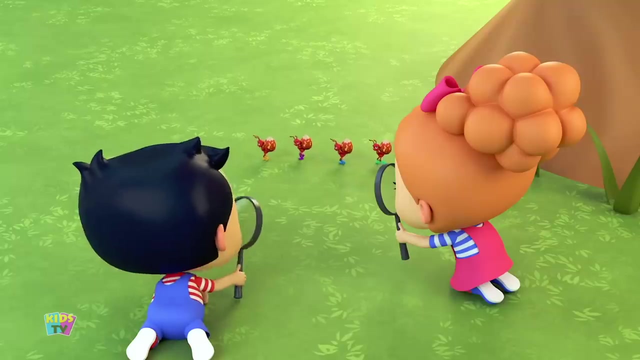 Oh my, I asked Huggy and Buggy to tidy their room before going out to play Those kids. Do you know where they are? I think I saw them in the backyard. I'll go find them, Jen. Wow, it's so cool to look at all the little insects. 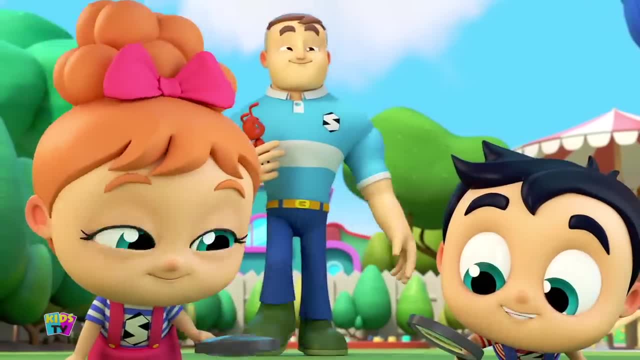 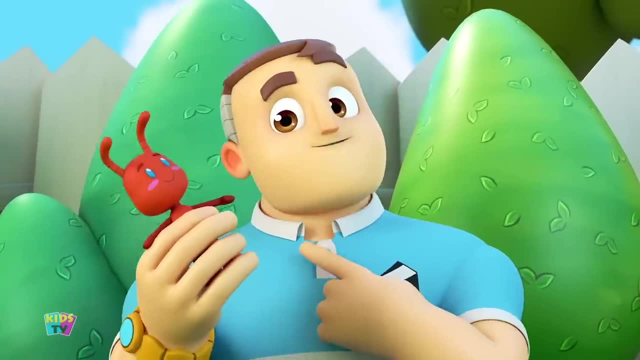 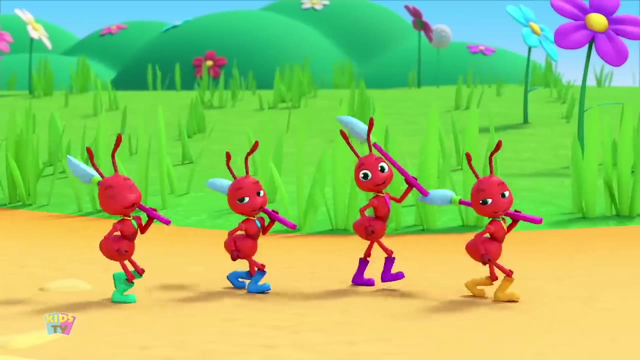 Yeah, the ants are my favorite. My favorite is the grasshopper. That reminds me of a story And I think this might be a good time to tell it to you: The ants go plowing in the field. Hi-ho, Hi-ho. 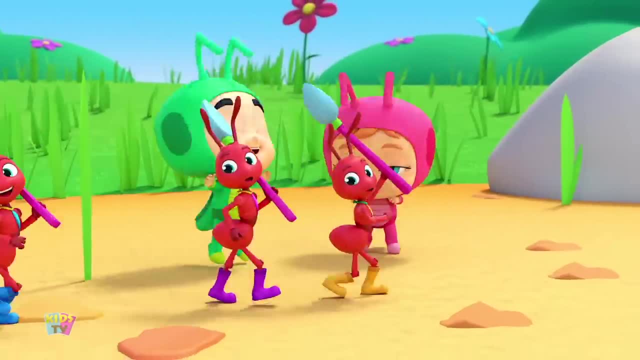 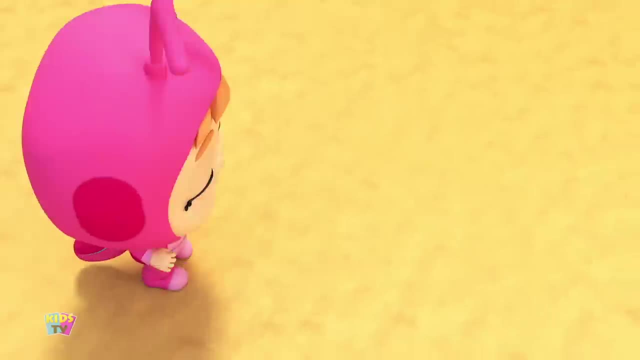 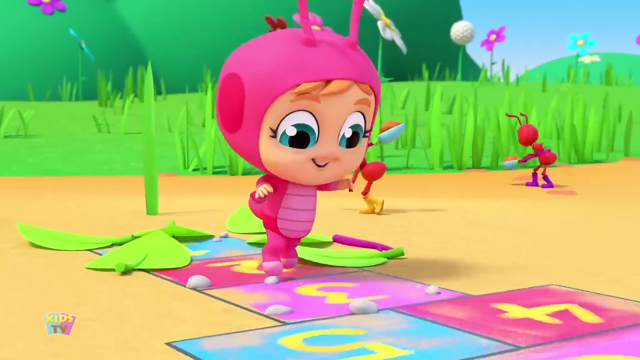 The ants go plowing in the field. Hi-ho, Hi-ho. The ants go plowing in the field. The grasshoppers do cartwheels And all they do is play. while the ants work all day, The ants go planting in the spring. 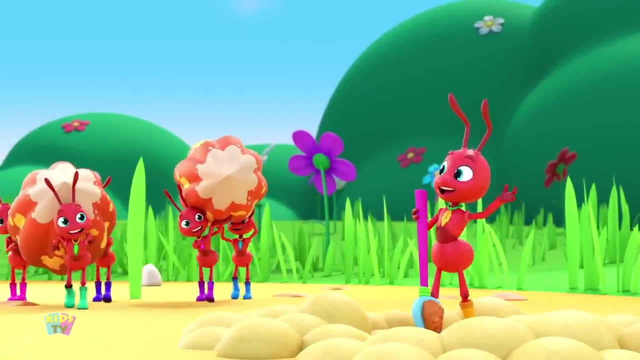 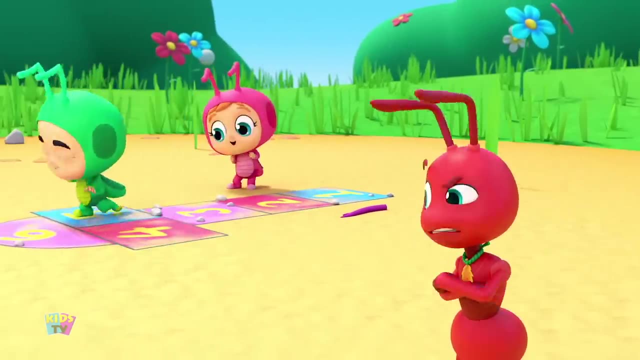 Hi-ho, Hi-ho, The ants go planting in the spring. Hi-ho, Hi-ho, The ants go planting in the spring. The grasshoppers don't do a thing, And all they do is play, while the ants work all day. 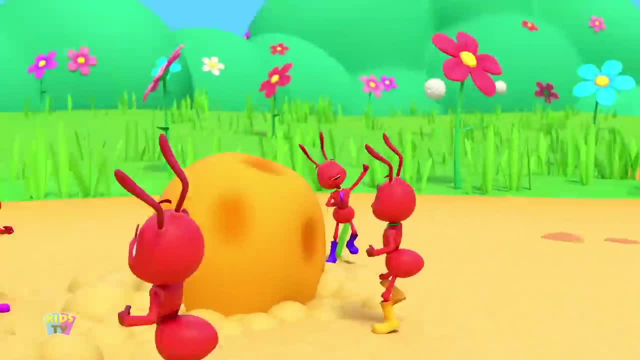 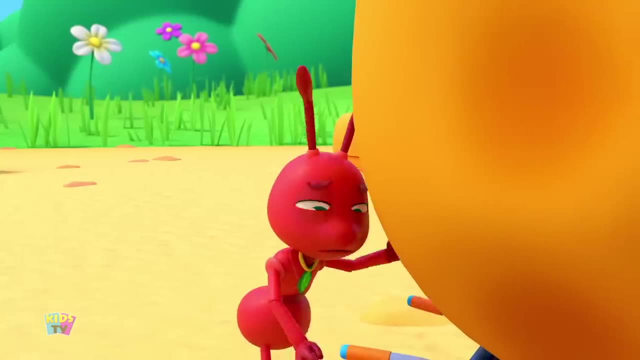 The ants go digging in the sun. Hi-ho, Hi-ho, The ants go digging in the sun. Hi-ho, Hi-ho, The ants go digging in the sun. The grasshoppers dance for fun, And all they do is play, while the ants work all day. 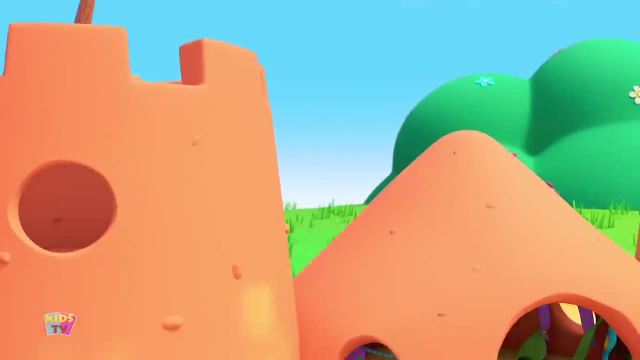 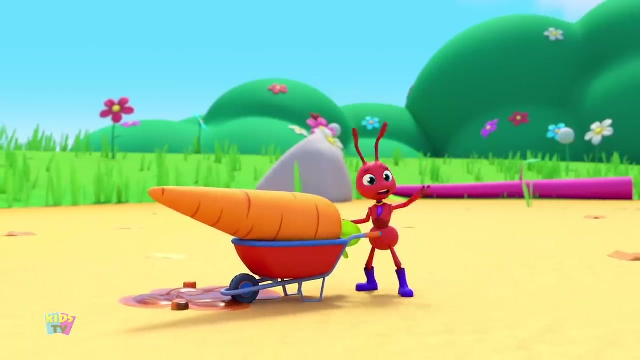 The ants harvest in the fall. Hi-ho, Hi-ho. The ants harvest in the fall, Hi-ho, Hi-ho. The grasshoppers don't help at all, And all they do is play, while the ants work all day. 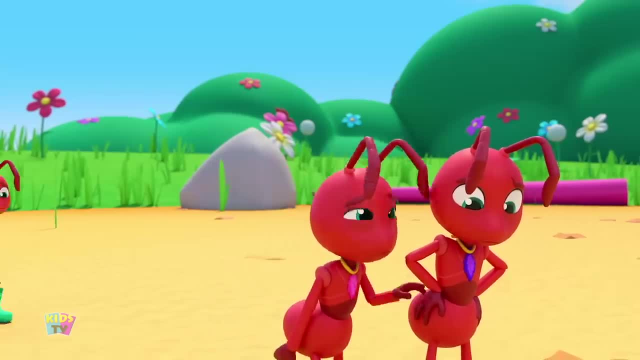 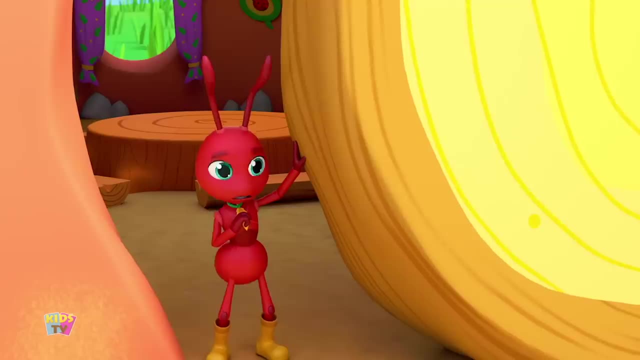 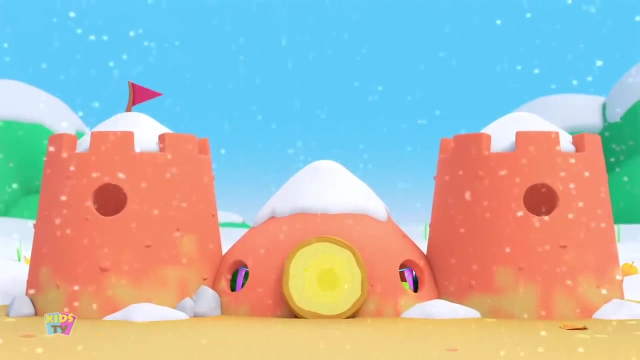 And all they do is play while the ants work all day. The ants go in when winter comes. Hi-ho, Hi-ho, The ants go in when winter comes. Hi-ho, Hi-ho, The ants go in when winter comes. 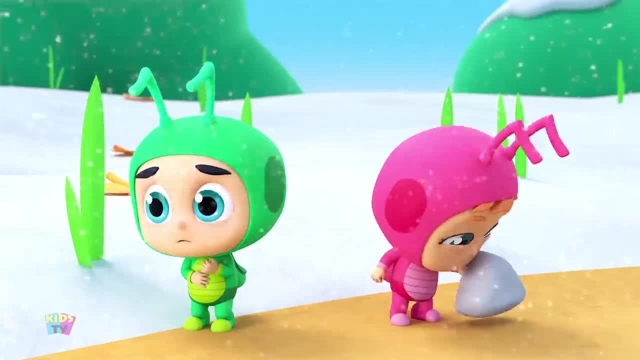 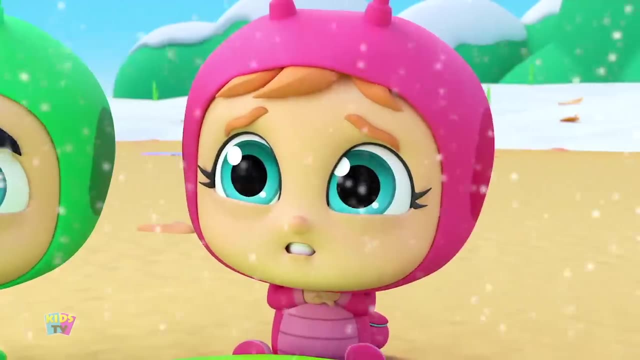 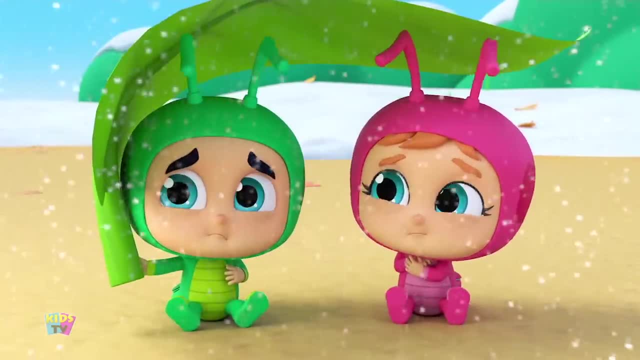 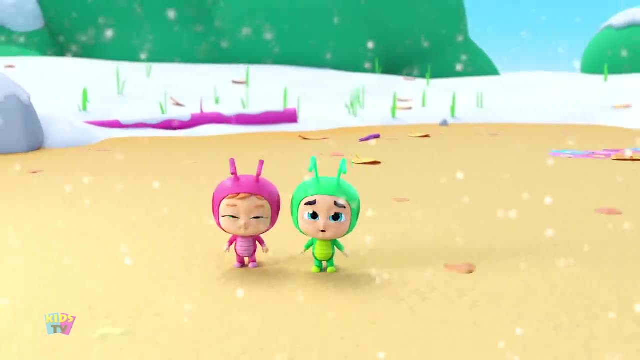 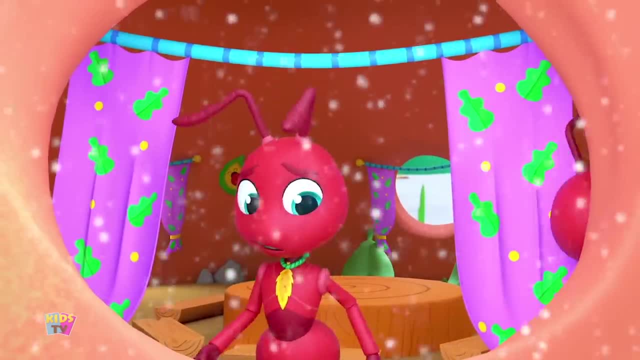 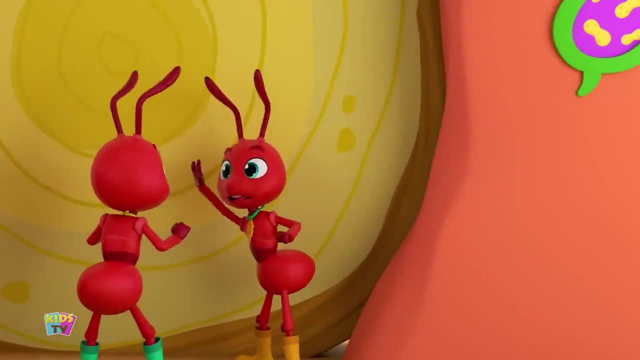 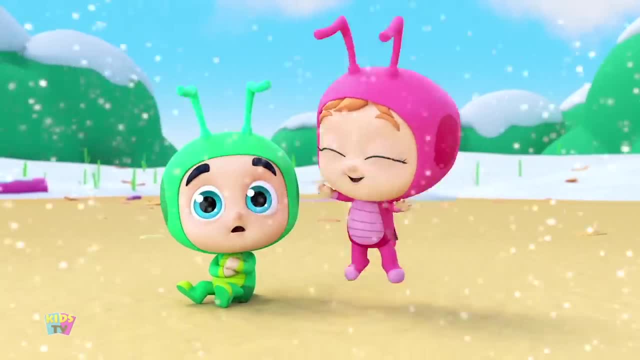 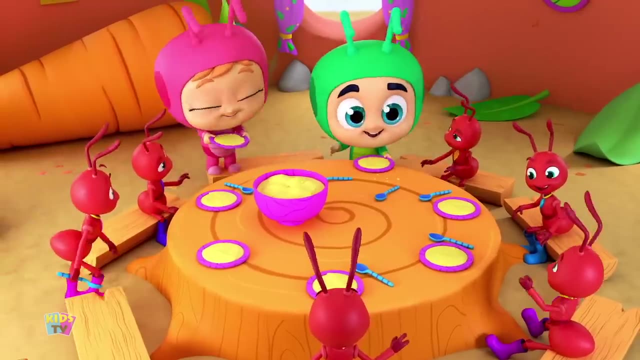 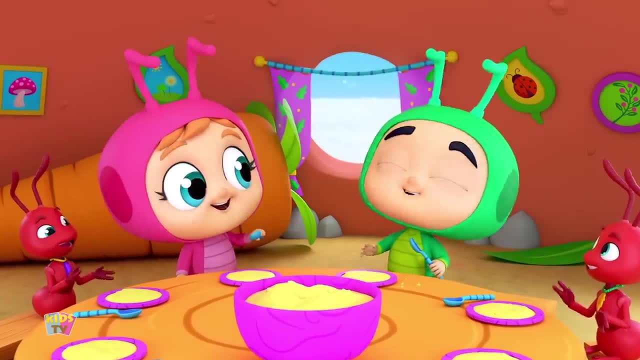 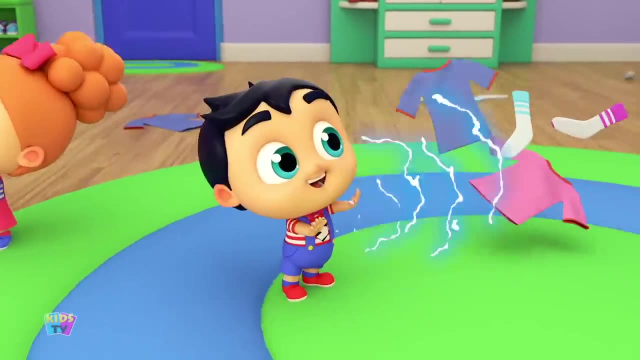 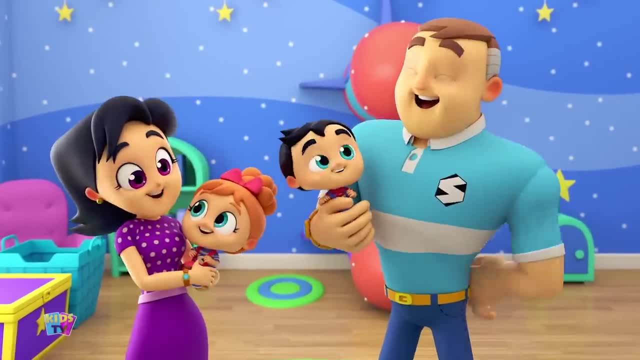 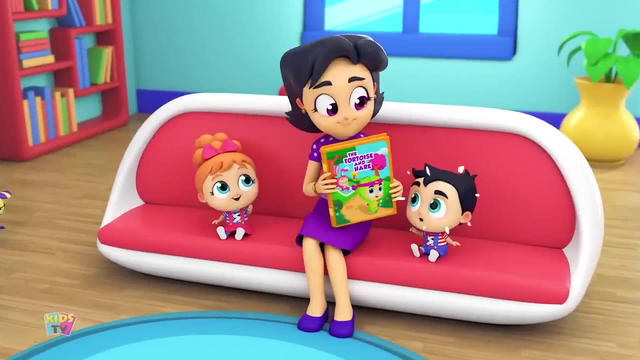 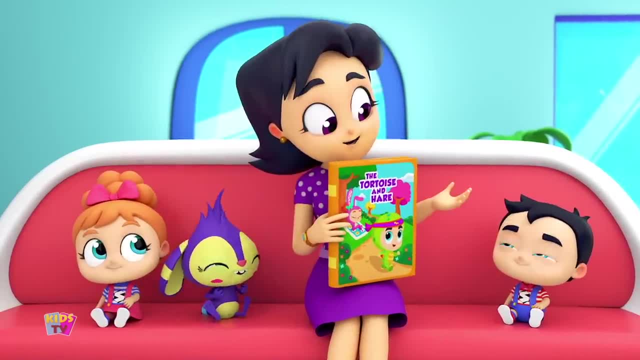 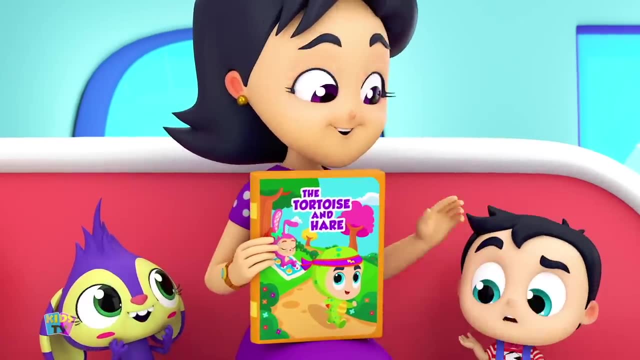 That says tortoise Huggy. What's a tortoise? A tortoise is a very big turtle. And what's a hare? A hare is a kind of rabbit. Why don't they just call the story The Turtle and the Rabbit? 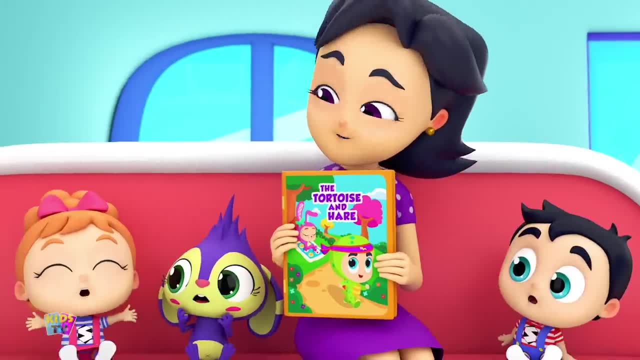 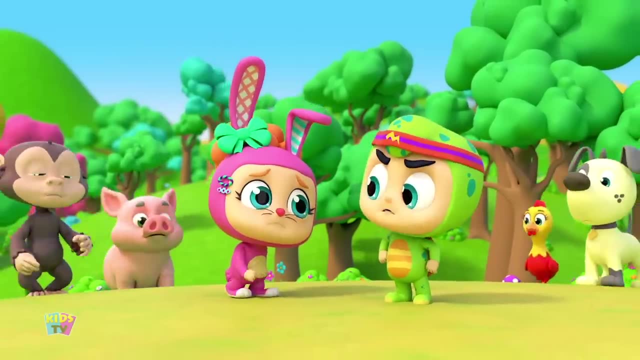 Well, that's a very good question. Can we just read the story? Hum, Alright. then One day the hare was teasing her friend the tortoise And she read the story. He wasn't being very nice. The boastful hare could run really, really fast. 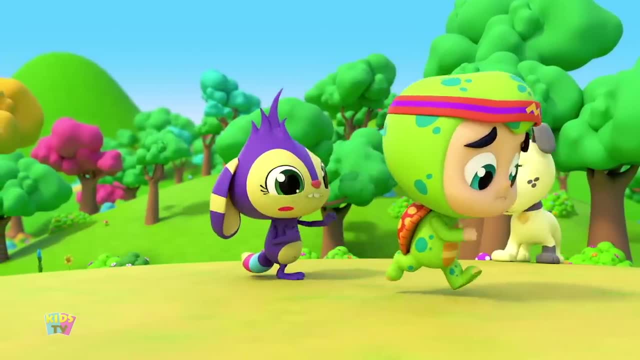 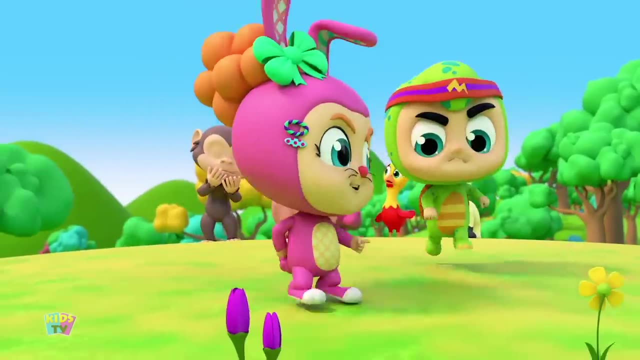 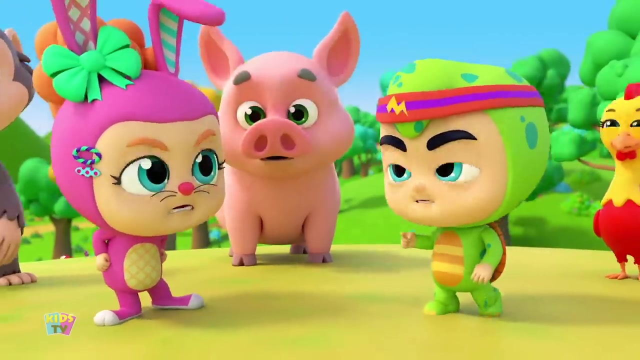 But the kind old tortoise was very, very slow. To be so slow, it must be sad, It must be very, very bad. The tortoise, he got pretty mad The day of the big, big race. Well, let's have a race, said he. 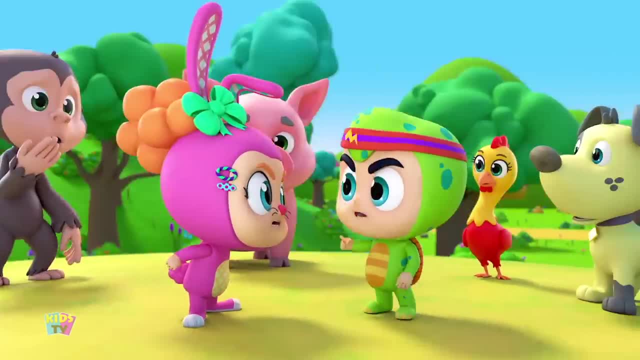 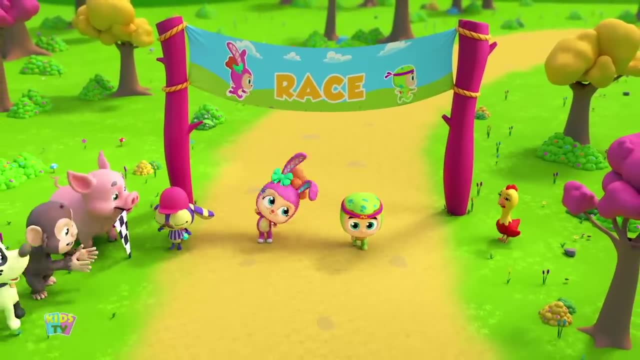 You're too slow, You can't beat me, I can, You can't. Well, let's just see The day of the big, big race. Pinky said: go the hare. he flew Over the hill and out of view. 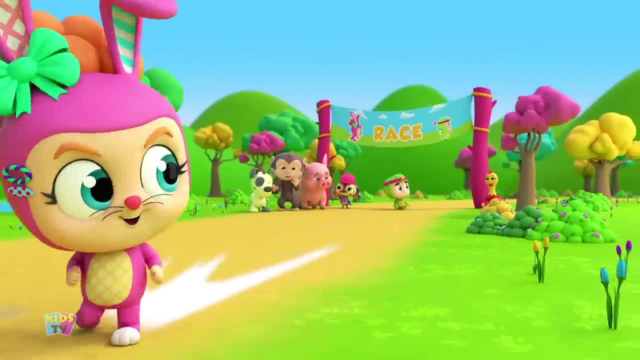 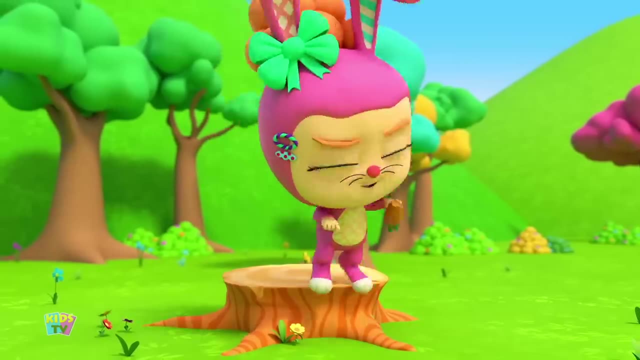 It looked like tortoise was stuck in glue The day of the big, big race. The hare, she laughed Ho ho ho. That old tortoise is slow, slow, slow. I can't be beaten. No, no, no. 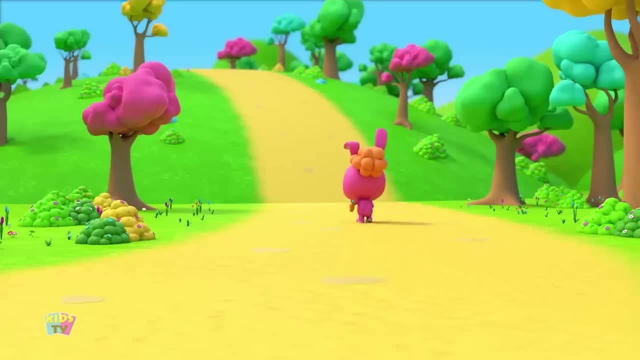 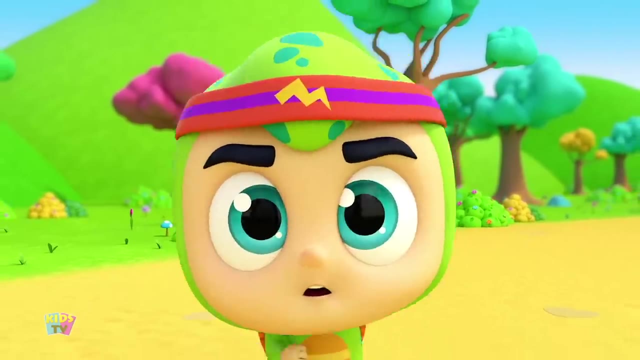 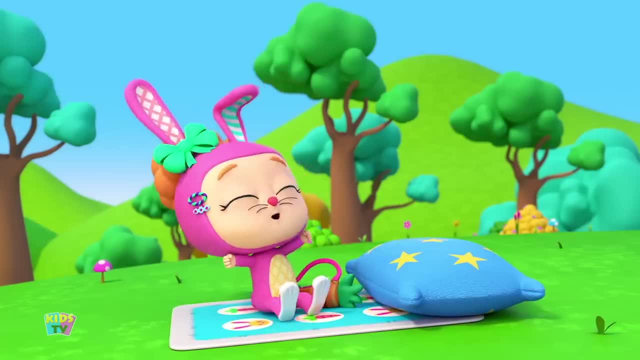 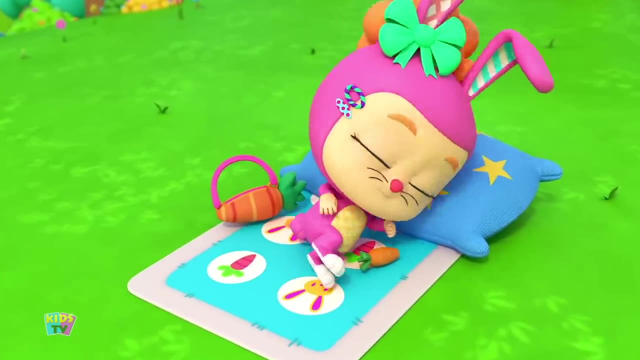 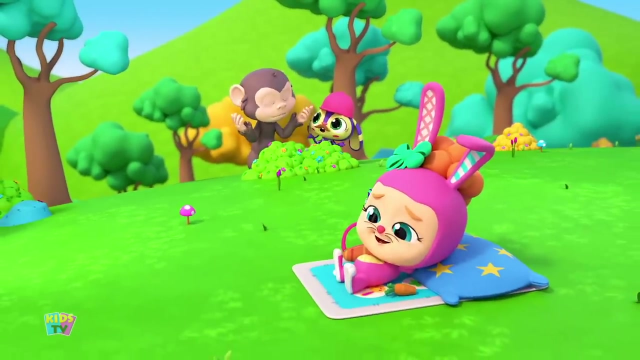 The day of the big big race. I am miles and miles ahead. I think I'll take a nap, She said. in a carrot patch she made a bed. The day of the big, big race. Just five minutes, not a minute more. 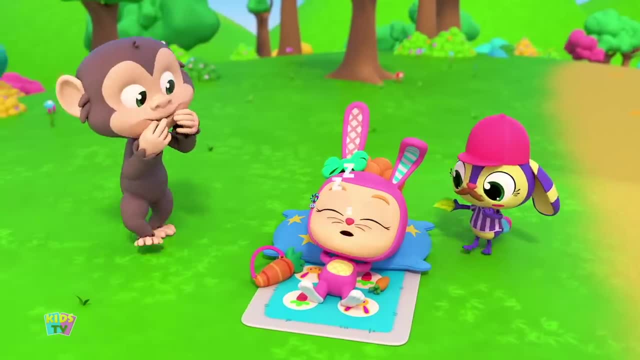 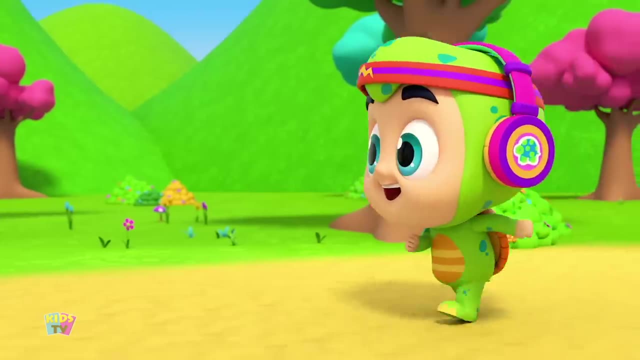 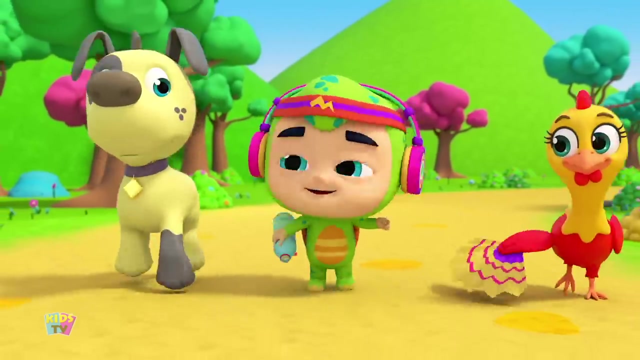 And it wasn't long before The boastful hare began to snore. The day of the big, big race. Slow old tortoise trudged along, Whistling a happy song. He was slow but he was strong. The day of the big, big race. 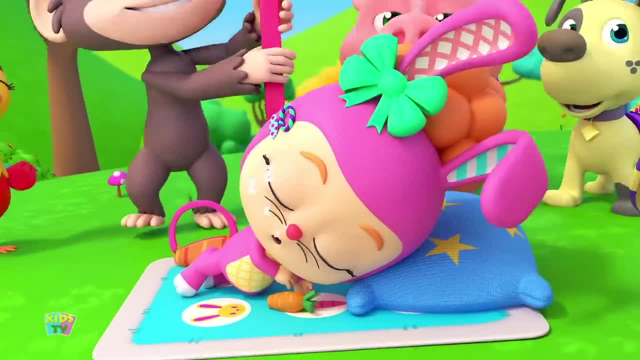 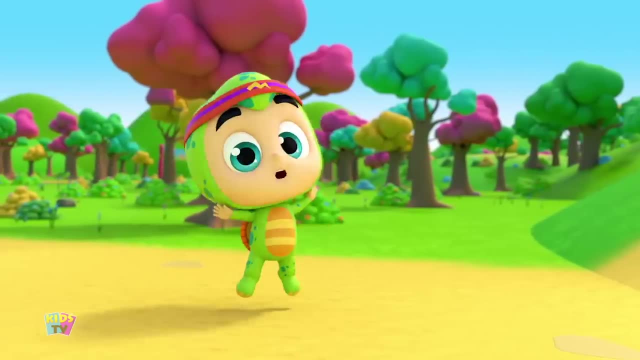 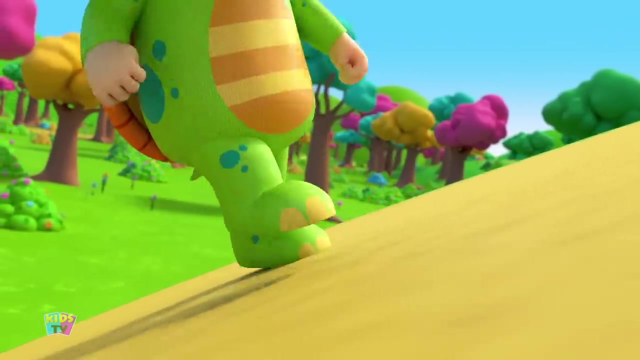 I won't give up. no, no, no. His confidence began to grow. Come on, legs, let's go, go. go The day of the big, big race. Even when the hill was steep, Still he climbed and still he creeped, And still the hare was fast asleep. 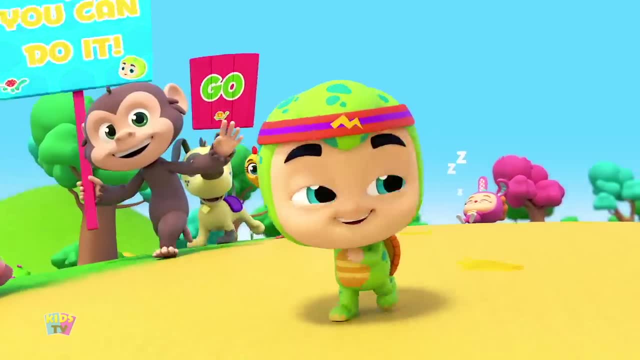 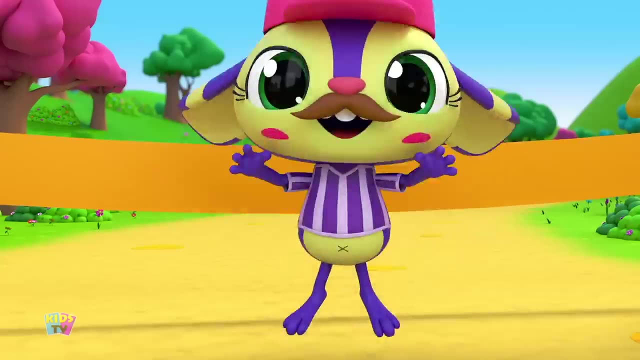 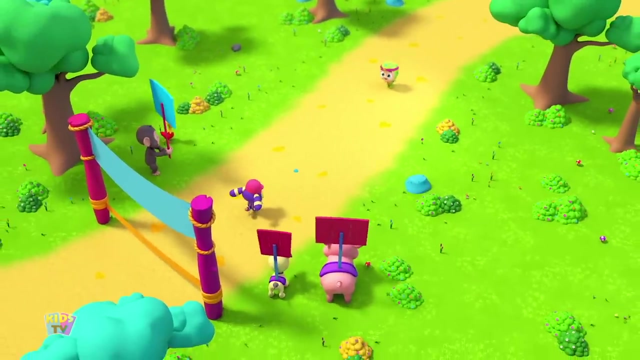 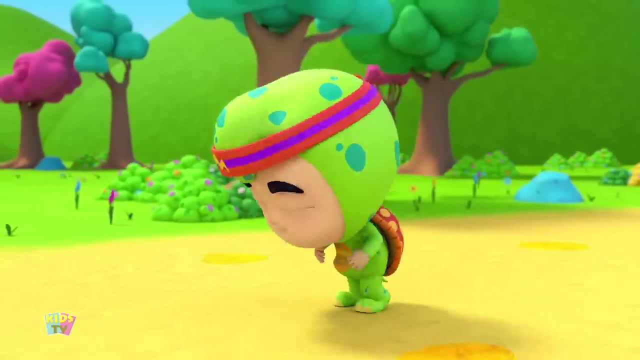 The day of the big, big race. Finally, he passed the hare, Fast asleep and unaware, The finish line. I'm almost there, The day of the big, big race. The crowd began to cheer and cheer As slowly, tortoise, he drew near, The hare, awoke and said: 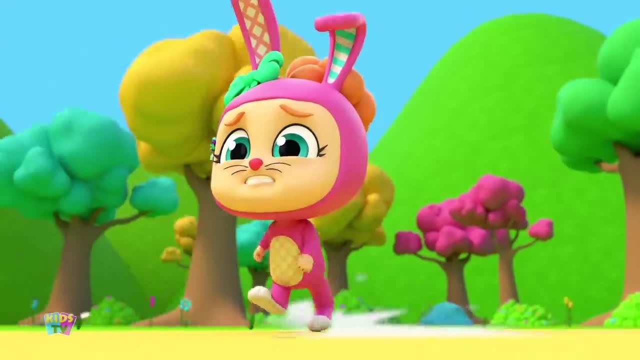 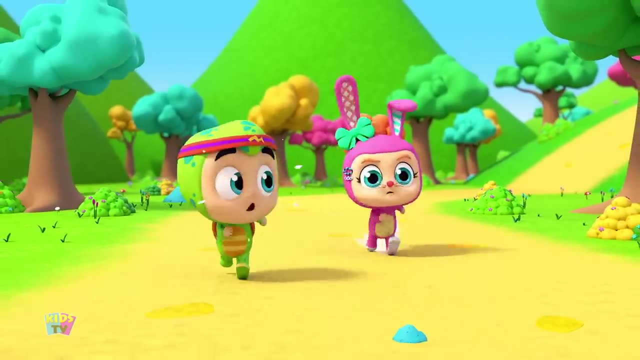 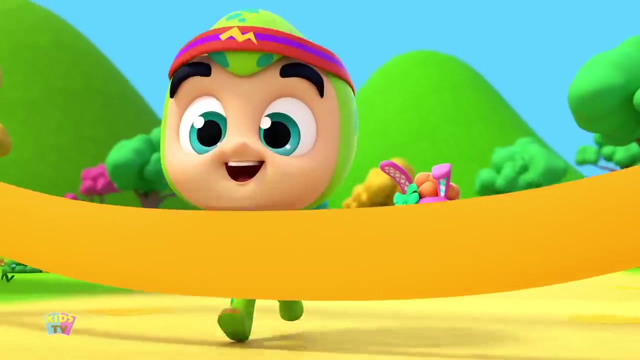 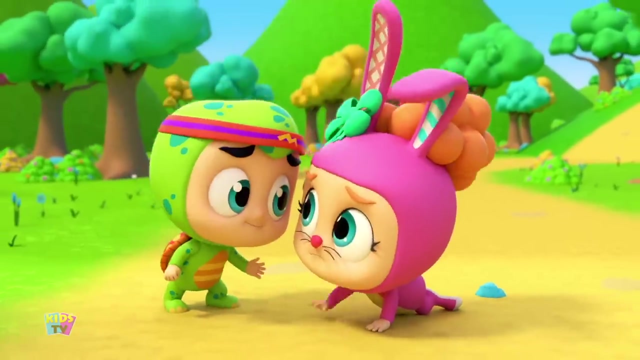 Oh dear. The day of the big big race. The hare began to roar, Run and run. Oh no, oh no. what have I done? Hooray? Slow old tortoise won The day of the big big race. The lesson here is plain to see. 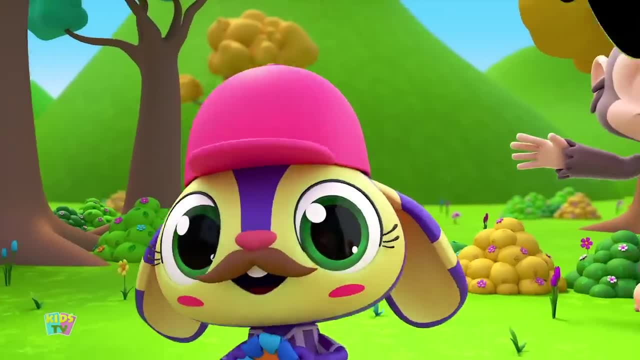 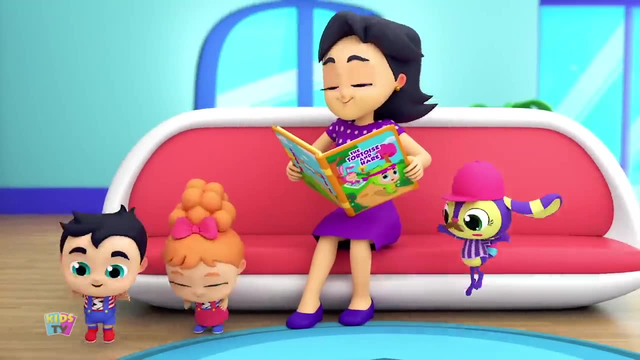 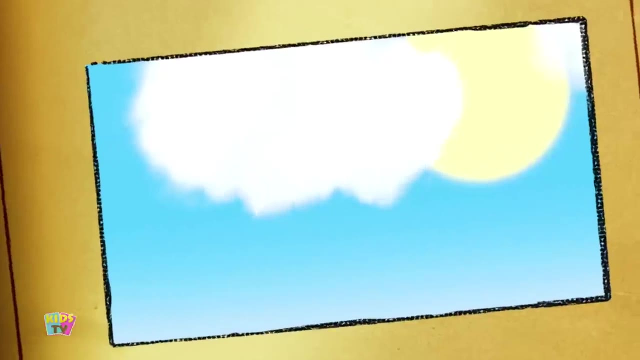 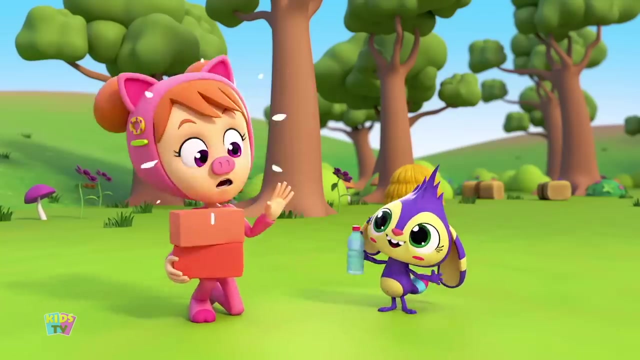 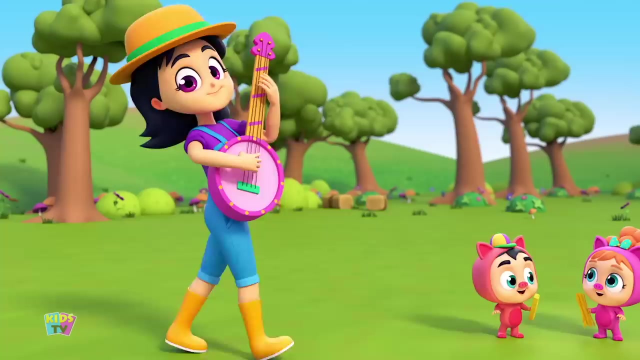 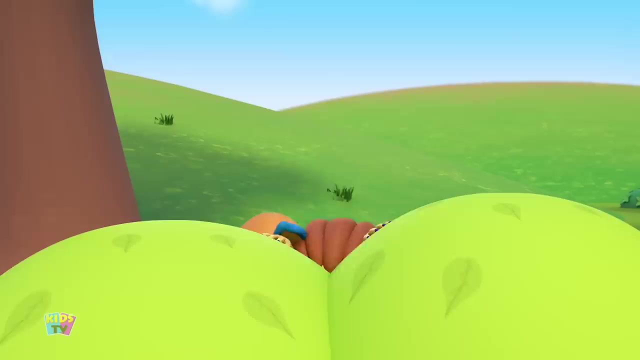 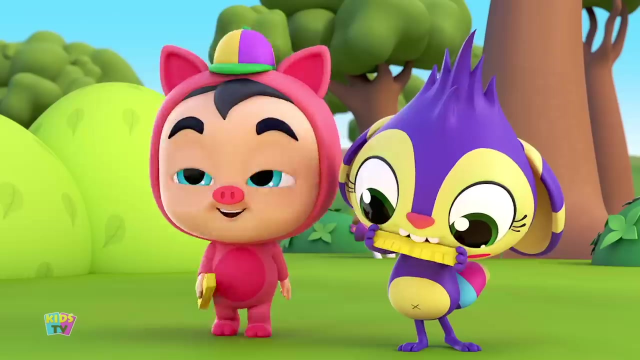 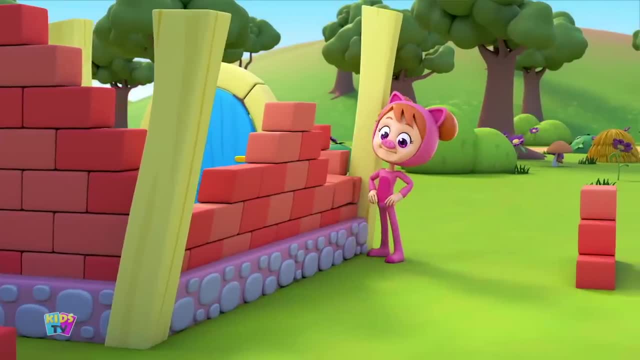 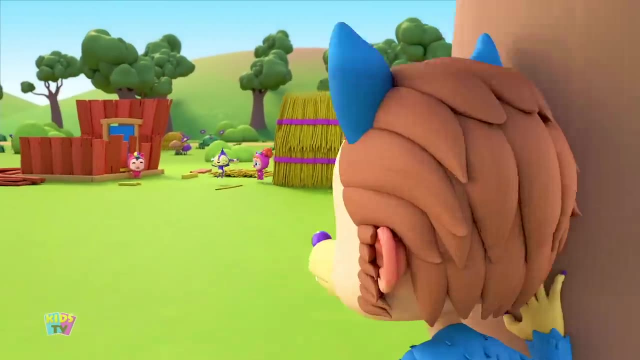 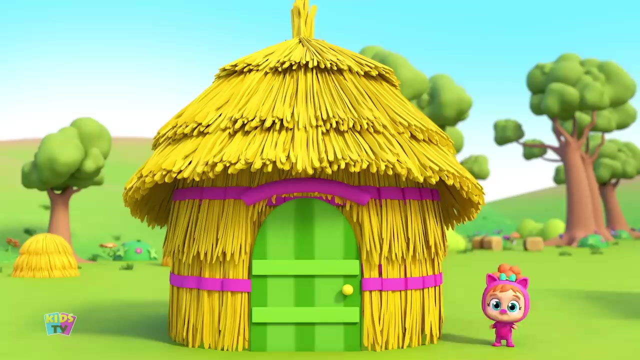 The day of the big big race, The three little pigs had three little homes. All in a row, all in a row. The three little pigs had three little homes. Once upon a time, My house is made of straw, My house is made of sticks And my house is made out of bricks. 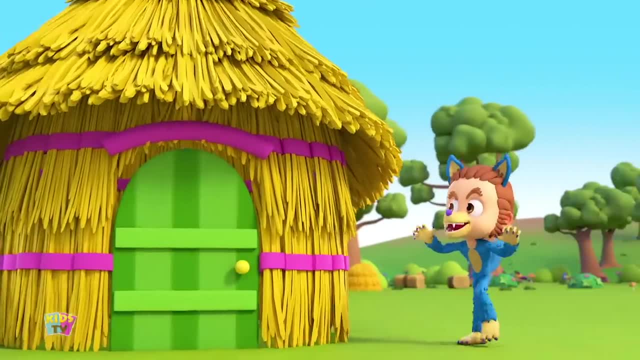 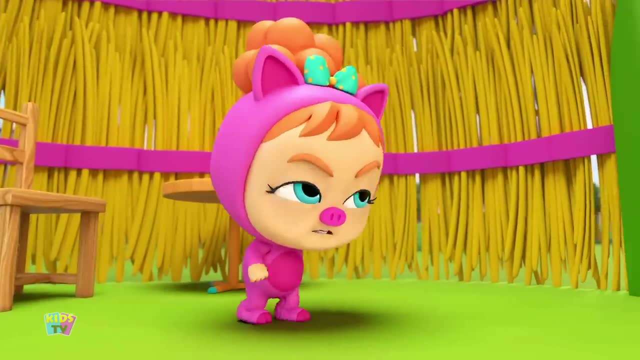 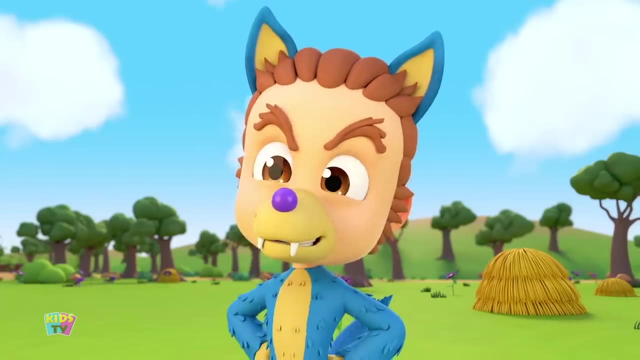 Little pig. now, let me in, let me in. let me in, Not by the hair of my chinny-chin-chin. no, no, no, no, no. Oh yeah, Now I'm going to huff and puff, huff and puff, huff and puff. 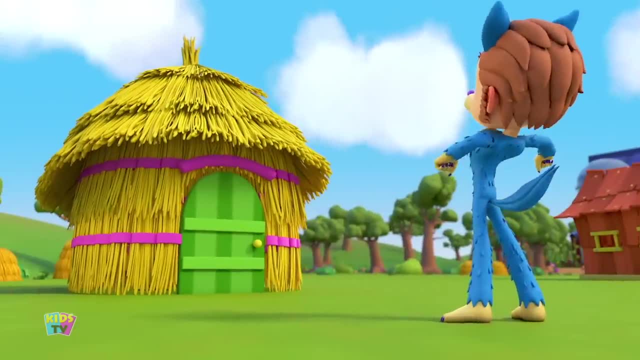 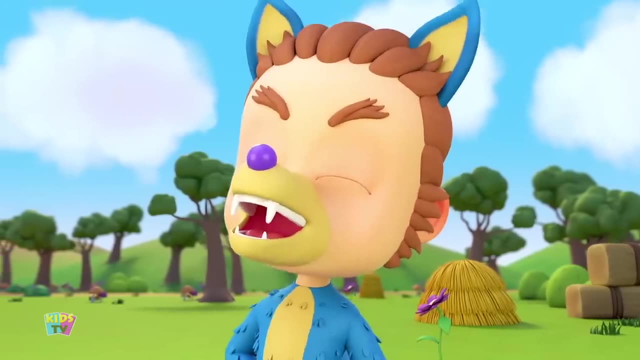 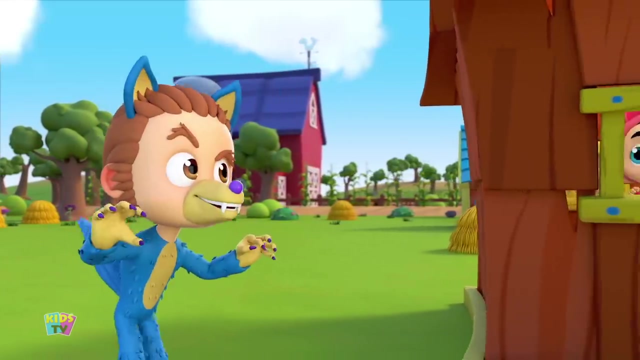 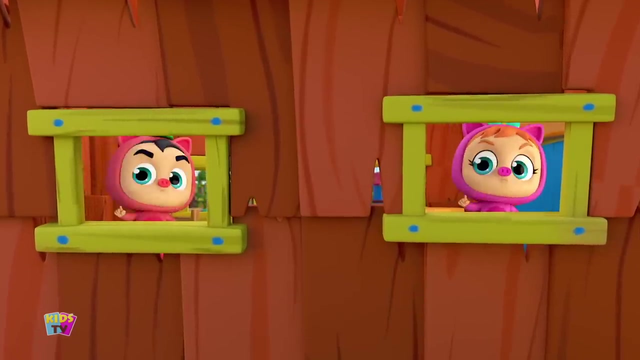 Now I'm going to huff and puff and blow your little house down. Oh no Said the wolf Little pigs. now let me in, let me in, let me in, Not by the hair of my chinny-chin-chin. no, no, no, no, no. 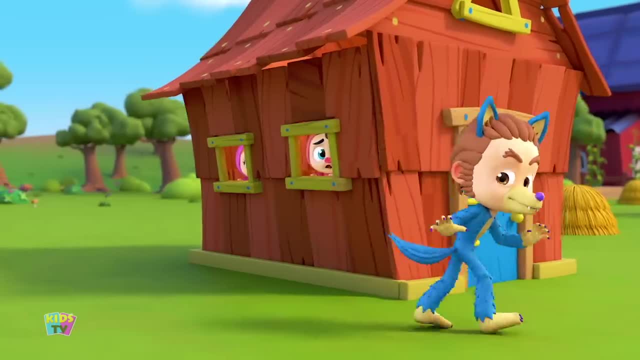 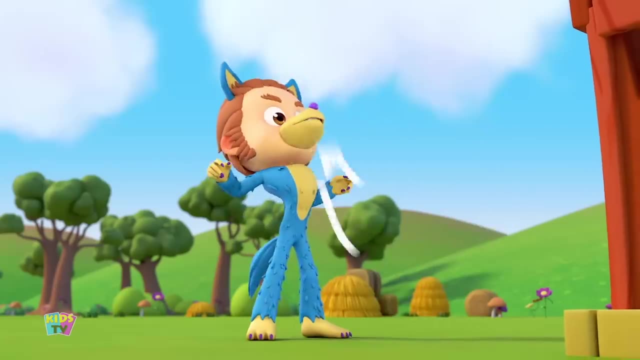 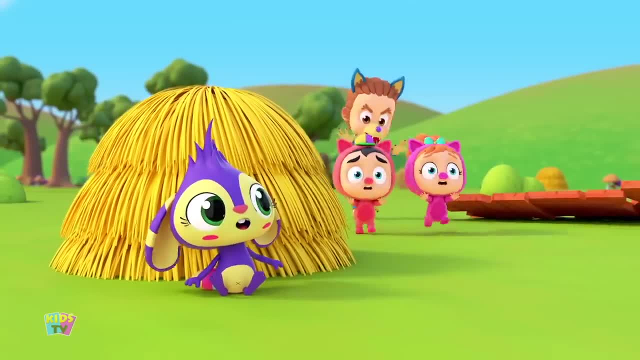 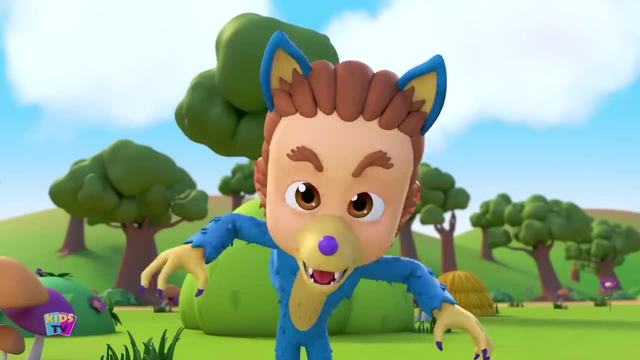 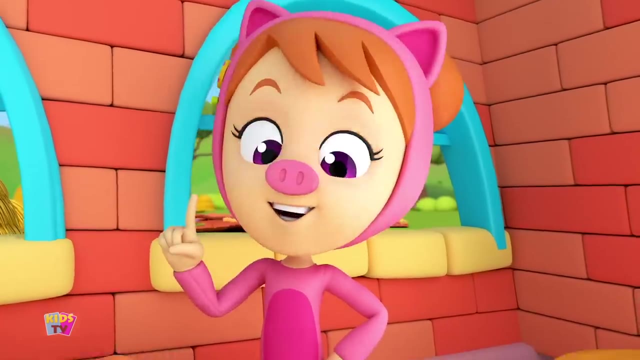 Oh, no Run, Said the wolf Little pigs. now, let me in, let me in, let me in, Not by the hair of my chinny-chin-chin. no, no, no, no, no, no, Oh, no Run. 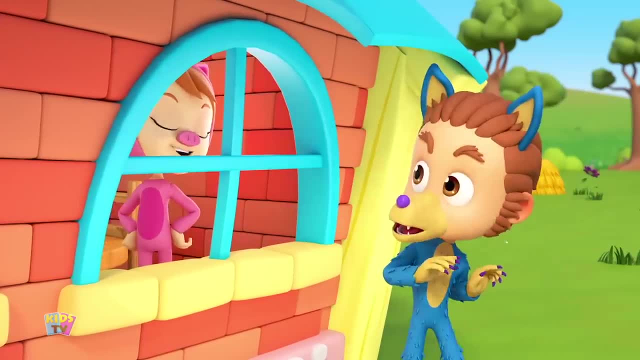 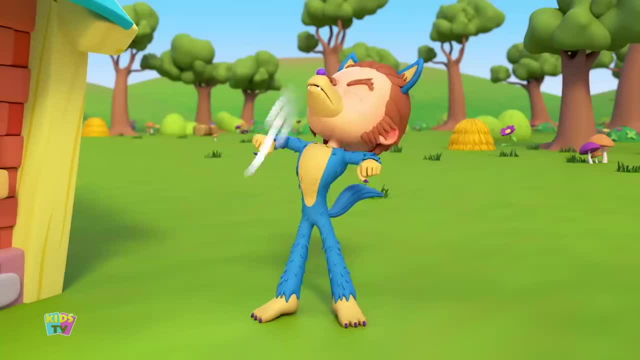 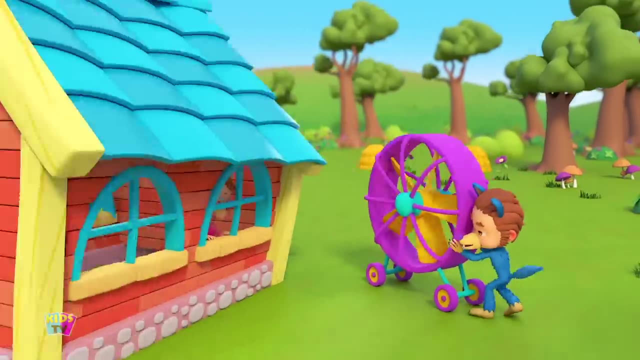 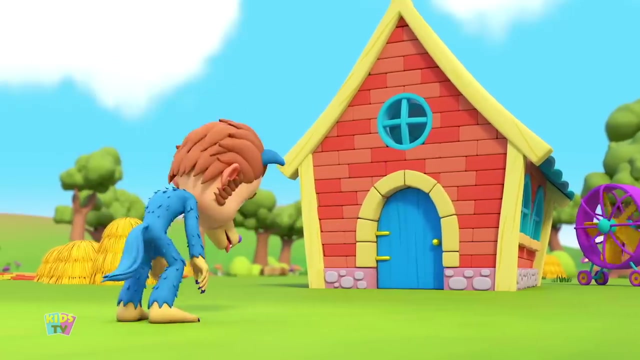 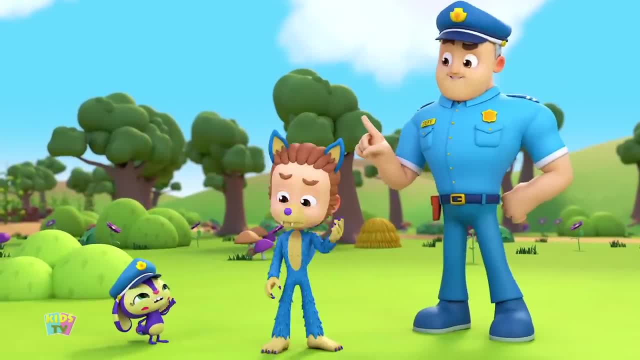 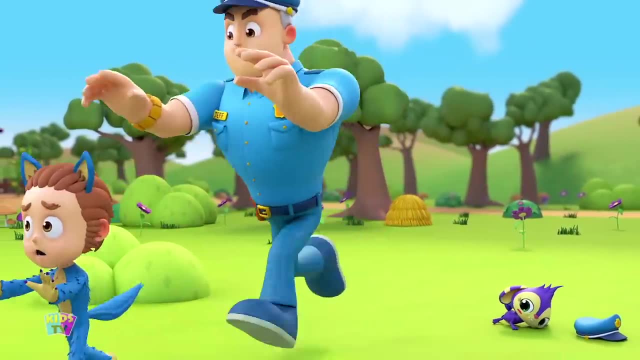 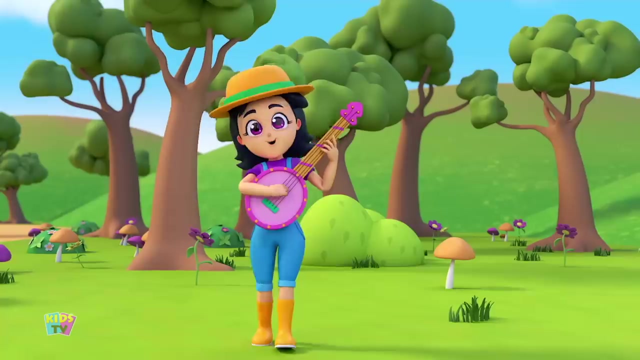 You can't do that, Can't do that, Can't do that, Said the police man. You can't do that. No, no, no, no, no. And that was the story of the Three Little Pigs. The Three Little Pigs. 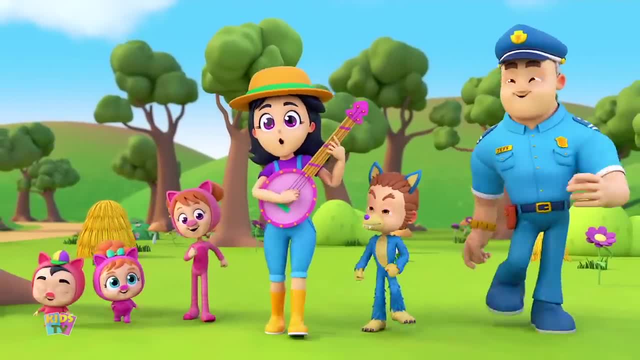 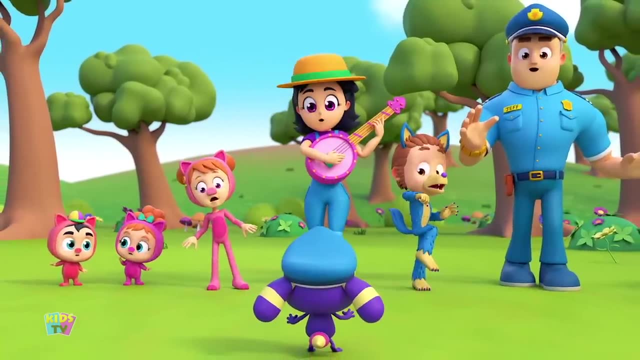 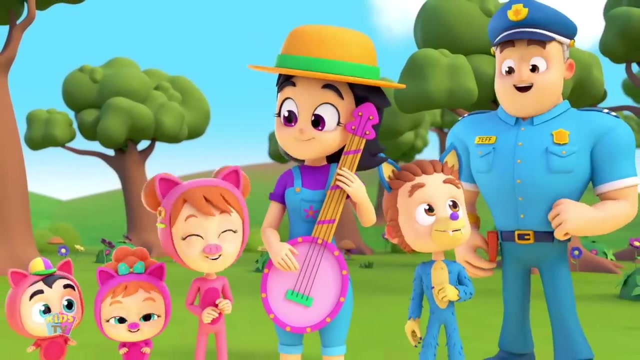 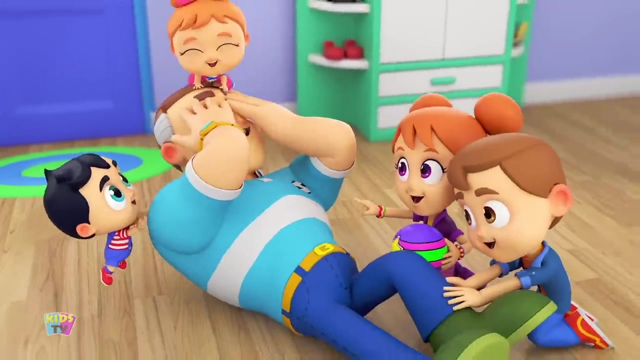 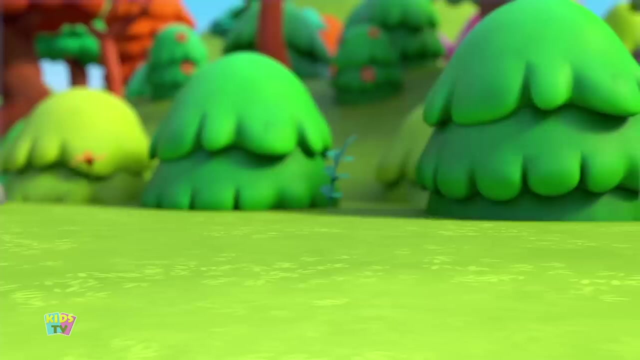 The Three Little Pigs. And that was the story of the Three Little Pigs Once upon a time. Once upon a time, Once upon a time. The Lion and the Mouse, The Lion and the Mouse. This is the story of The Lion and the Mouse. Mouse was creeping through the woods. 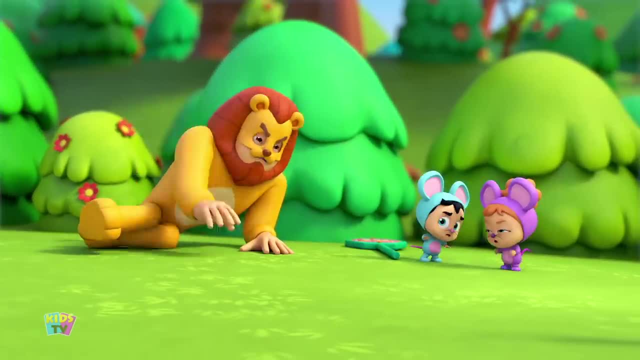 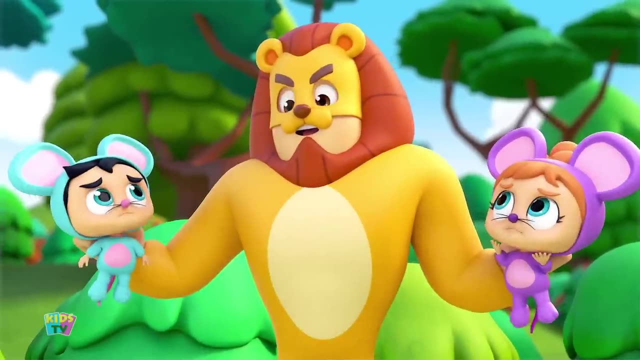 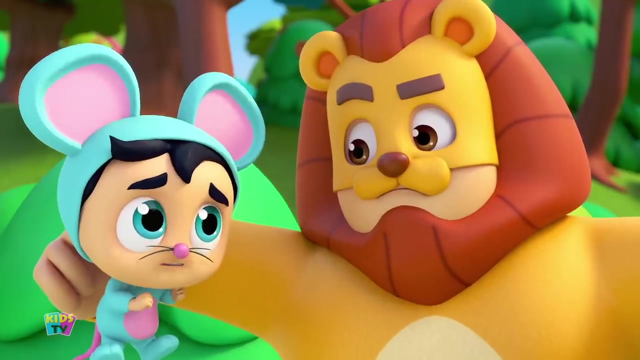 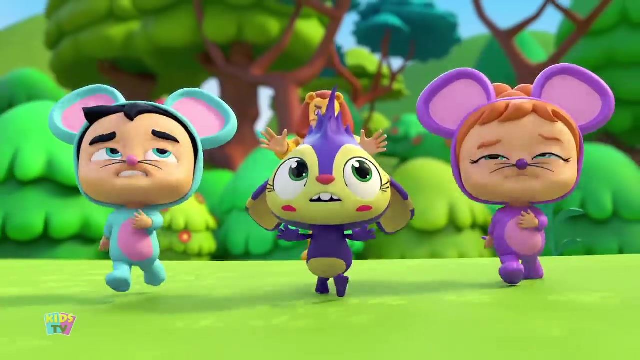 And woke a sleeping lion. Angrily he grabbed that mouse. She was scared and crying. She said: If you let me go, I'll help you someday soon. you'll see, When you need me, I'll be there. You'll count on me. The Lion and the Mouse. The Lion and the Mouse. 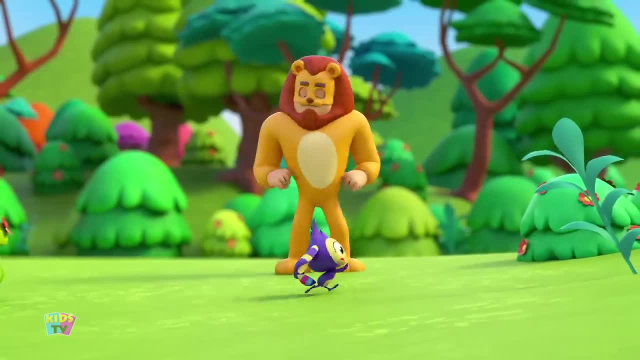 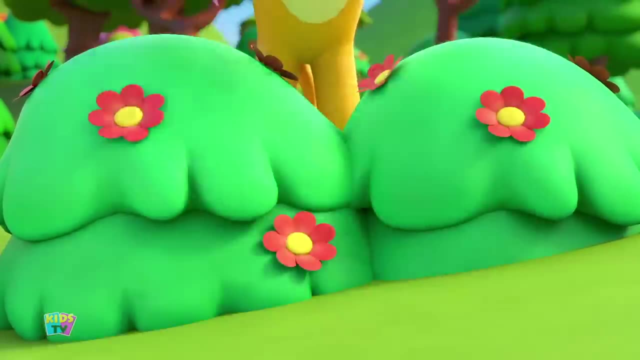 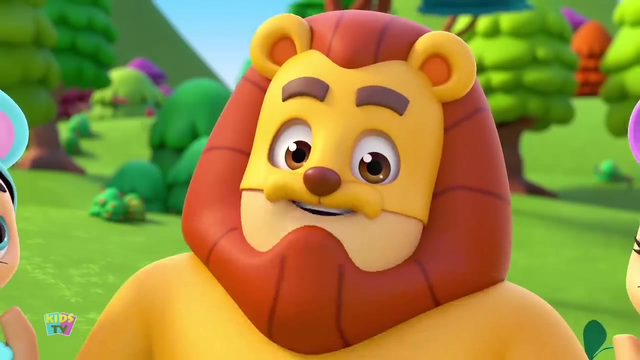 This is the story of The Lion and the Mouse. Lion and the Mouse, The Lion and the Mouse. This is the story of The Lion and the Mouse. Lion said: You tiny thing, what can you do for me? Tell you what. you made me laugh. 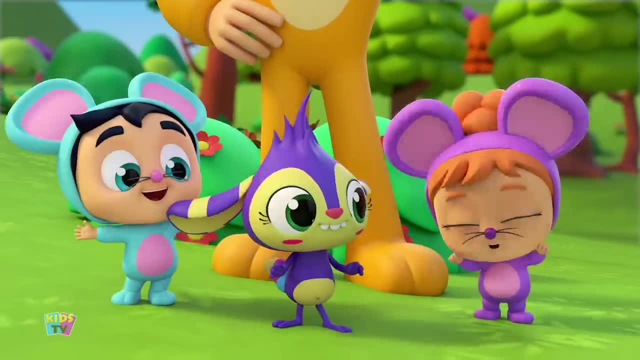 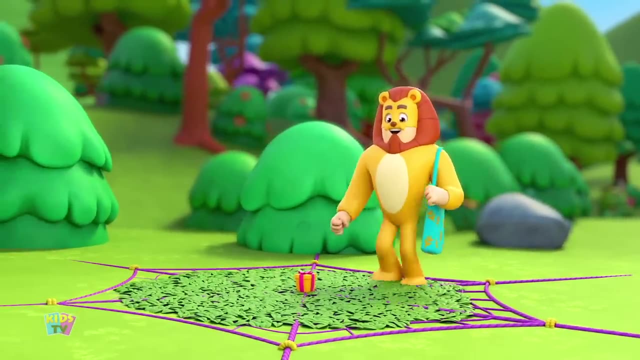 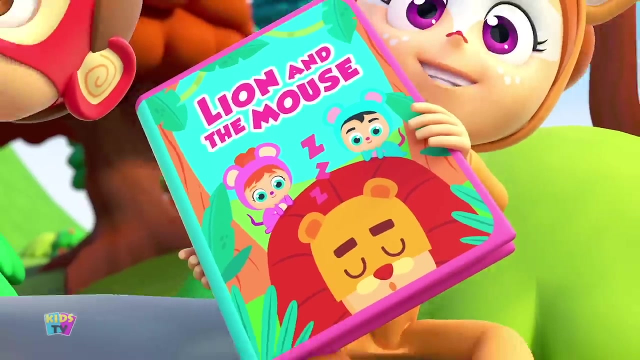 So I will set you free. Thank you. Next day, Lion stalked his prey, But on his way back home He walked into a trap. He was captured and alone. The Lion and the Mouse. The Lion and the Mouse. This is the story of The Lion and the Mouse. 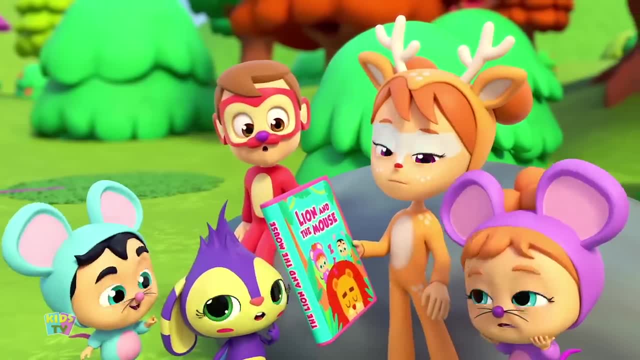 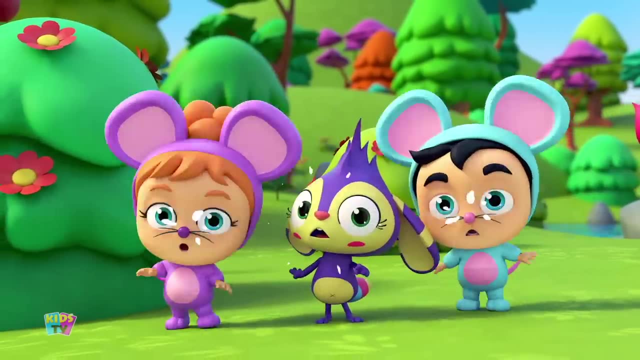 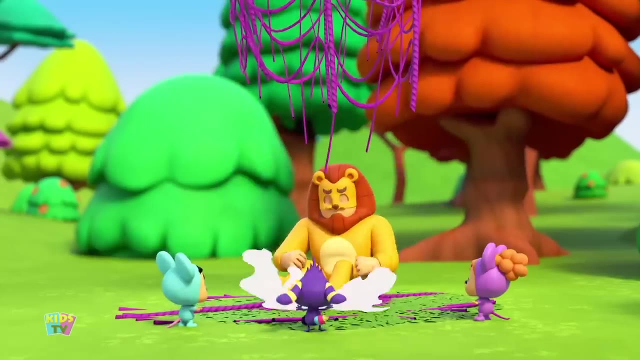 Lion and the Mouse. The Lion and the Mouse. This is the story of The Lion and the Mouse. Tiny Mouse heard Lion's roar. He scurried to the scene. She gnawed the rope, Released the lion and said: Now we're a team. Lion answered: 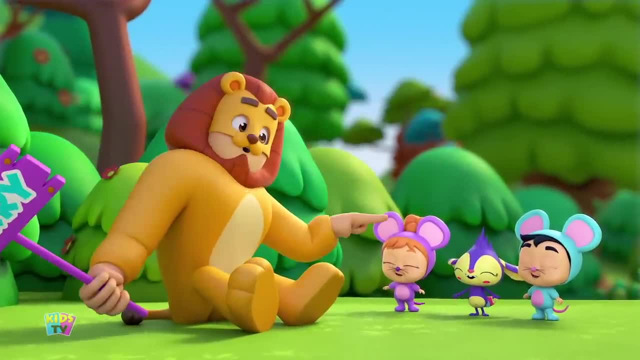 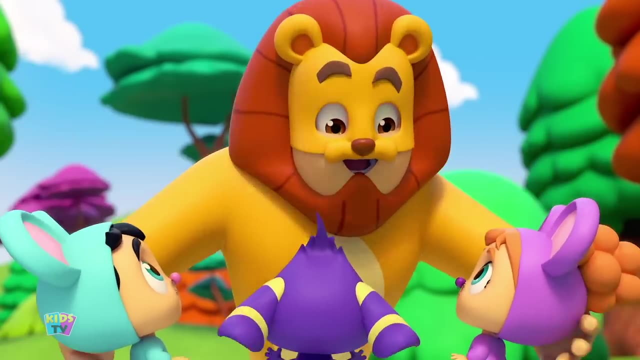 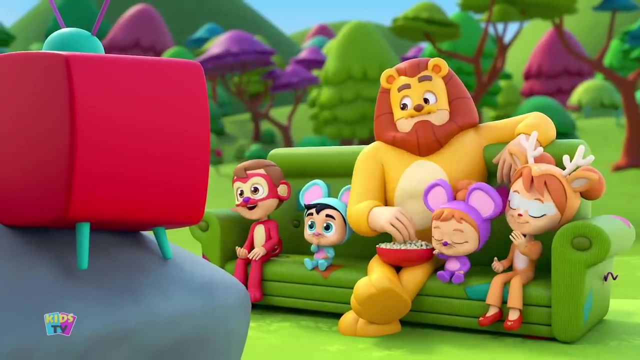 I was wrong to laugh because you're small. If it weren't for you, I would not be here at all. The Lion and the Mouse. The Lion and the Mouse- Best friends forever. The Lion and the Mouse. The Lion and the Mouse. The Lion and the Mouse. 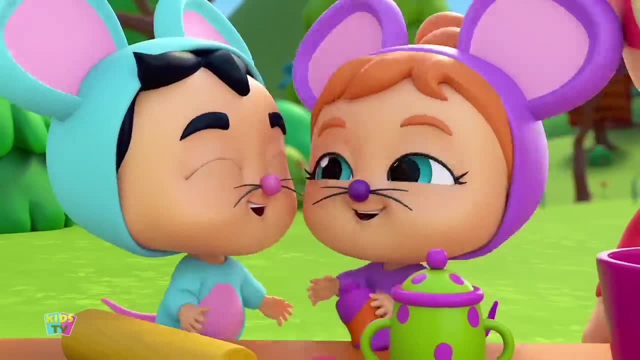 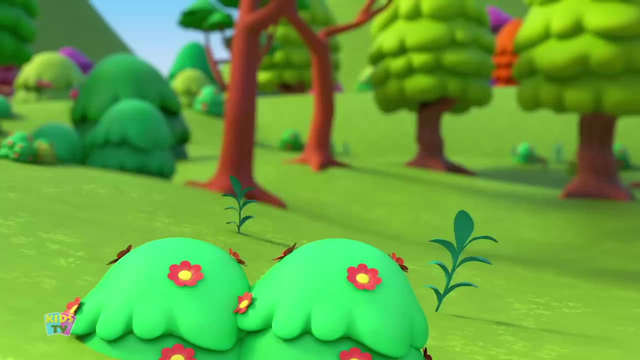 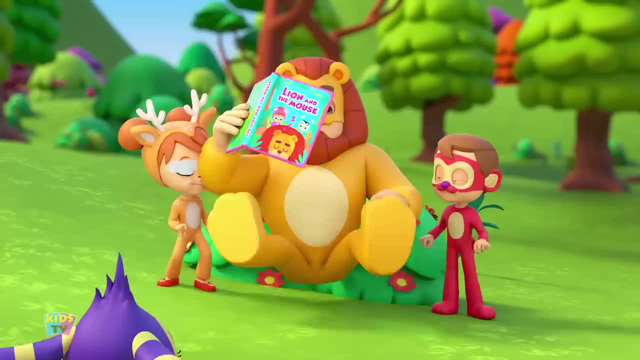 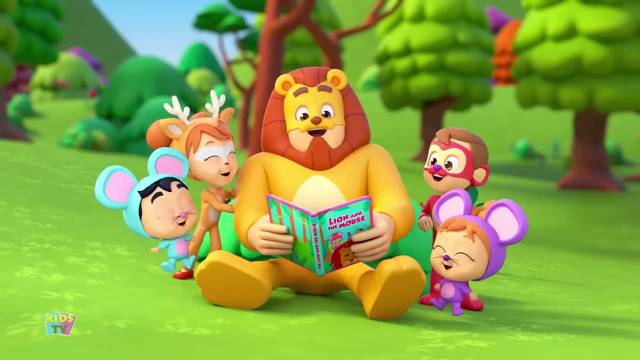 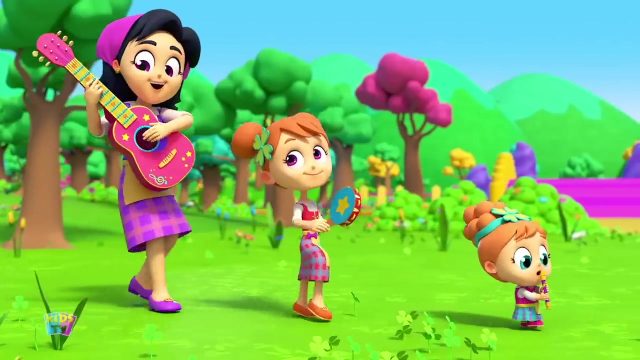 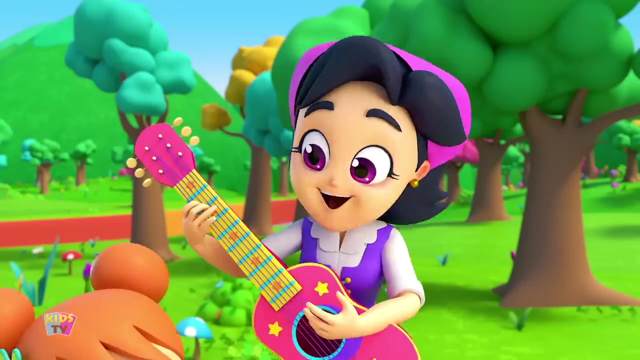 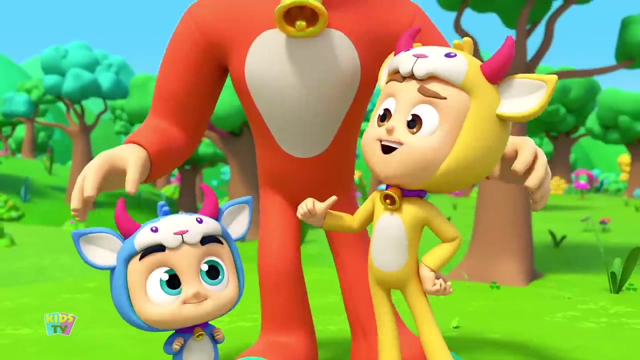 Lion and the Mouse. Lion切った 4k Mission Control Hammer sólo Não Bela Bela. Once upon a time they lived upon a grassy bluff: Billy the Little and Billy the Middle And Billy the Biggie, the Billy Goat Scruff. 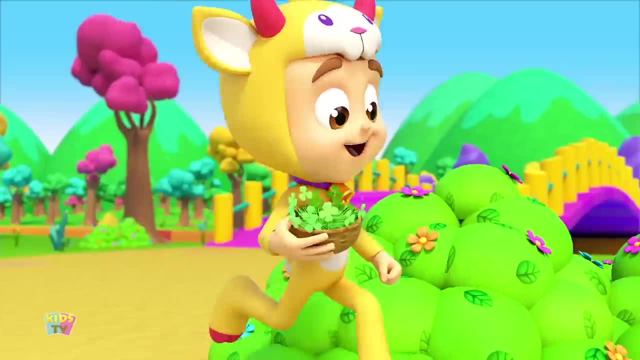 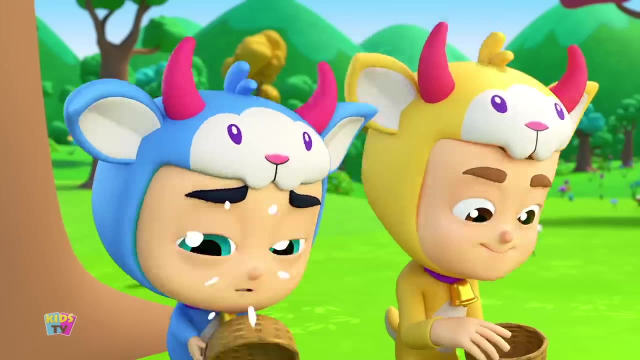 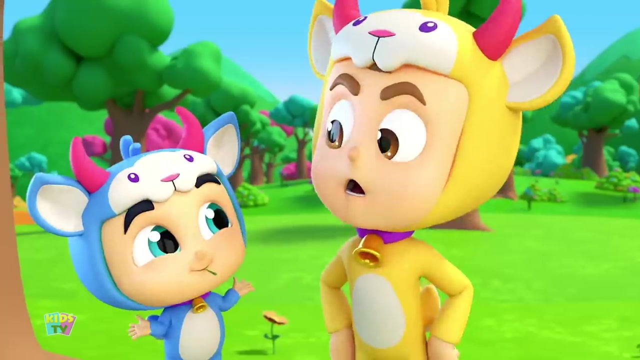 Billy the Biggie, the Billy Goat Scruff. They ate and ate the grass all day until it all was gone. They ate all the clover till none was left over. They were lawnmowers, those Billy Goat Scruff. They were lawnmowers, those Billy Goat Scruff. 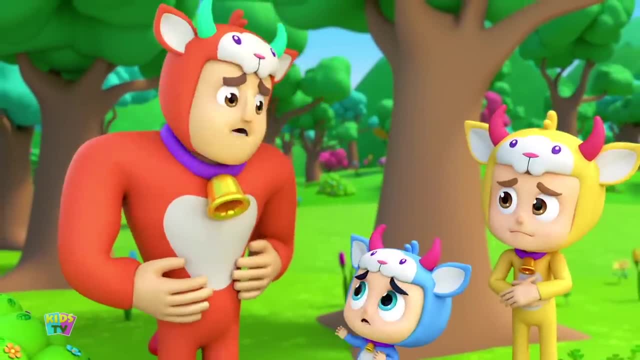 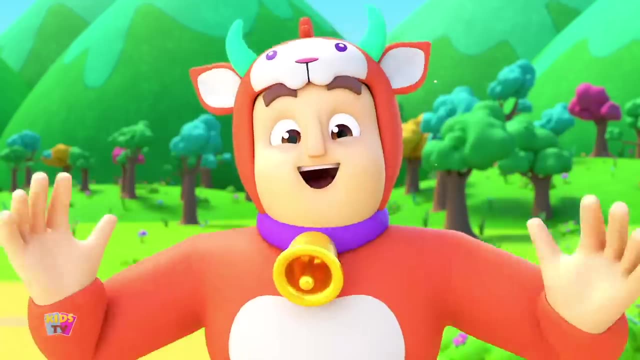 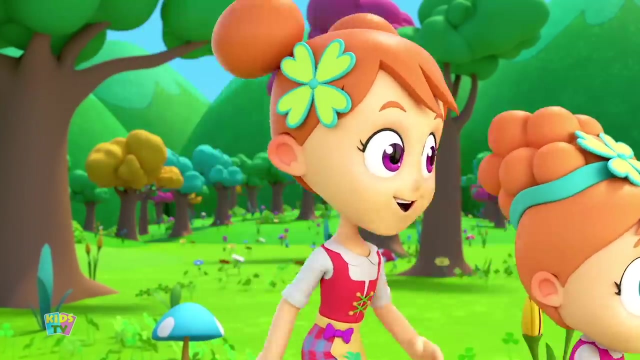 But over a river and over a bridge was a hillside covered with grass, Green and delicious and rich and nutritious. It answered their wishes, that yummy, fresh grass. It answered their wishes that yummy, fresh grass. Billy the Little ran down to the river and onto the bridge he hopped. 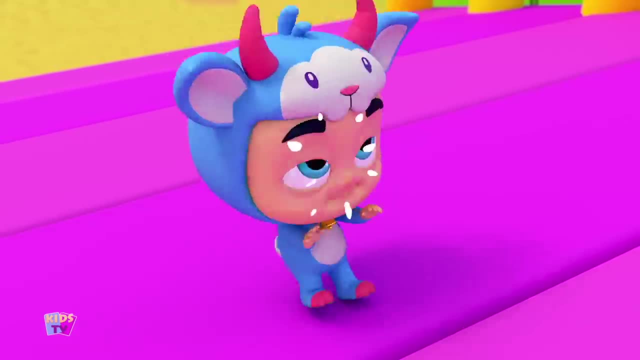 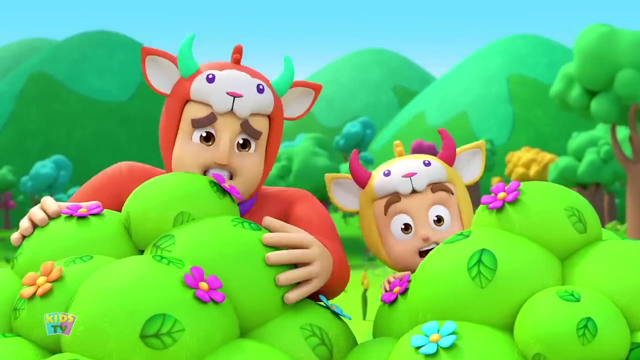 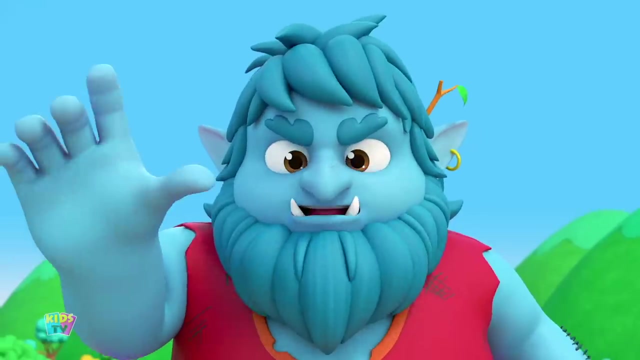 Clippity, cloppity, hippity, hoppity. Up jumped a troll and he hollered out: Stop. Up, jumped the troll and he hollered a stop, Who are you? Said the troll. I'm Billy, the Little Goat. Scruff, Before I get thinner, I'll eat you for dinner. 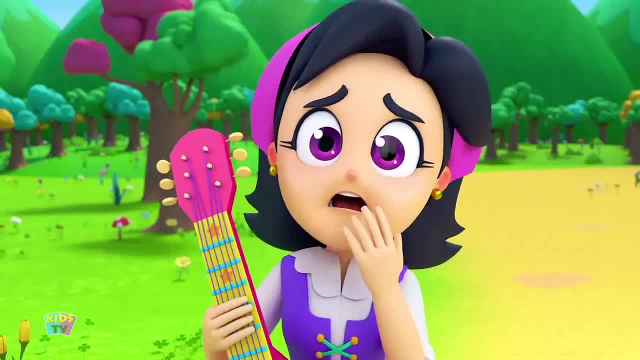 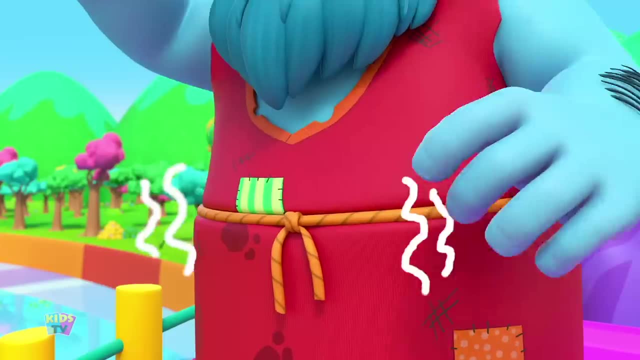 Would this be the end for this Billy Goat Scruff? Would this be the end for this Billy Goat Scruff? Oh please, Mr Troll, I'm very small and you look very hungry, Billy. Billy, the Middle Goat Scruff is coming next and he's much bigger and tastier than I am. 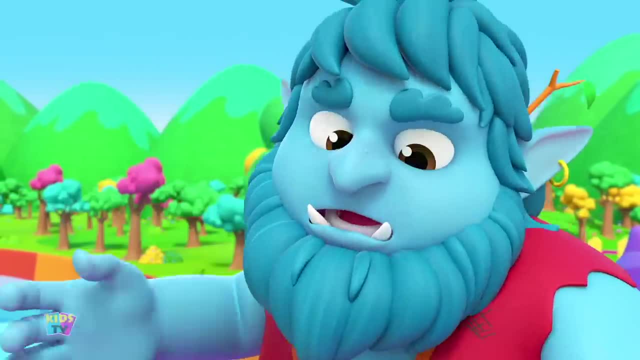 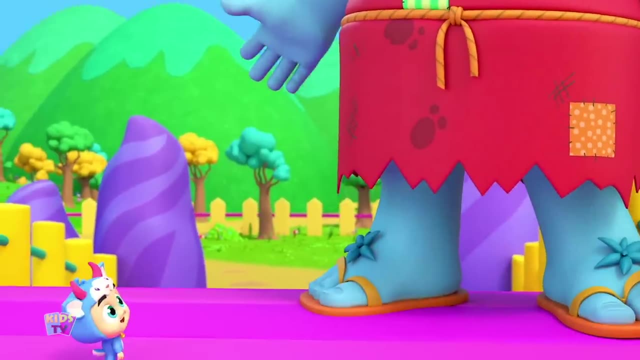 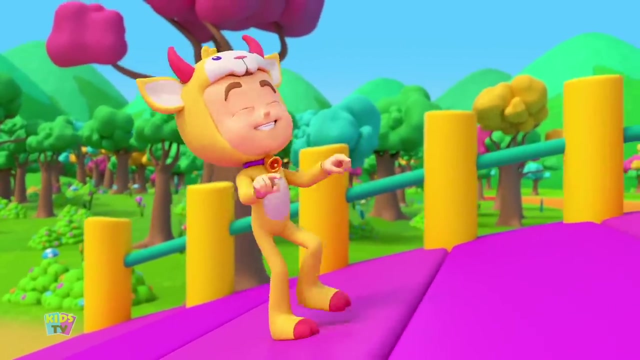 Well, alright, then be off with you. I'll wait for Billy the Middle. Goat Scruff. Billy the Middle ran down to the river and onto the bridge. he hopped, Clippity, cloppity, hippity, hoppity Up, jumped the troll and he hollered out. 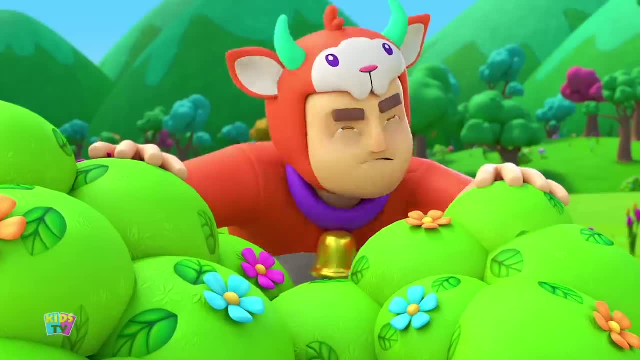 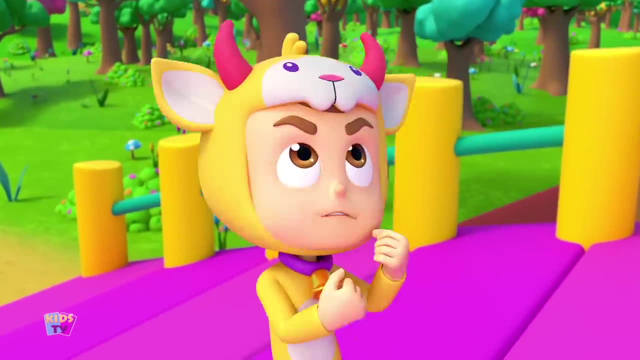 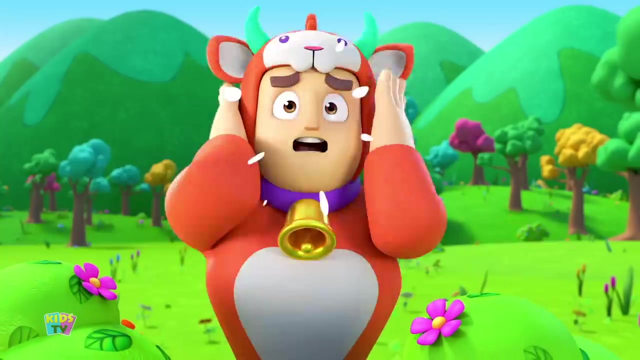 Stop Up, jumped the troll and he hollered a stop. Who are you, Said the troll? I'm Billy the Middle Goat Scruff. Before I get thinner, I'll eat you for dinner. Would this be the end for this Billy Goat Scruff? Would this be the end for this Billy Goat Scruff? 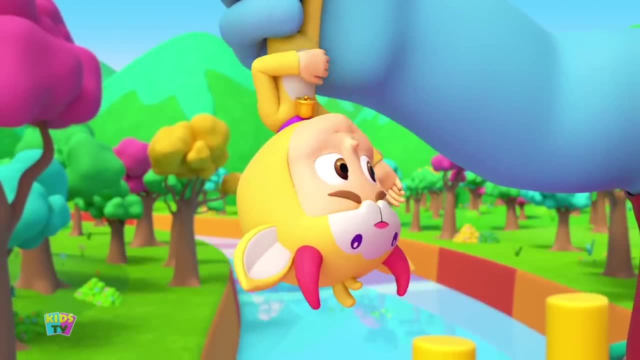 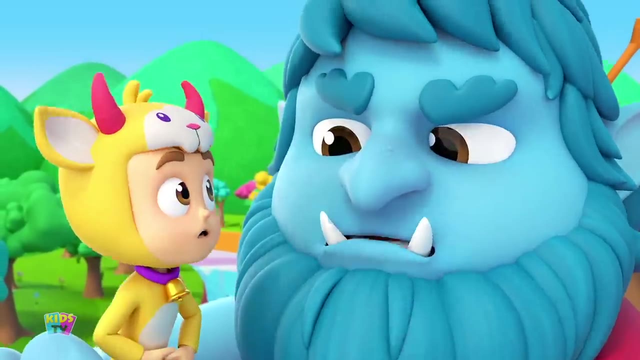 Oh please, Mr Troll, I'm not very big and you look very hungry. Billy the Biggie Goat Scruff is coming next and he's much bigger and tastier than I am. Well, alright, then be off with you. I'll wait for Billy the Biggie Goat Scruff. 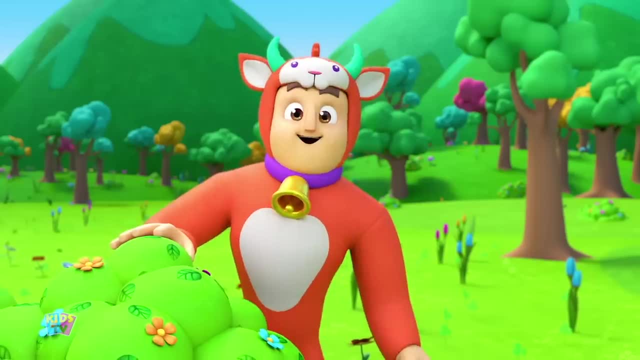 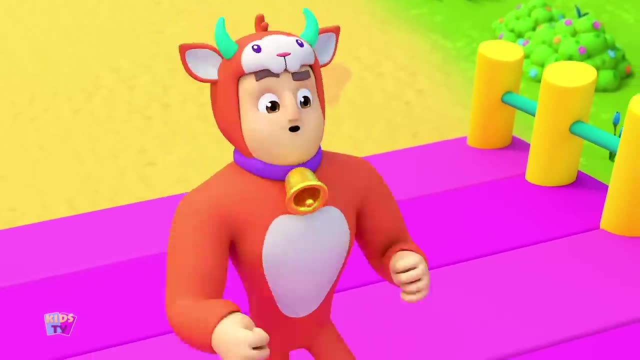 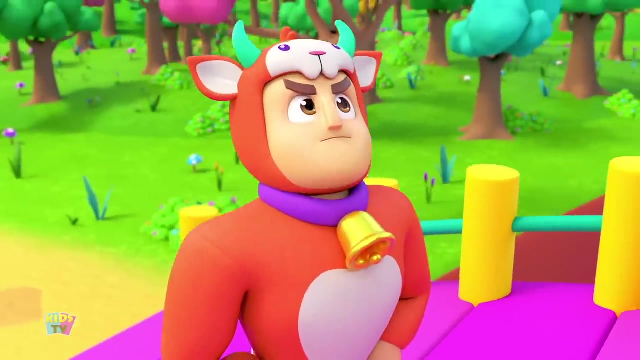 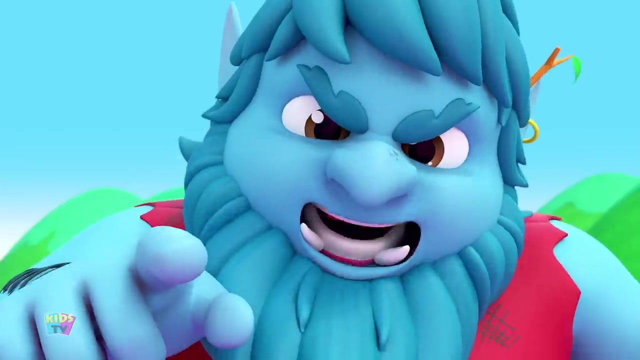 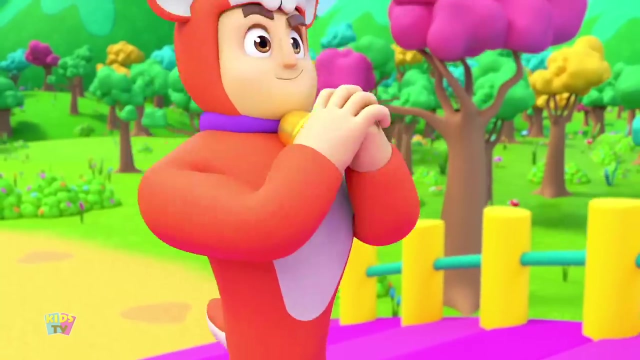 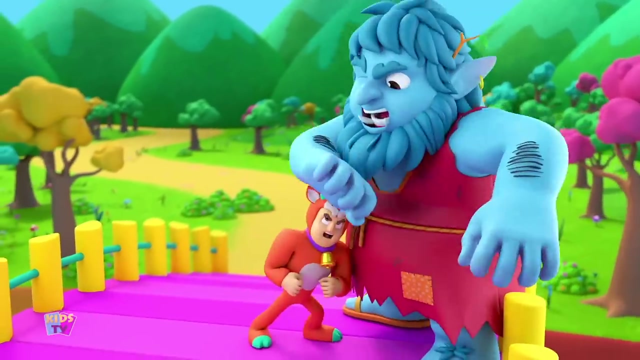 I would to you, Billy the Middle Goat Scruff. The Troll's raw wit was in sí, Billy the Middle Goat Scruff. Hey guys, And for this Billy go gruff. Oh yeah, Billy the Biggie. He lowered his horns And charged straight at the troll, And over and over. 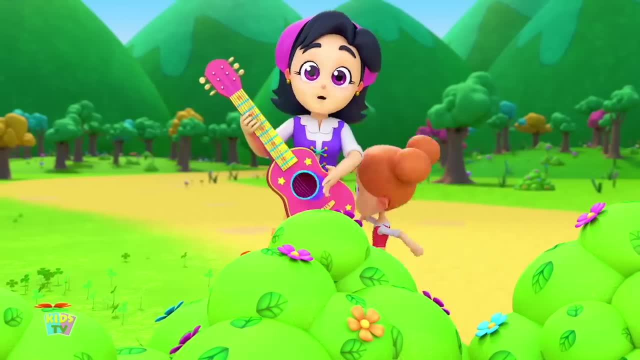 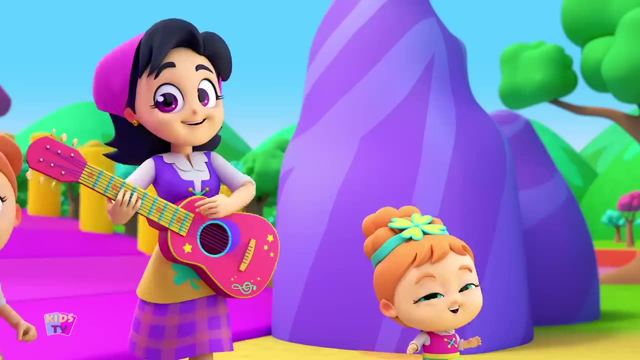 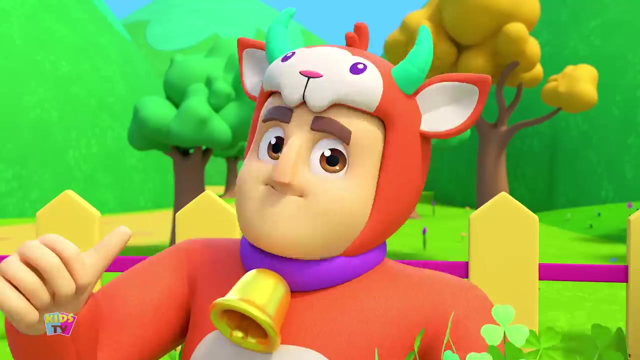 Hill, over glen And over the mountain, That bad troll flew. Over the mountain, That bad troll flew, And happily ever after He lived upon that grassy block. Billy the Little And Billy the Middle And Billy the Biggie. The Billy Goats Gruff And Billy the Biggie. 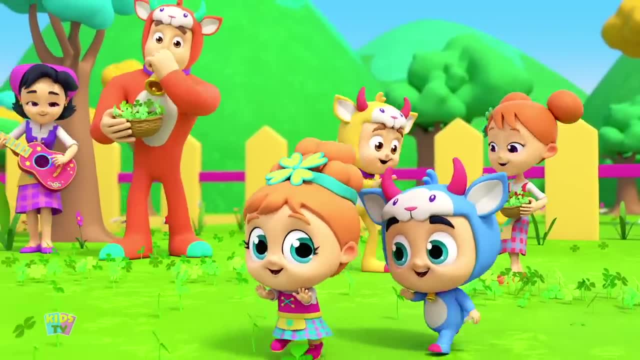 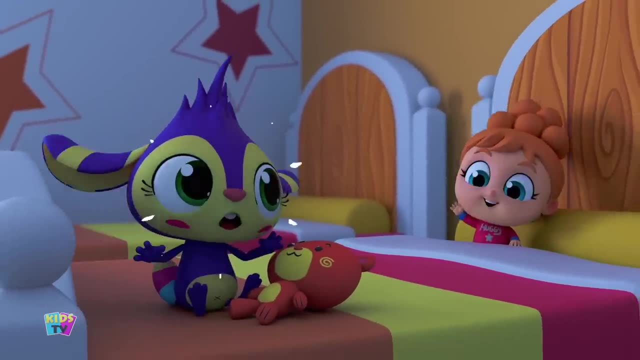 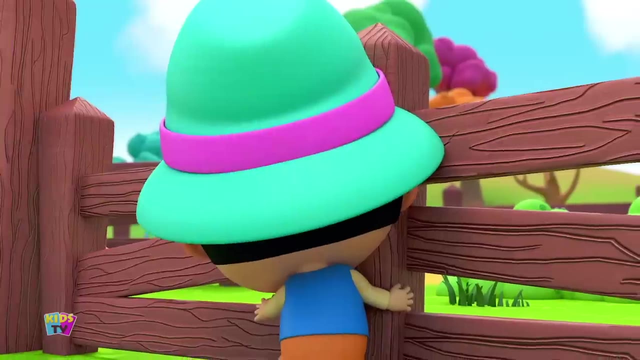 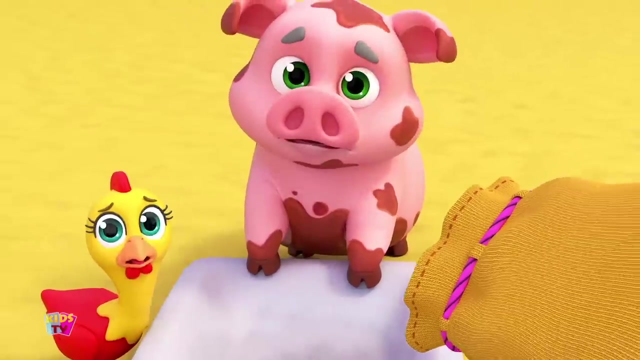 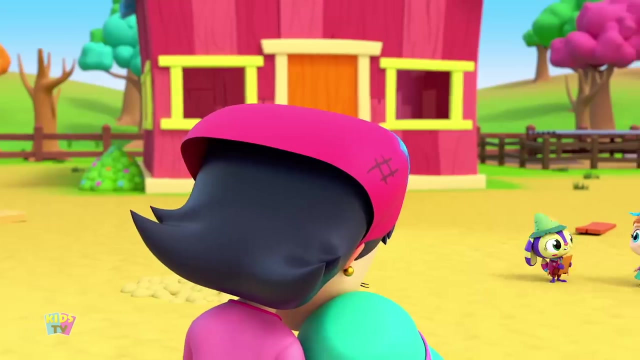 The Billy Goats Gruff. There was a little boy And his name was Jack. He lived with his mama In a little old shack. Jack asked: mama, Why are we poor? A giant came And smashed our door. He stole everything we had. We had. He stole everything we had. 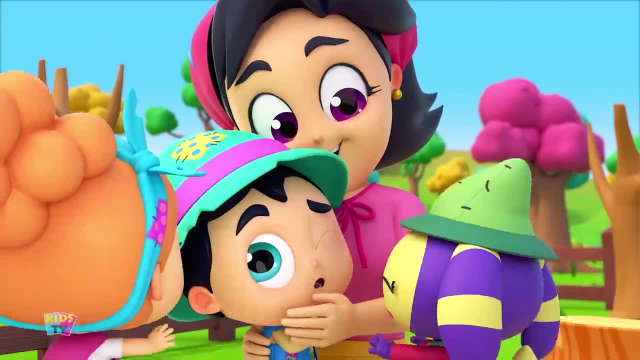 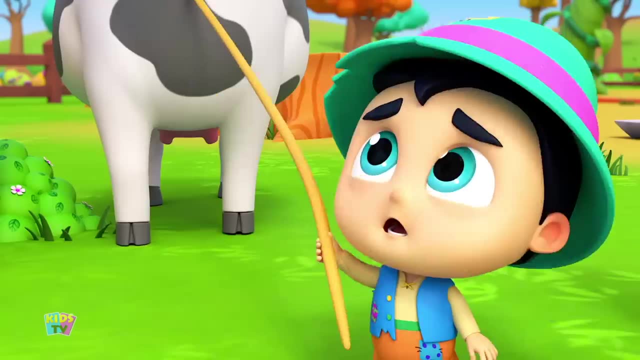 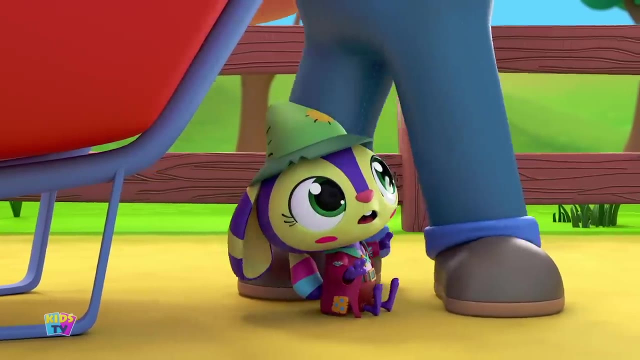 Jack, we have to sell our cow Off to the market. You better go now. So Jack took the cow And he walked down the road Where he met a man Pulling a heavy load. That's a mighty fine cow, He said. he said That's a mighty fine cow. 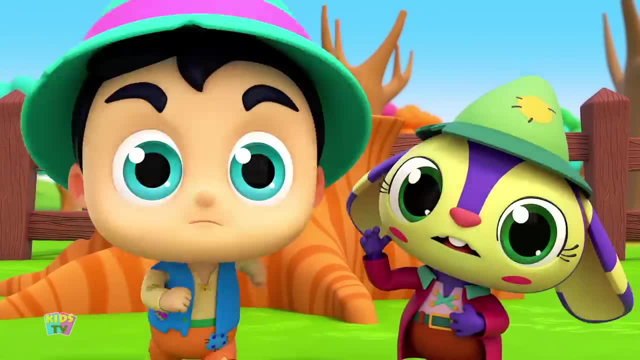 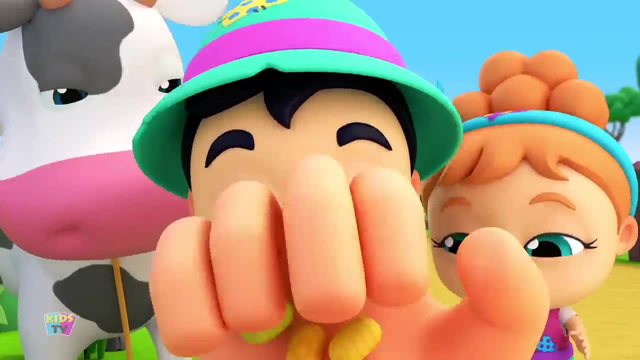 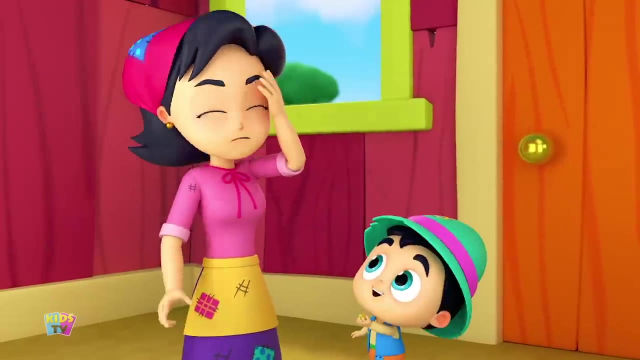 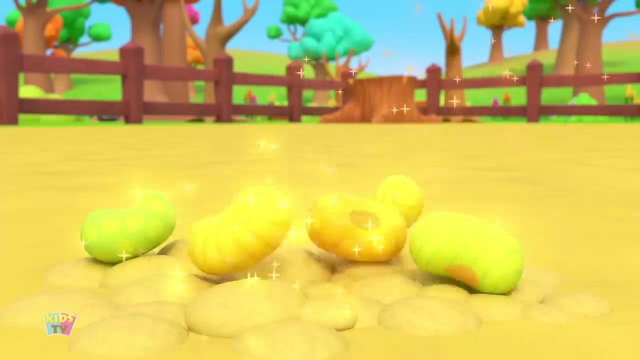 He said: I'll buy your cow For magic beans, The prettiest beans You've ever seen. That's a deal. And Jack ran home. When mama saw the beans, She moaned and groaned: Out the window, They flew. They flew Out the window, They flew The minute the beans. 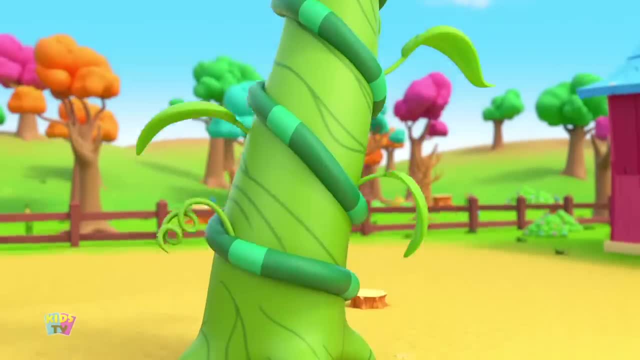 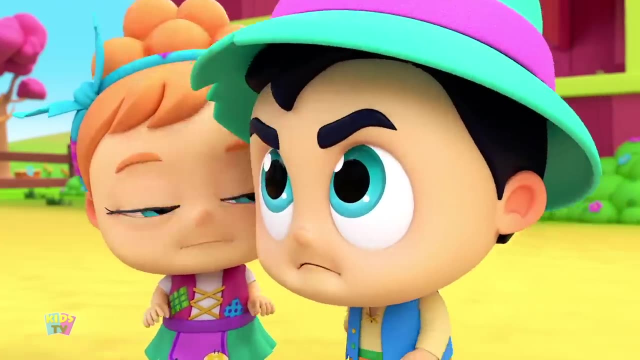 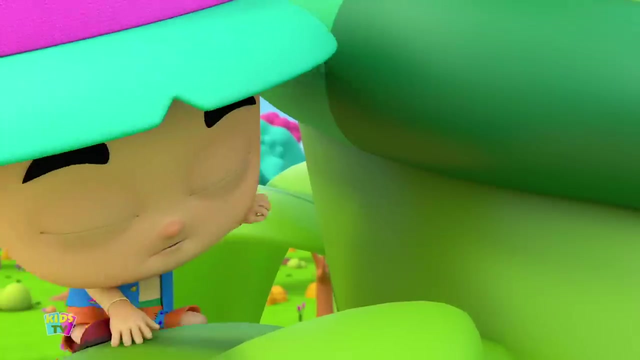 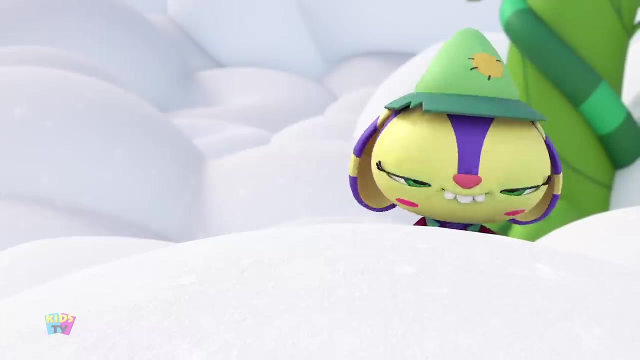 Landed on the ground. They started to make A rumbling sound Out from the ground. The beans stalked through Right up to the clouds And then right through Up that stalk. Jack climbed, Jack climbed Up that stalk. Jack climbed Through the clouds And through the sky. Jack was very, very high. 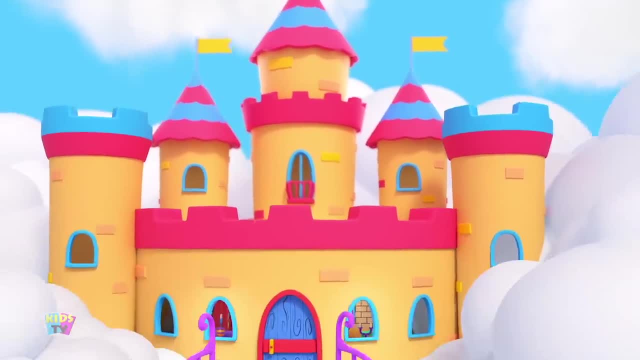 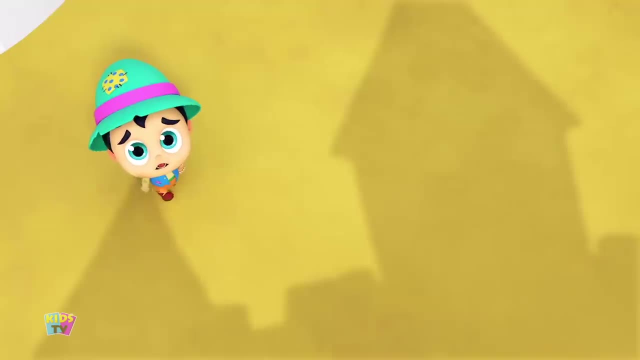 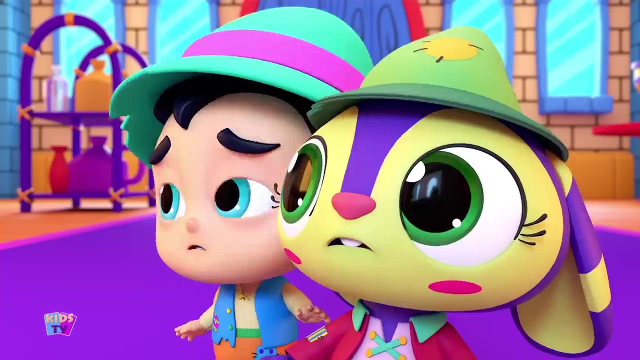 He came to a door In a dark, dark cloud With a sign that read: No kids allowed. Jack was very, very high. Jack just walked Straight through, Straight through. Jack just walked Straight through Into a castle. The dark door led And down the hallway. Young Jack sped A huge room he found. 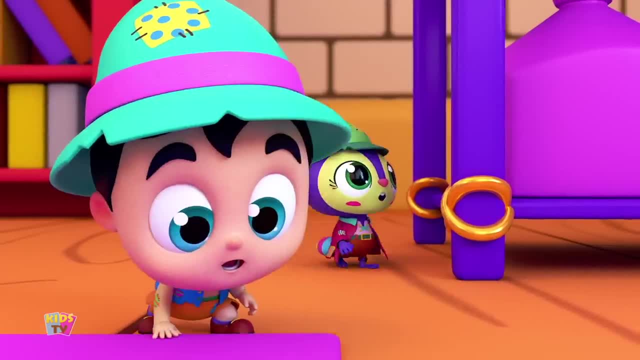 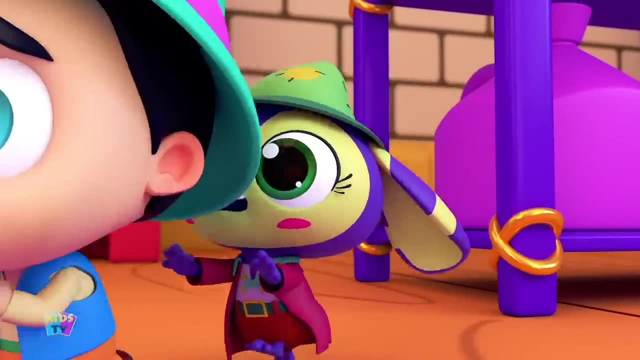 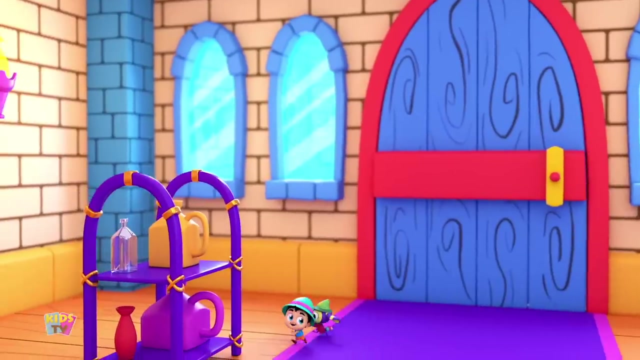 Then he heard A scary sound: A giant steps, Boom, boom, boom. A giant steps, Boom, boom, boom, boom, Fee-fi-fo-fum. I smell a boy By gosh my thumb, That bad giant. He boomed and boomed And Jack went flying Out of that room. 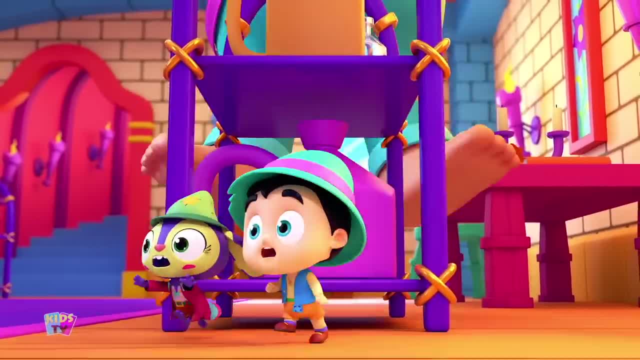 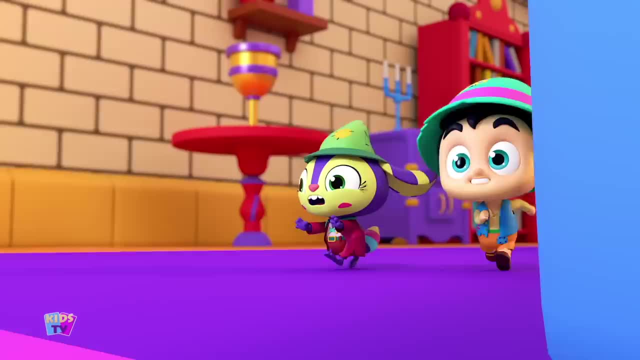 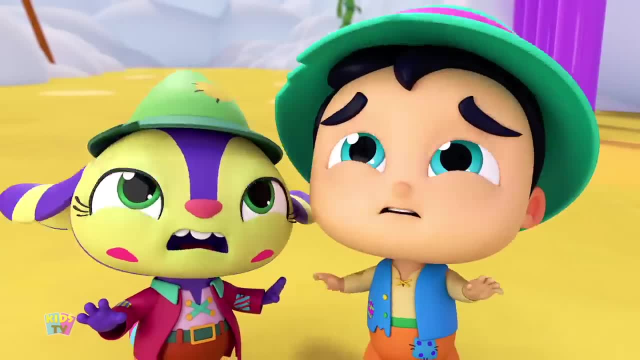 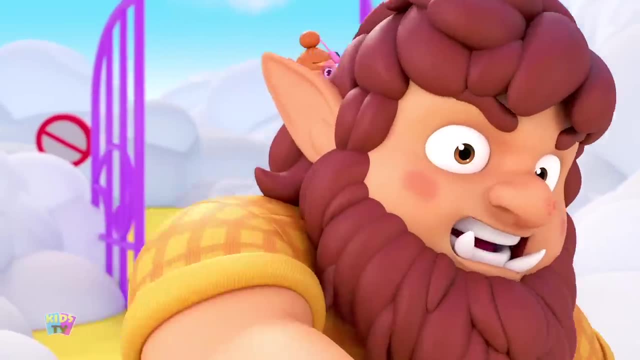 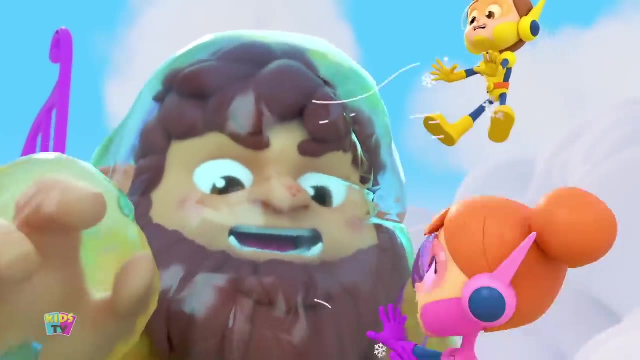 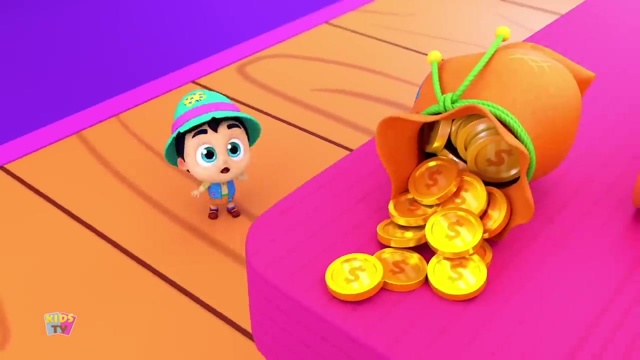 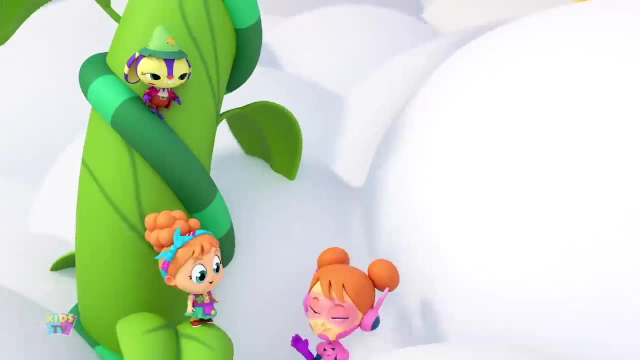 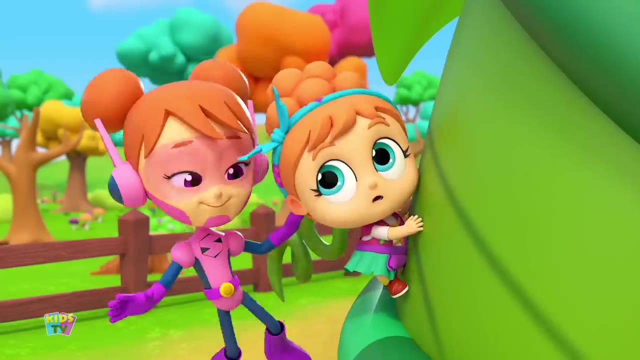 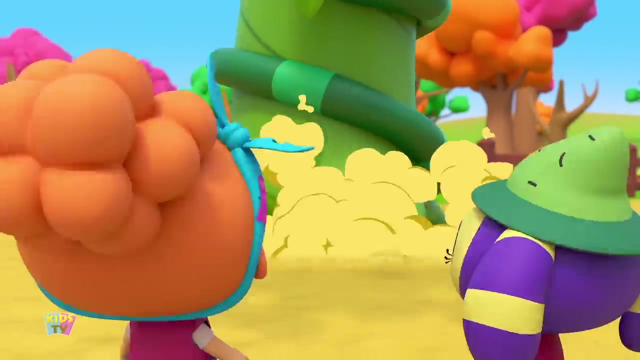 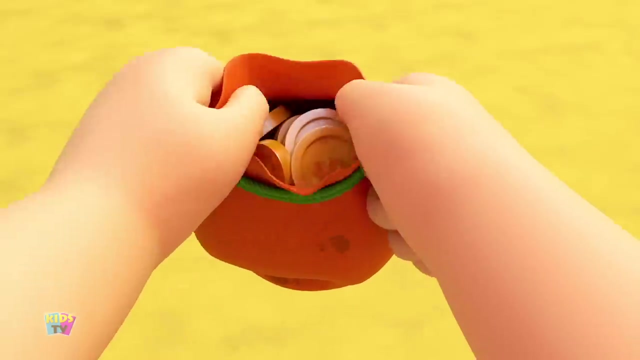 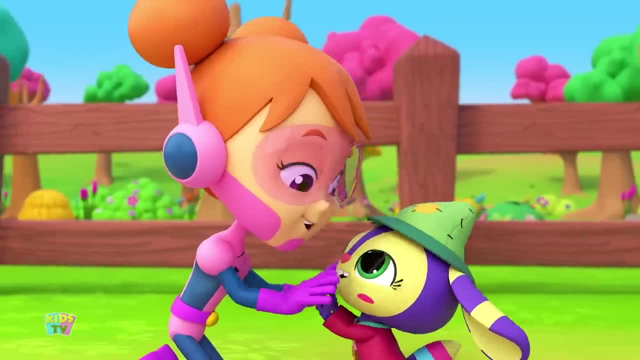 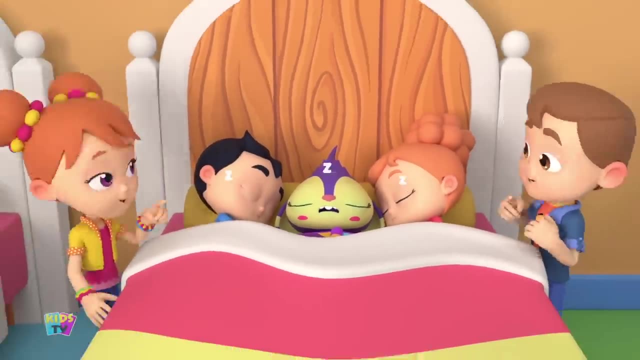 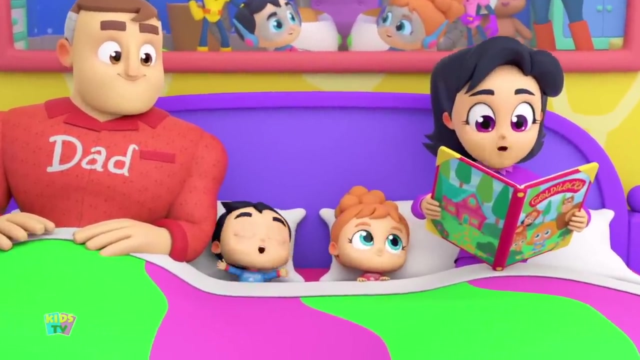 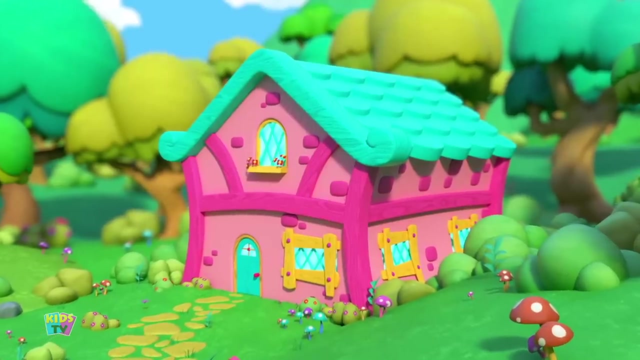 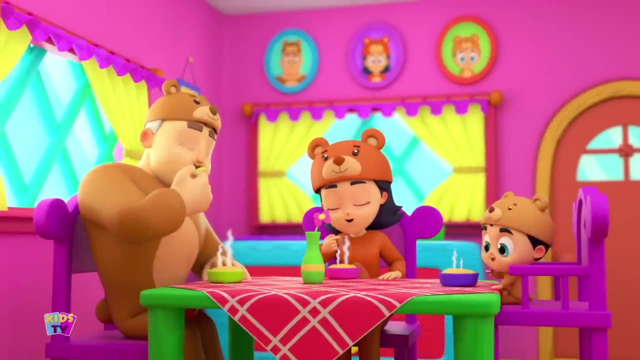 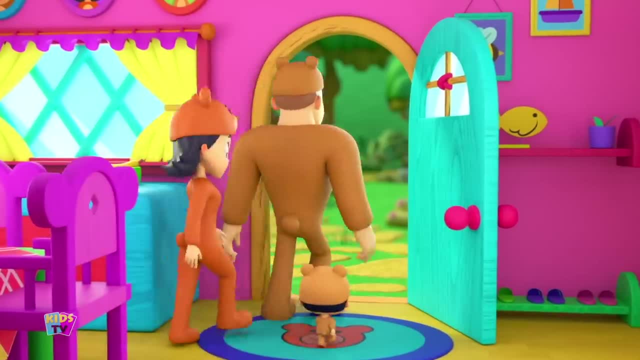 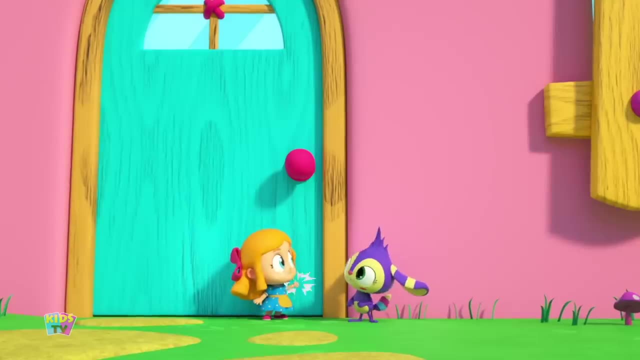 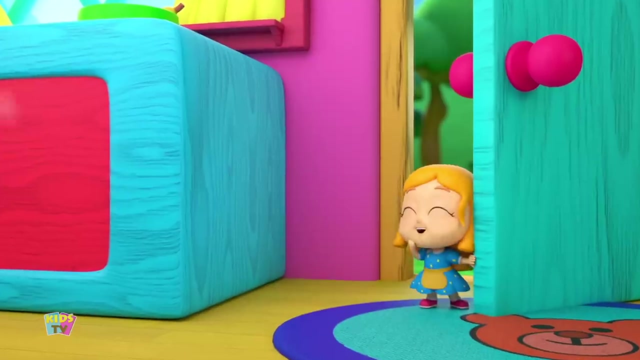 let's go walk in the forest. That's when Goldilocks came by, found their house in the thicket Knock, knock, knock. no answer. so Goldie entered the kitchen. Mmm smells good. She grabbed a spoon. 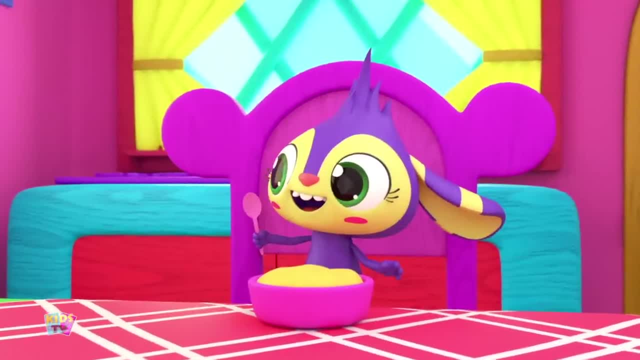 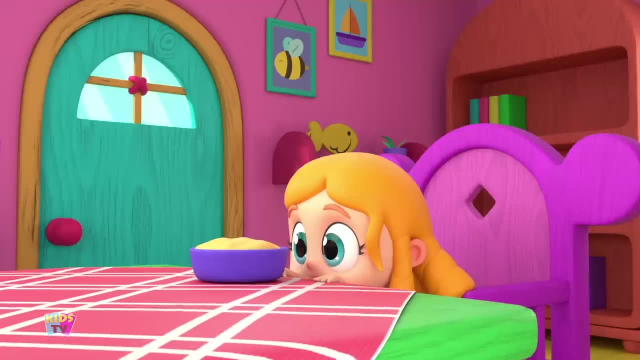 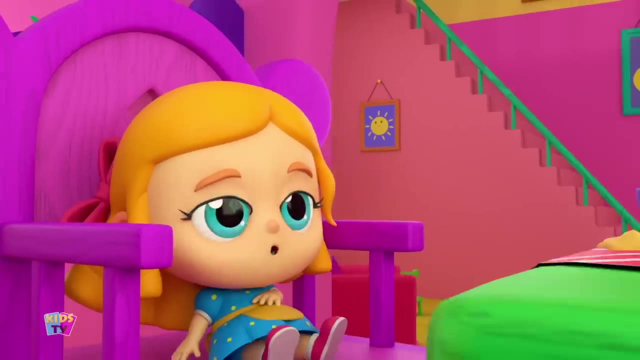 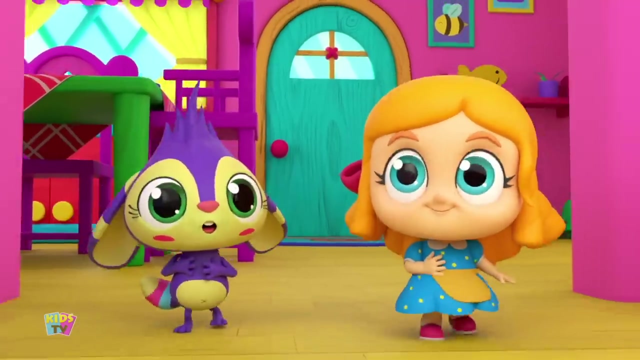 though she had no permission. Papa bear's porridge way too hot, Mama bear's porridge way too cold, Baby bear's porridge- just right, just right, just right. After Goldie had her fill, she felt lazy and tired. In the living room she spied chairs of three different sizes. 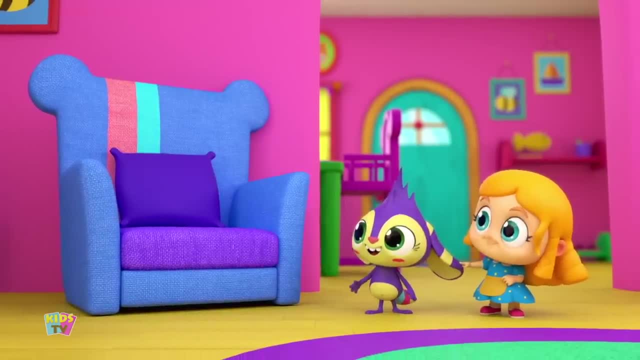 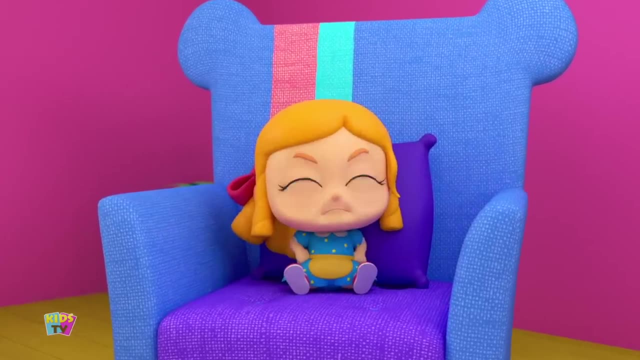 They looked quite inviting, so Goldie thought she'd try them. Papa bear's chair way too hot. Mama bear's porridge way too hot. Mama bear's porridge way too hot. Mama bear's porridge way too. 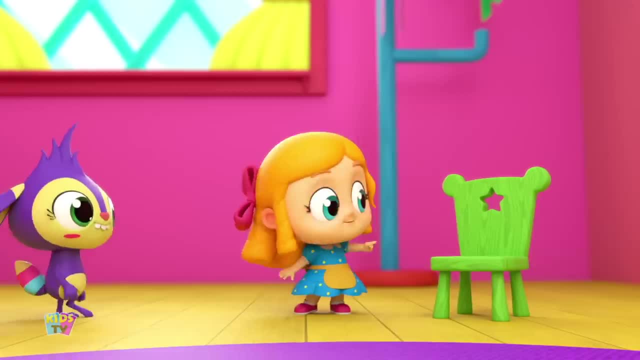 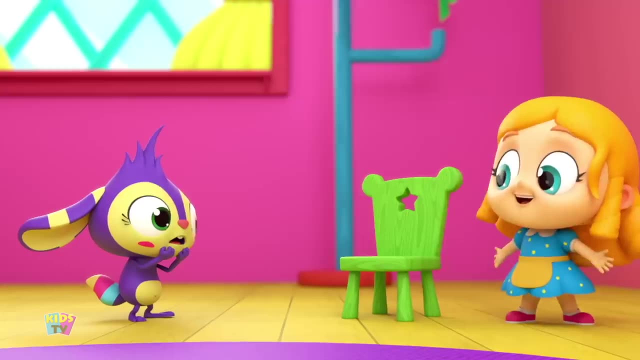 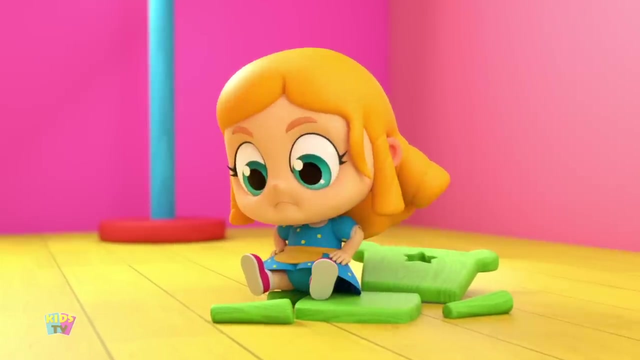 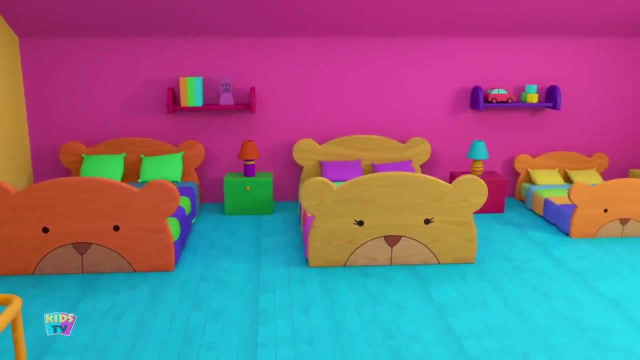 Mama Bear's chair- way too soft, Baby Bear's chair, just right, just right, just right. Just as Goldie settled in, that chair broke into pieces. Goldie went upstairs and found three nice beds she could sleep in. They looked quite inviting. so Papa's bed- she creeped in. 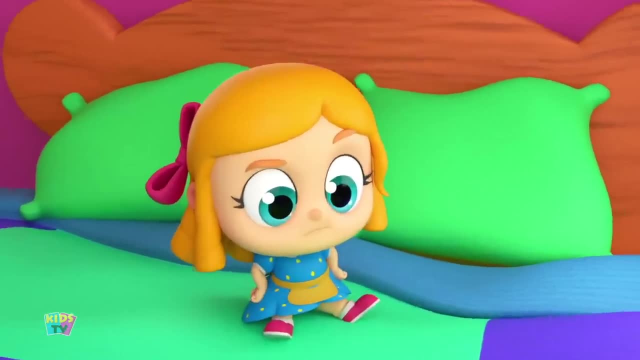 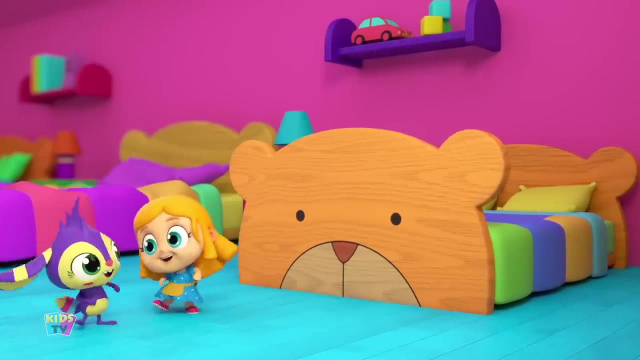 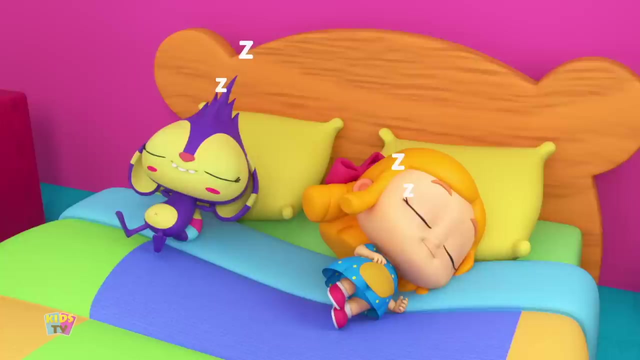 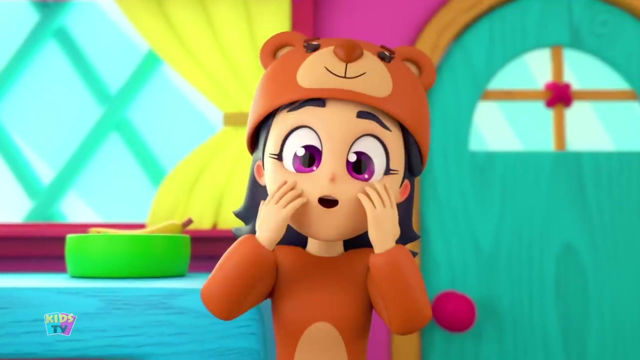 Papa Bear's bed way too hard. Mama Bear's bed way too soft, Baby Bear's bed- just right, just right, just right. Goldie Locks fell fast asleep. three bears came back home. Soon, as they stepped in, they knew they were not alone. 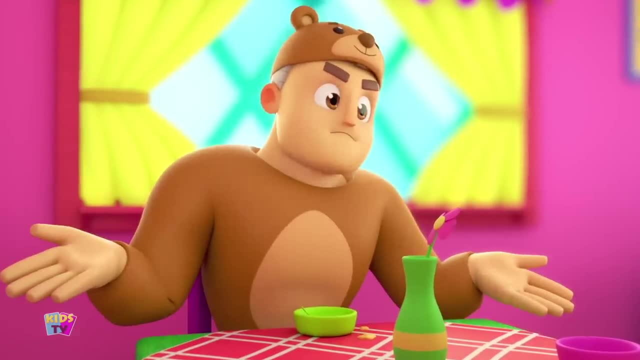 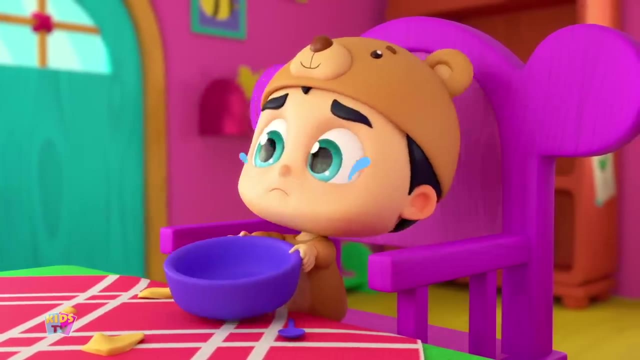 Grr, someone's been eating my poke, Growl Papa. Grr, someone's been eating my poke, Someone's been eating my porridge. Said Mama, Someone's been eating my porridge, Cried Baby, And they ate it all up, ate it all up. 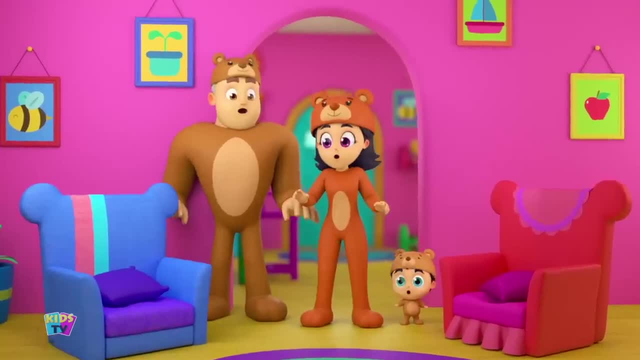 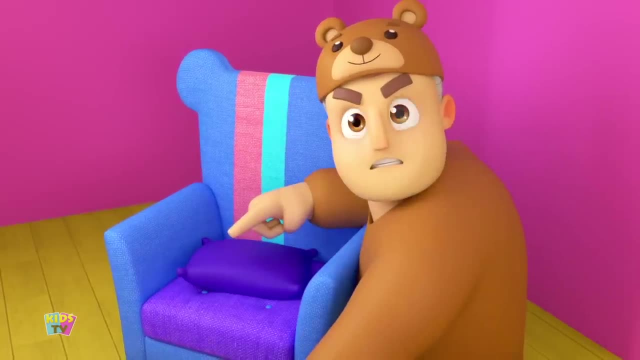 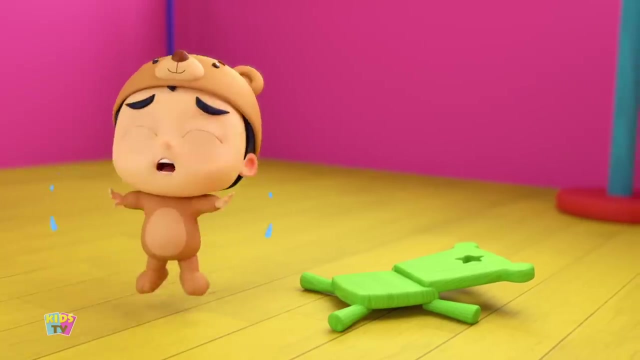 They walked into the living room And what do you think they noticed: Grr, someone's been sitting in my chair, Growl Papa, Someone's been sitting in my chair, Said Mama, Someone's been sitting in my chair, Cried Baby, And they've broken it up. broken it up. 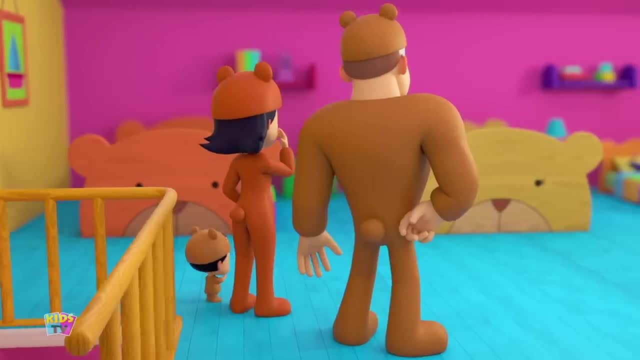 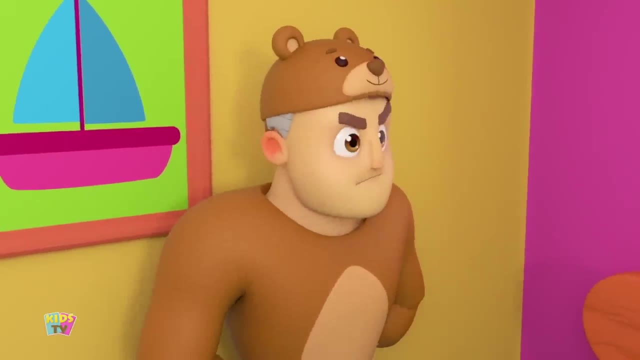 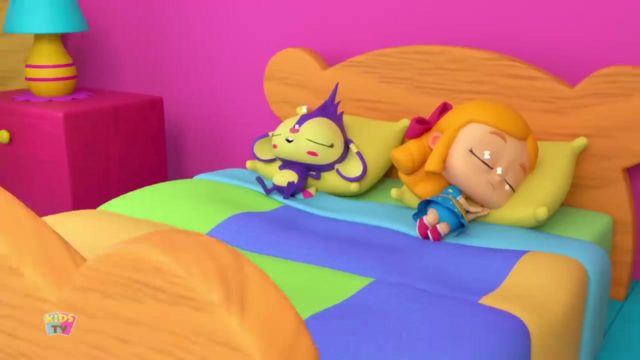 Upstairs in their bedroom. now What do you think? they noticed: Grr, someone's been sleeping in my bed, Growl, Papa, Someone's been sleeping in my bed. Said Mama, Someone's been sleeping in my bed, Cried Baby. And there she is. there she is. 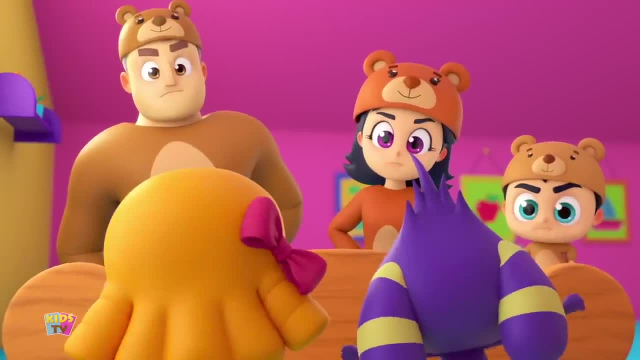 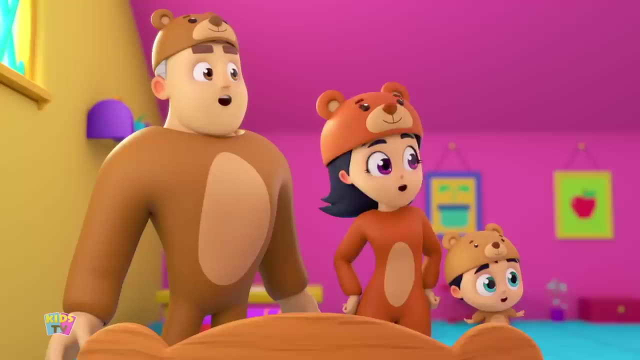 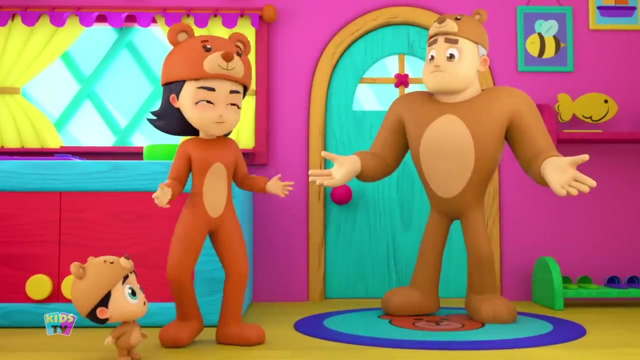 Goldie Locks woke up and saw three brown bears staring at her. She screamed Help, Jumped out of bed and ran away from her bed And ran away with a clatter Down the stairs and through the door. Goldie's gone forevermore. Our three bears. 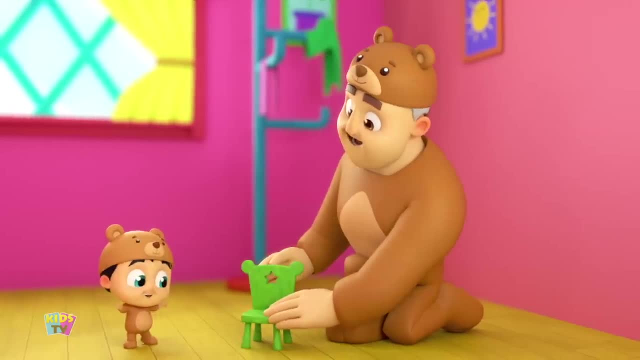 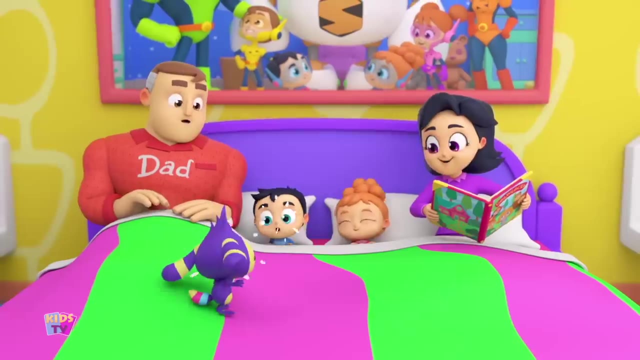 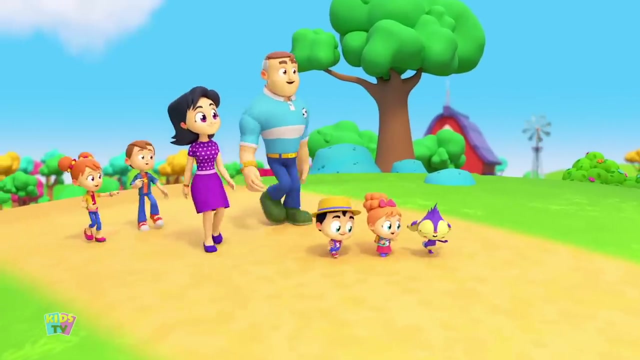 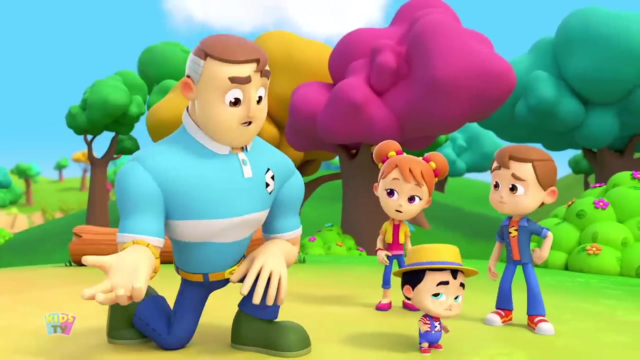 They scratched their heads, Fixed the chair and made the beds And sat down to eat their porridge. And that is the story of the three bears. Yeah, Buggy, did you just take Huggy's apple? No, Hey, my apple's gone. 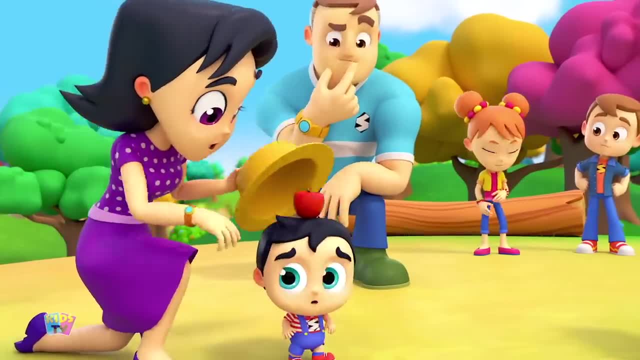 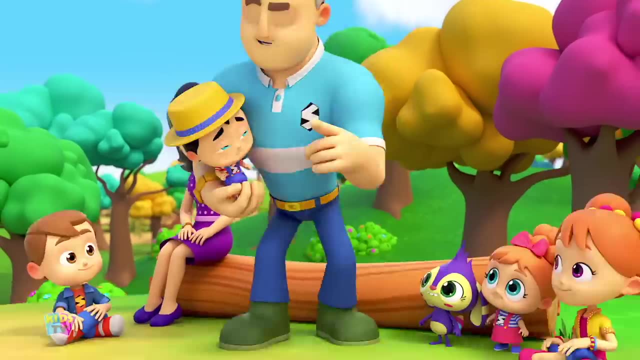 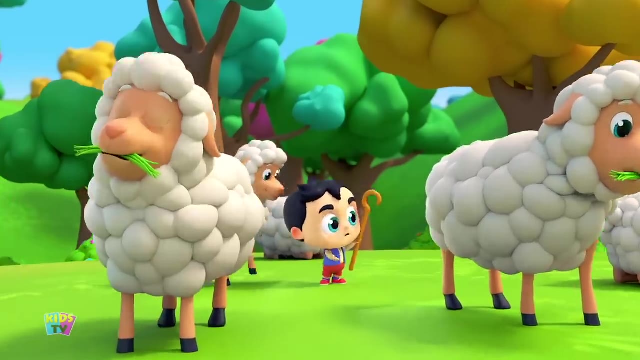 It wasn't me. Well, Buggy, what's that? Um, Hmm, I think it might be a good time to tell you a story, Buggy, There was a boy who watched the sheep- The silliest boy you ever did see One sunny day. 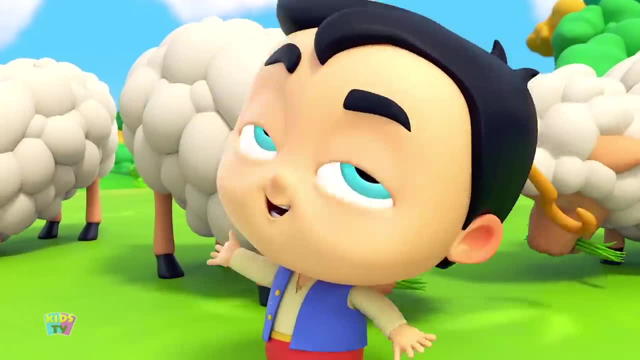 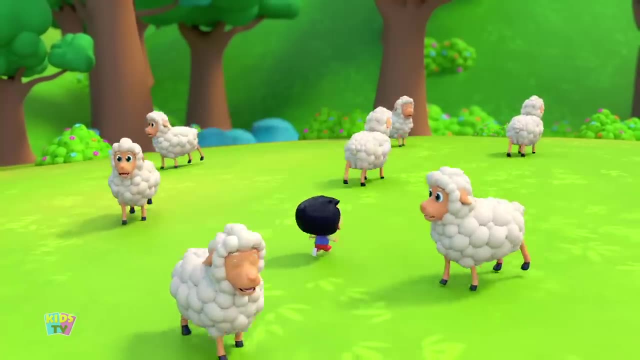 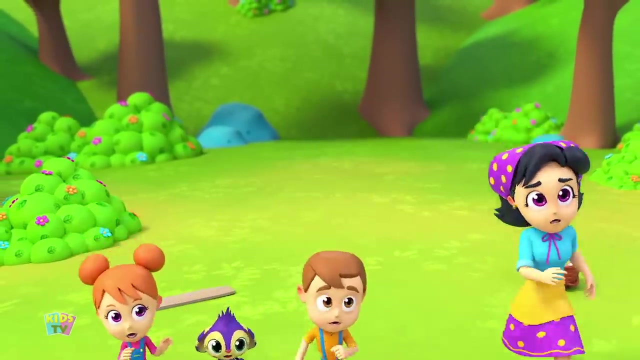 Who knows why He thought for fun He'd tell a lie. The boy cried: Wolf, Please, please come, Hurry, Hurry, Run, run, run. And up the hill A farmer came To chase that wolf away. again There was no wolf. 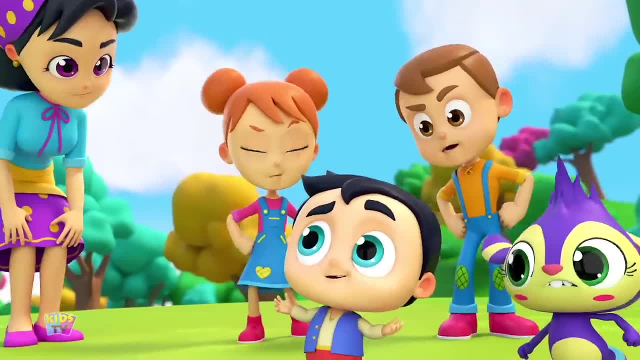 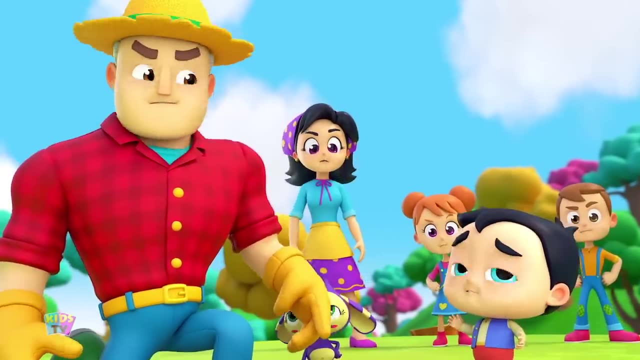 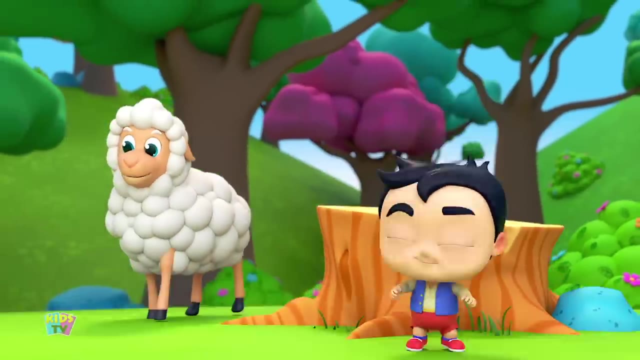 Not even one, It's just a trick I played for fun. The farmer said: See here, young man, Don't play that trick on me again. Okay, I promise. The very next day At half past ten, The silly boy cried Wolf, Wolf again And up the hill. 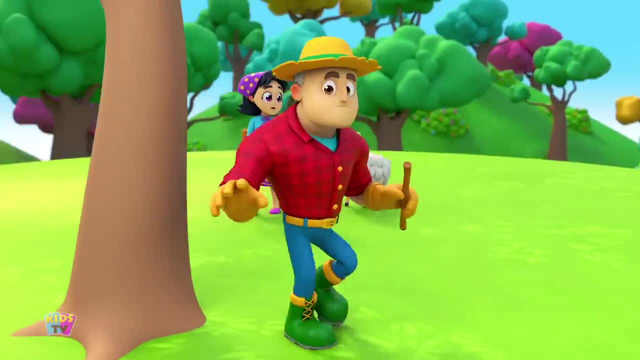 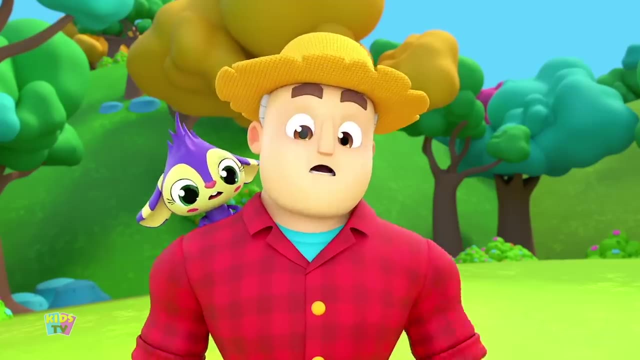 The farmer came To chase that wolf away. again, There was no wolf, Not even one. It's just a trick I played for fun. The farmer said: See here, young man, Don't play that trick on me again. See here, young man, Don't play that trick on me again. 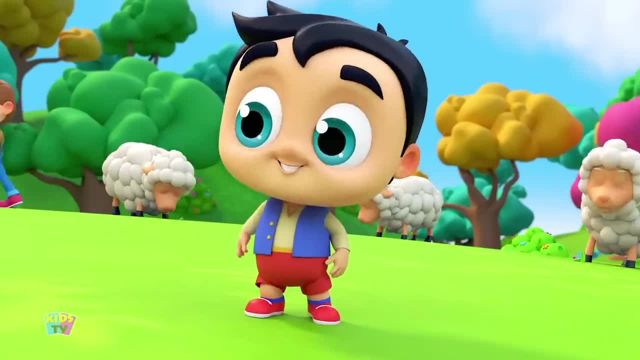 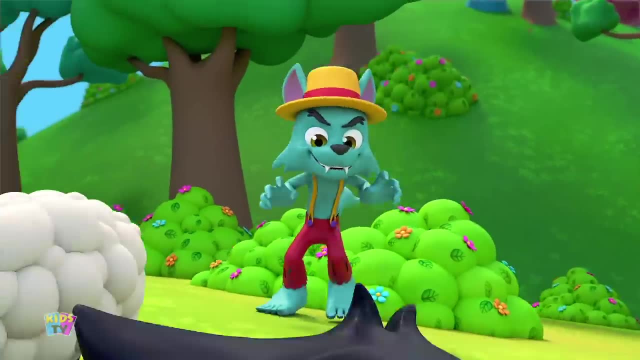 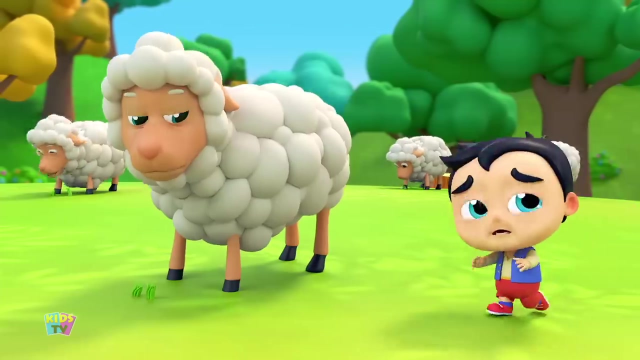 Okay, I promise. But that same day, At quarter past two, A big, bad wolf Came into view, Into the field. The wolf did creak To scare the boy And steal the sheep. The boy cried: Wolf, Please, please come, Hurry, Hurry. 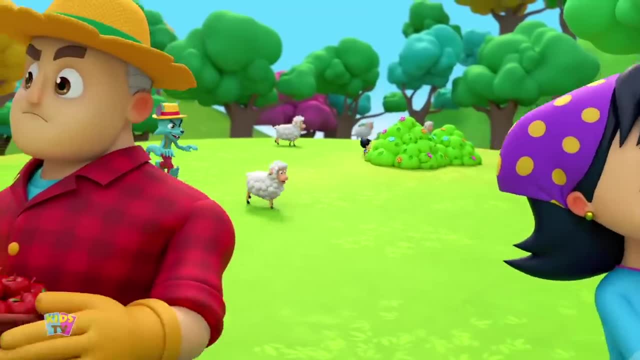 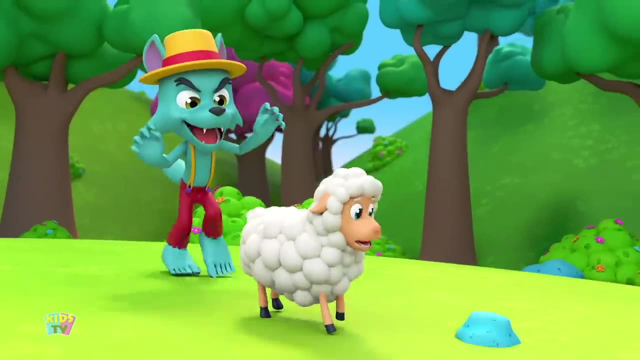 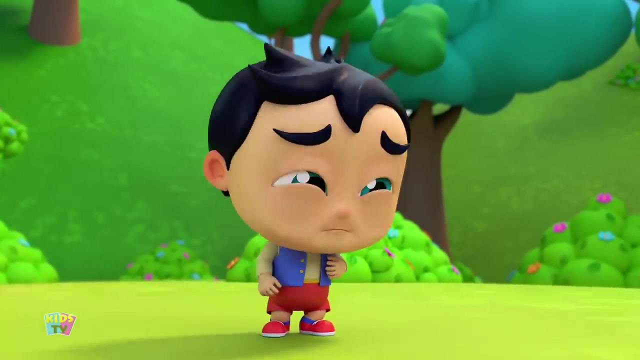 Run, run, run, Wolf Wolf. It's not a game, Please come now. But no one came. The farmer said The silly boy, He shook with fright That wolf stole Every sheep in sight. The little boy Was very sad Because he knew That he'd been banned. 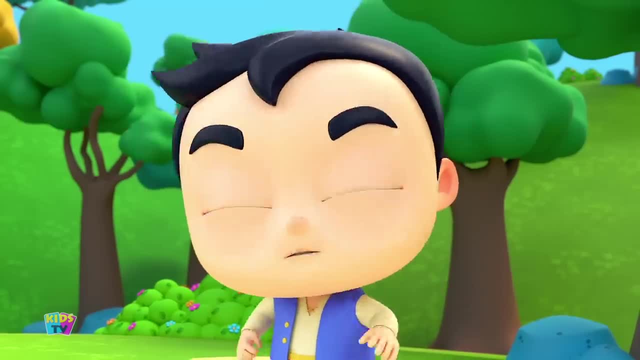 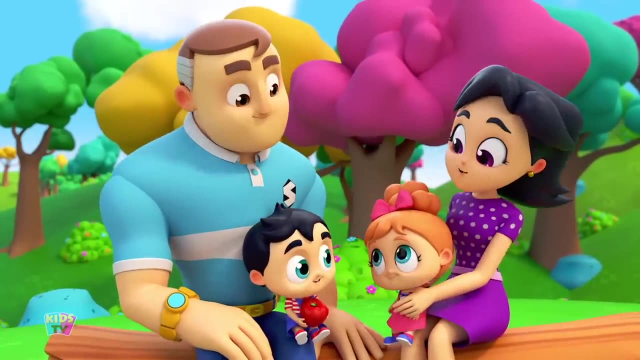 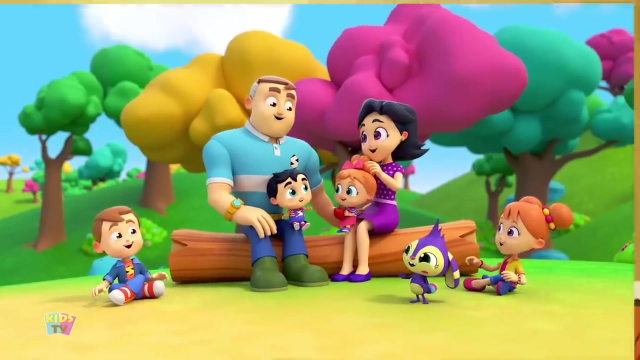 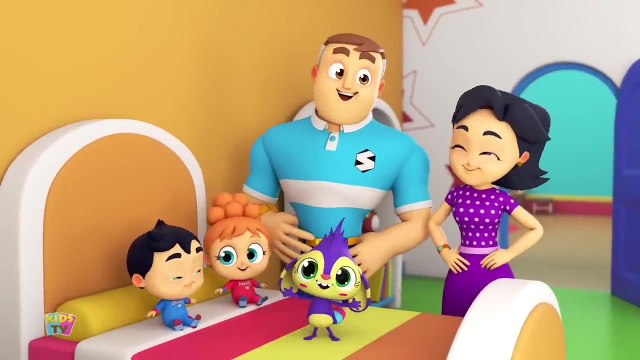 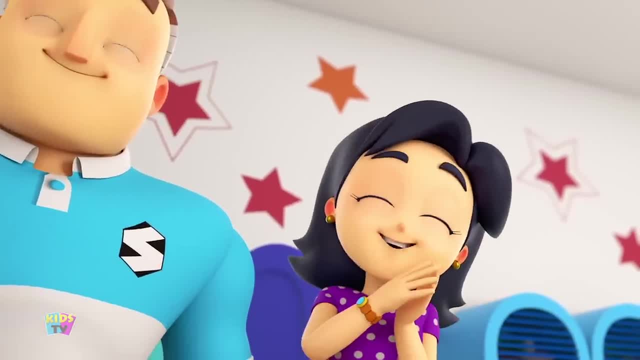 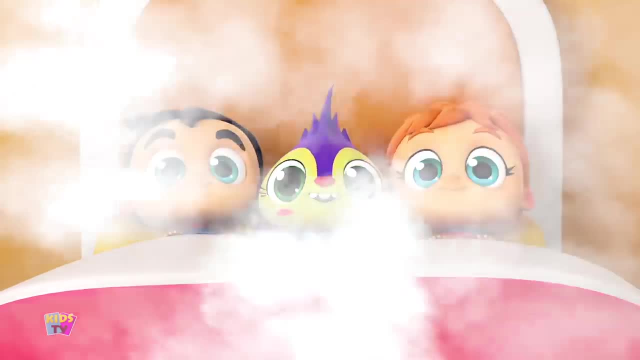 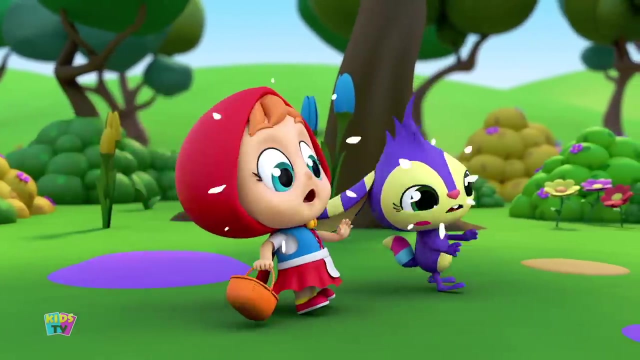 Yeah, read us a story. Okay, you two Snuggle in and close your eyes, And I'll read you the story Of Little Red Riding Hood. Yay, Little Red Riding Hood Went out one day. Uh-huh, uh-huh, She was going to grannies far away. uh-huh, uh-huh. 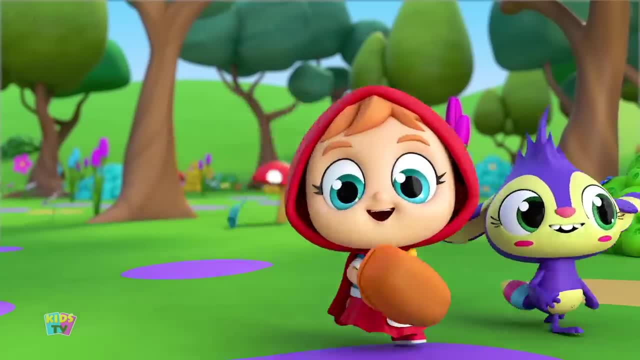 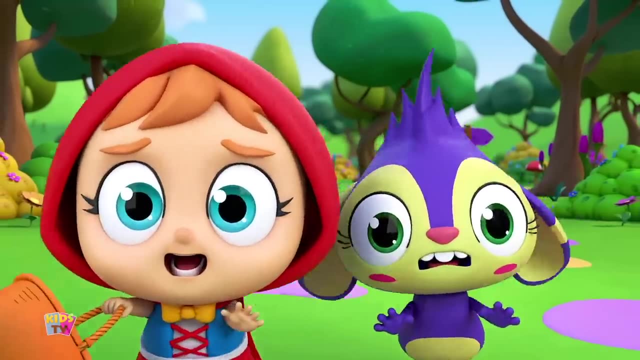 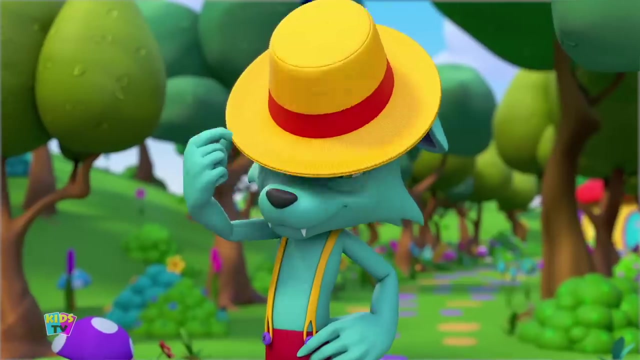 She followed a path through the deep dark woods To get to grannies as quick as she could. uh-huh, uh-huh, uh-huh, A big bad wolf came into view. uh-huh, uh-huh, He raised his hat and said: how do you do? 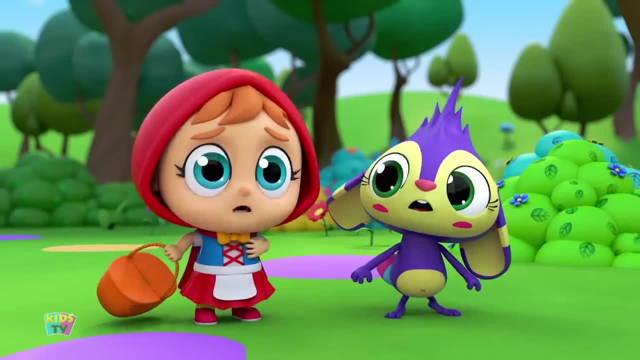 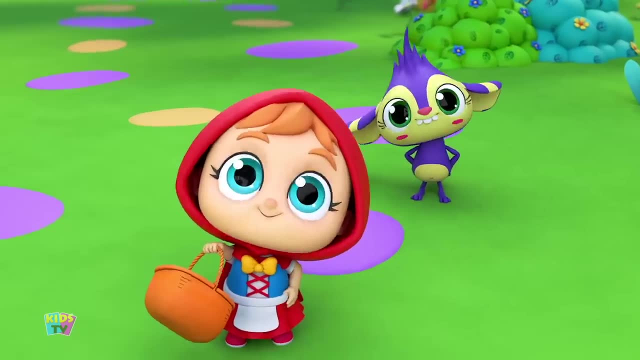 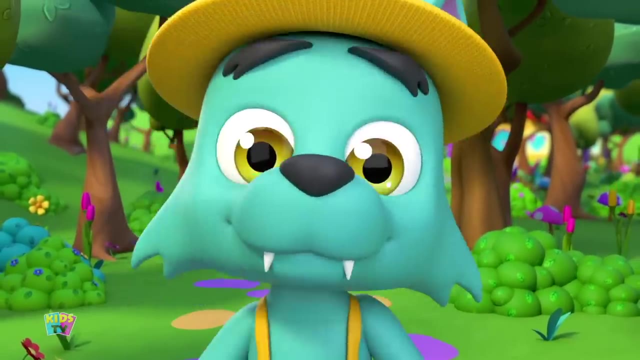 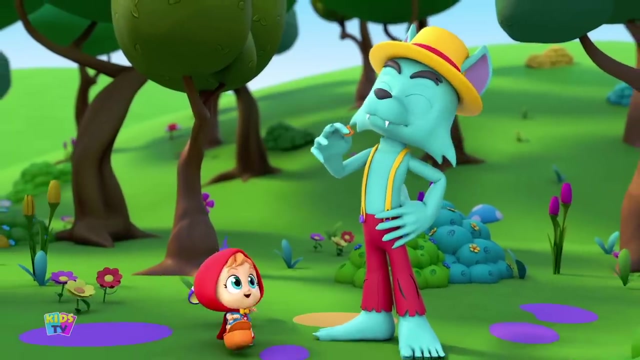 Uh-huh, uh-huh. She said: my granny is feeling ill. I'm bringing her cookies to make her well. Uh-huh, uh-huh, uh-huh, Said Little Red Riding Hood. I must run. Uh-huh, uh-huh. 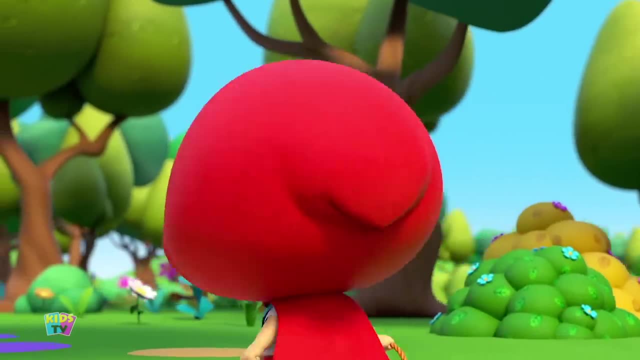 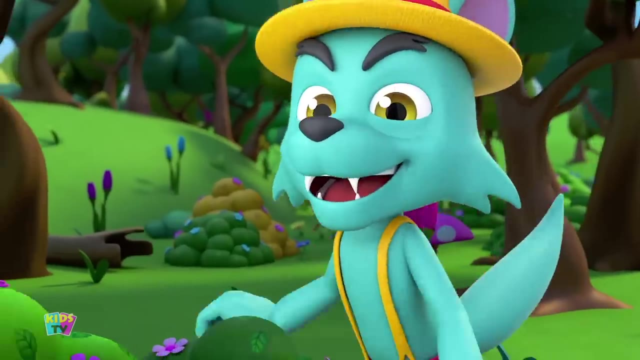 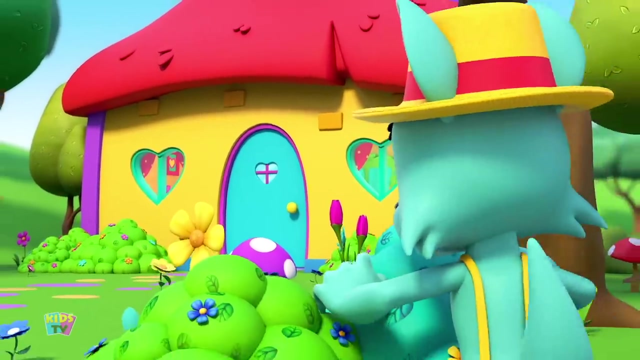 I'm expected at grannies at half-past One. uh-huh, uh-huh. She said good day And she walked away, But the big bad wolf knew a faster way. Uh-huh, uh-huh, uh-huh. The big bad wolf came to grannies' house. 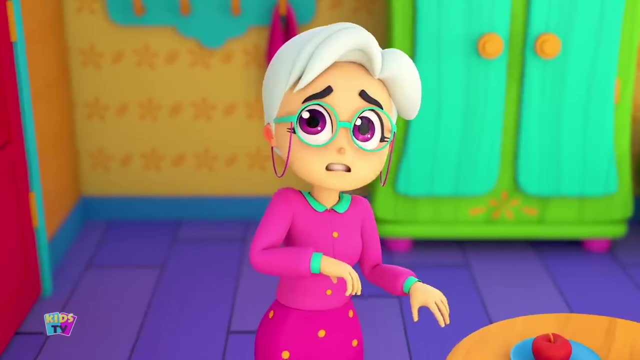 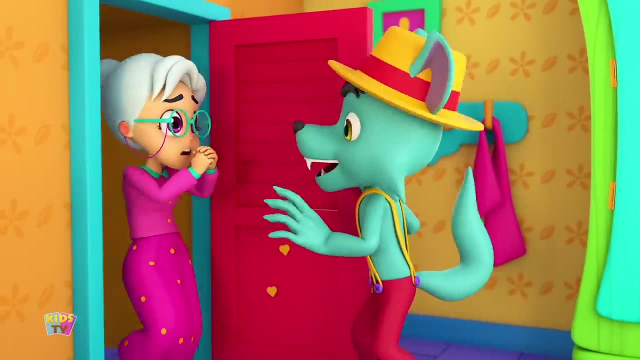 Uh-huh, uh-huh. And poor old granny was all alone. Uh-huh, uh-huh, Granny, get in the cupboard. That bad wolf said. Then he put on her clothes And jumped out of the house And went to bed. Uh-huh, uh-huh, uh-huh. 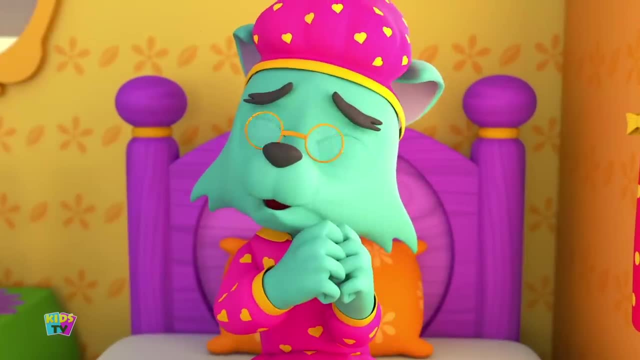 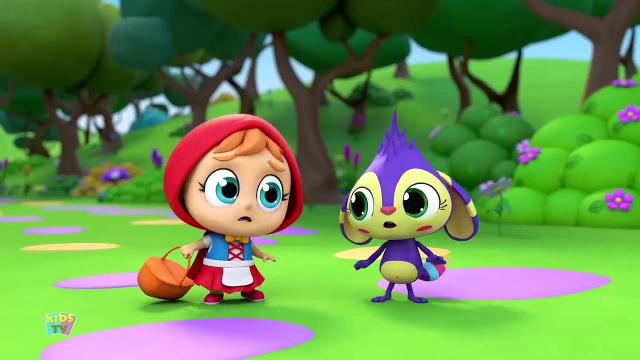 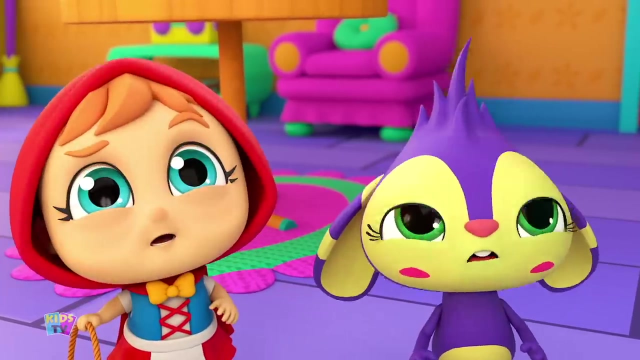 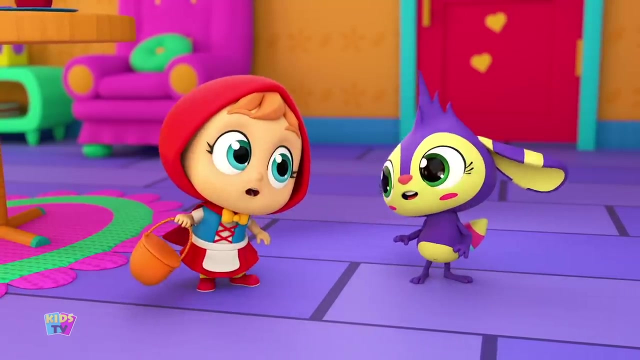 Then in came Little Red Riding Hood. Uh-huh, uh-huh, Dear granny. I came as quick as I could. Uh-huh, uh-huh. The wolf said, dear, come over here. But the little girl knew something was weird. Uh-huh, uh-huh, uh-huh. 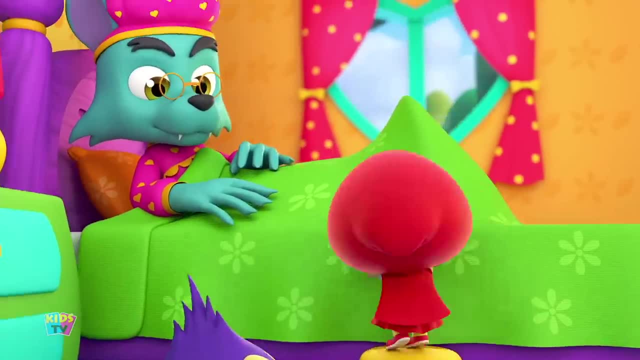 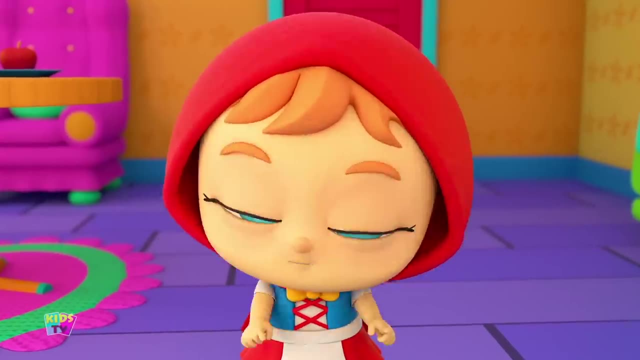 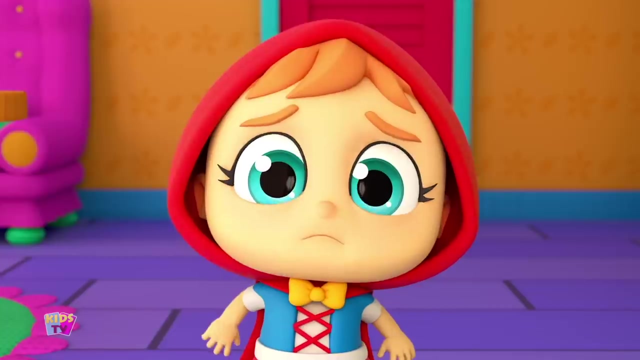 Uh-huh, uh-huh, uh-huh, Granny, what great big ears you have. Uh-huh, uh-huh, Granny, what great big eyes you have. Uh-huh, uh-huh, Granny, what great big teeth you have. The wolf said better to eat you with. 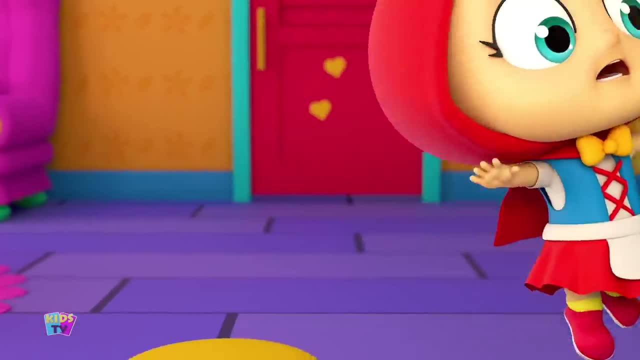 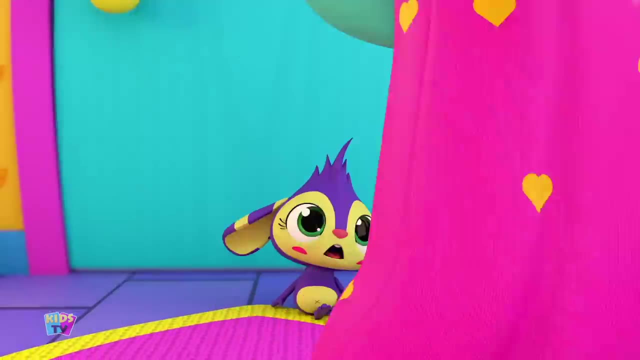 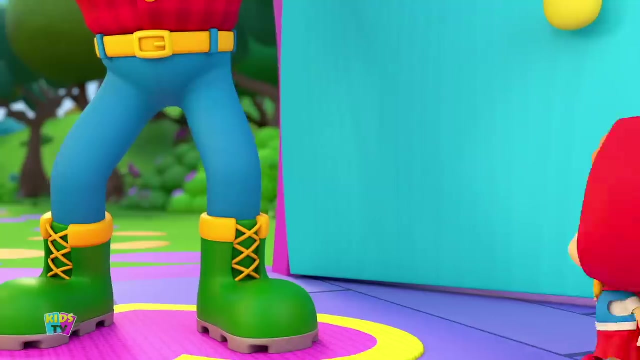 Uh-huh, uh-huh, uh-huh. Help, Cried Little Red Riding Hood. Uh-huh, uh-huh, uh-huh. And in ran a hunter who was in the woods. Uh-huh, uh-huh, uh-huh. 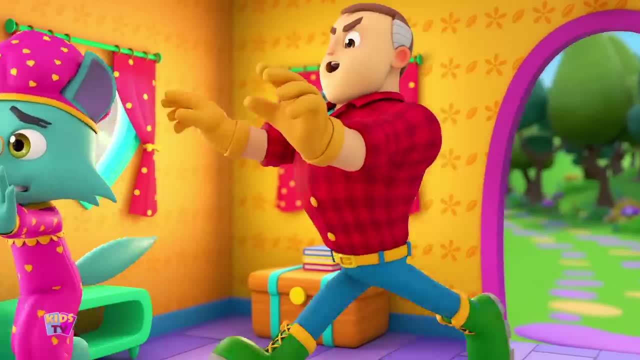 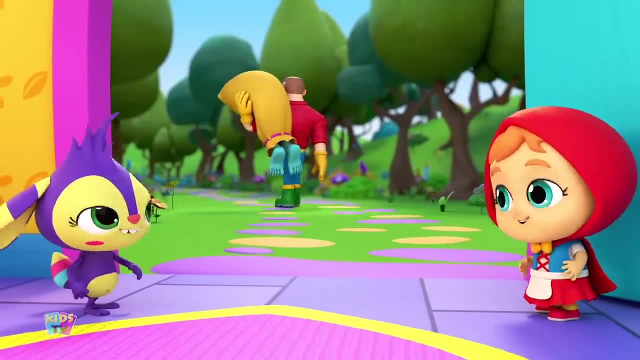 The hunter grabbed the wolf And he put him in a sack. And the big bad wolf, he never came back. Uh-huh, uh-huh, uh-huh. We're safe now, granny. The little girl said Uh-huh, uh-huh, uh-huh. 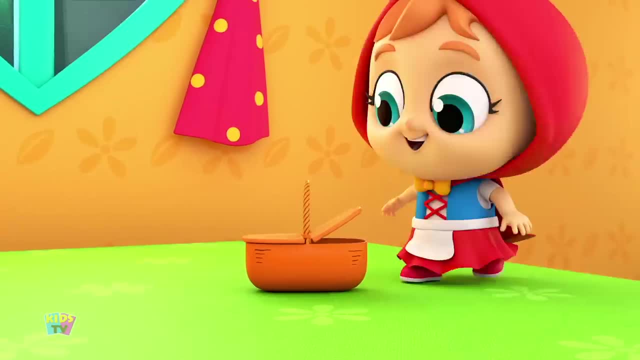 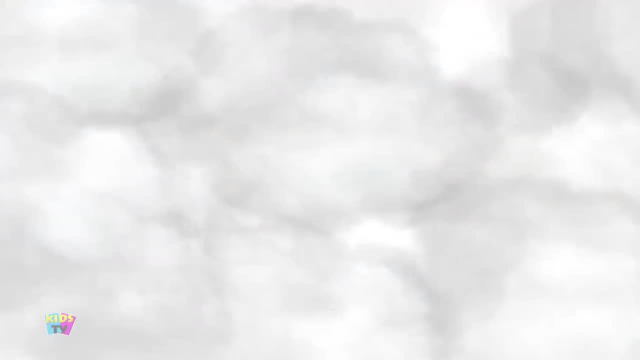 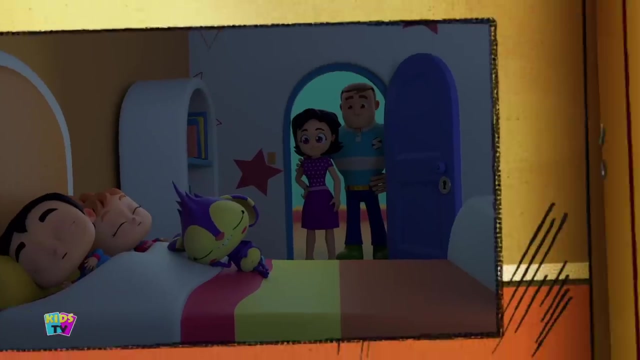 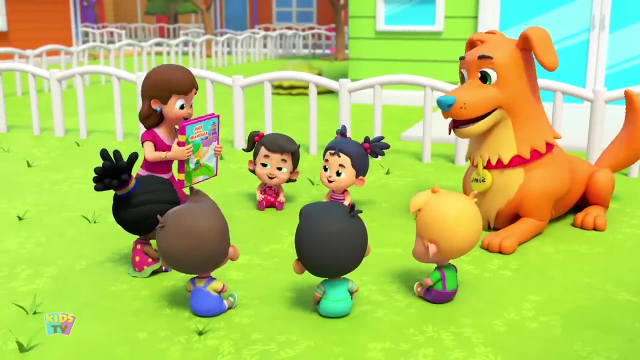 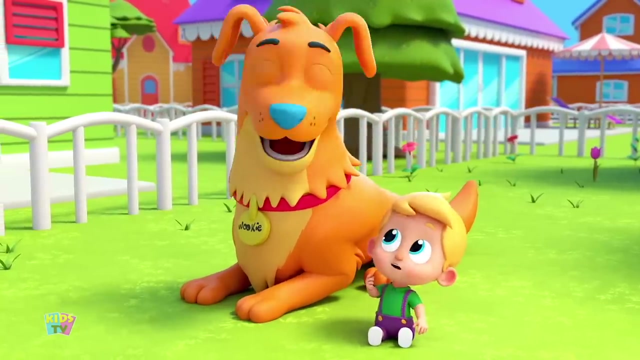 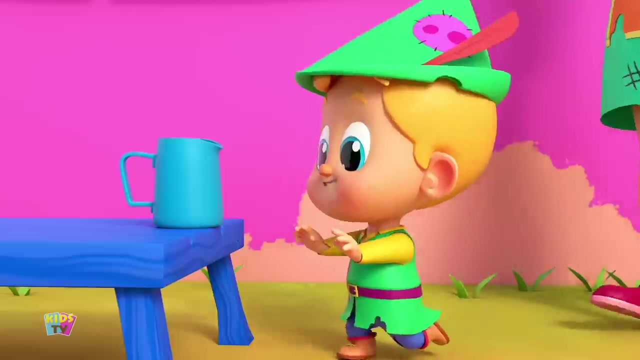 And she helped granny get back. Uh-huh, uh-huh, They ate the cookies happily And that's the end of our story. Uh-huh, uh-huh, uh-huh. Well, let's find out. Long ago, Jack and his mom Lived their life on a country farm. 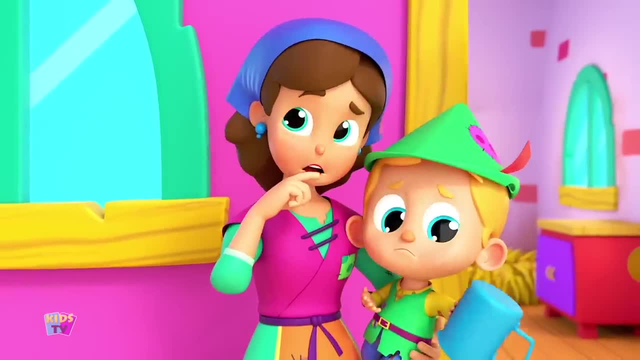 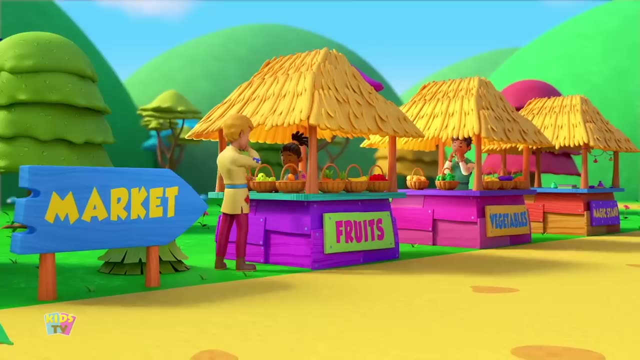 They were poor, not enough to eat. So they made a plan to make ends meet Jack. go sell our cow Bessie, And with the money we can grow more crops On market day. Jack sold old Bess To a funny lass who was oddly dressed. 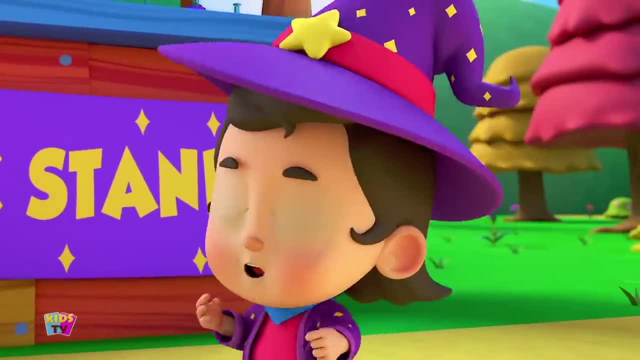 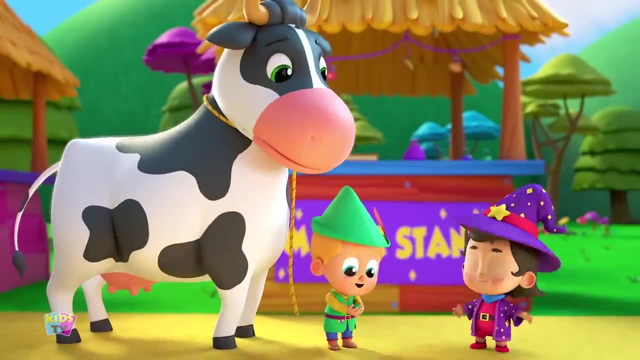 Hello young man. she politely bowed. I'll trade you beans for that. No, no, no, no, no. The milking cow, they're magic beans And they'll grow a crop as high as the sky. Jack went home to show his mom. 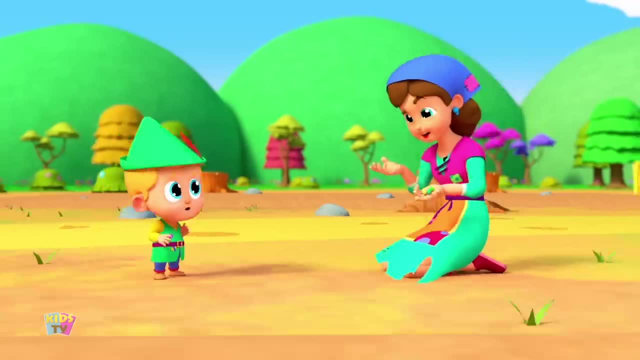 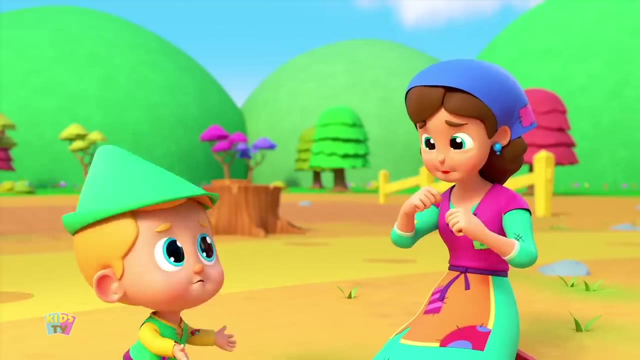 But when she saw what he had done, She threw away the beans outside. Oh Jack, just beans. oh my, She cried. But but mom, they're magic beans. Oh, magic, sh-magic. Then next day, where the beans did land, 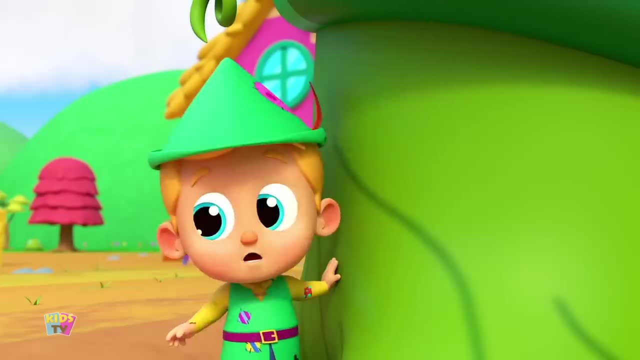 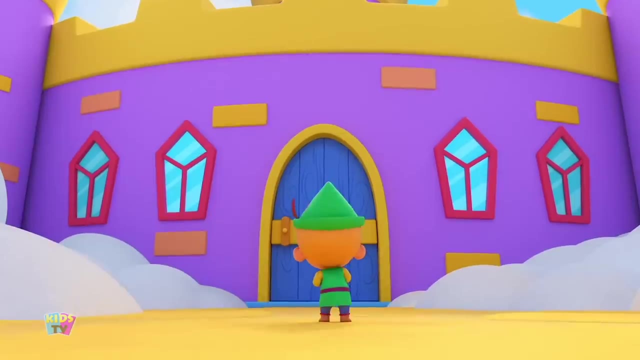 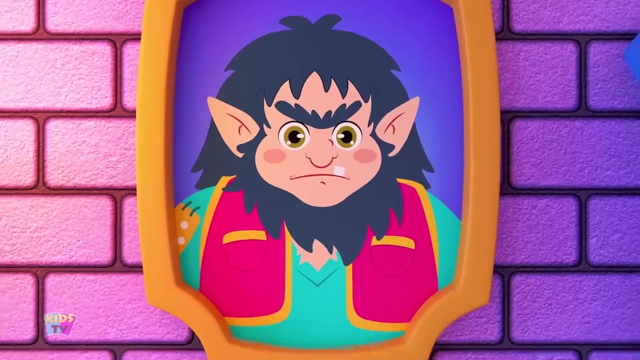 A giant beanstalk grew. Oh man, Jack climbed those twisty Vines so high And found a castle in the sky- Wa-ha, Look at that. But when he went inside the place, A big fat giant with an ugly face Came thumping in, so very loud. 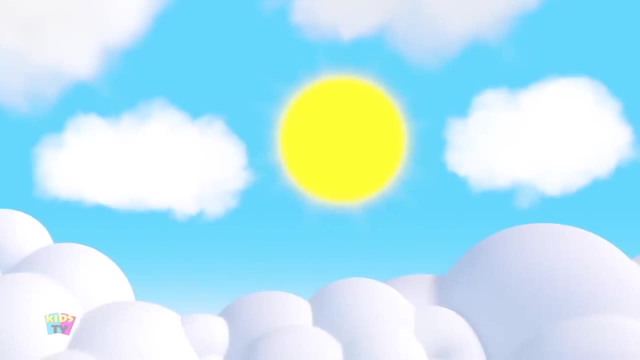 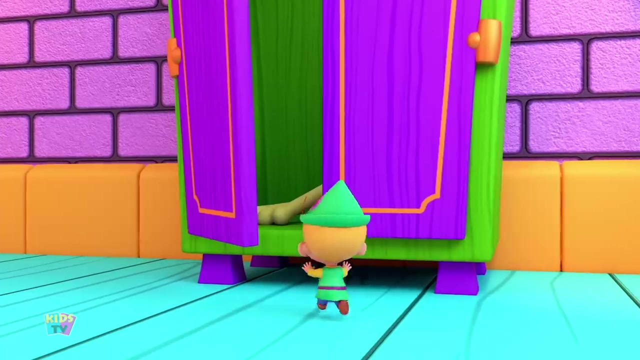 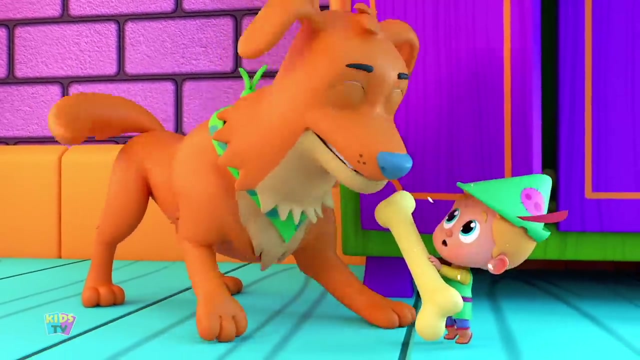 Shook the heavens and the clouds. Fee-fi-fo-fum, I smell a boy. Yum yum, yum, Fee-fi-fo-fum, Ready or not, here I come. Jack was so frightened That he hid in the cupboard While the giant counted his gold. 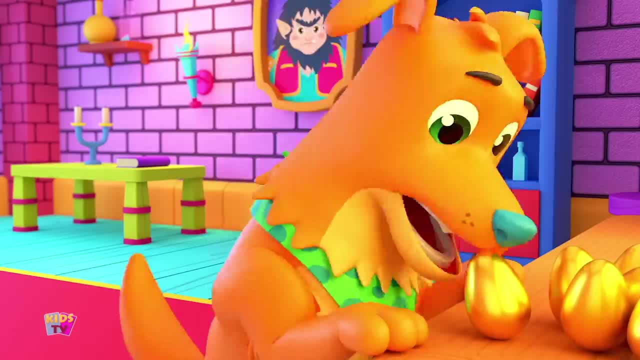 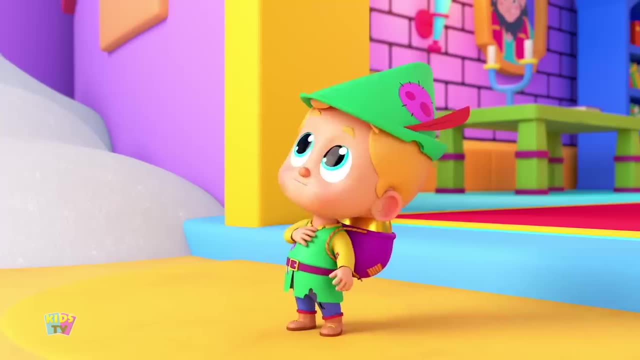 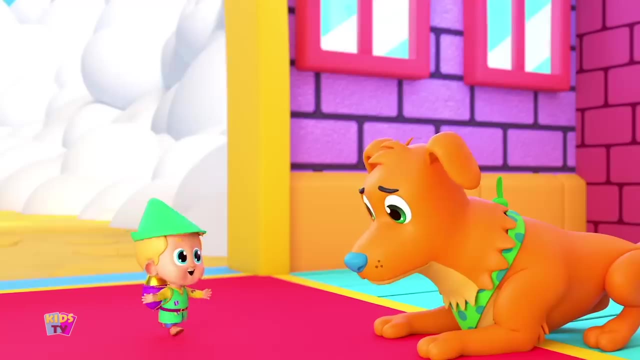 When the big old giant fell asleep, Jack escaped with gold to keep, Decided he'd go back up there. But first I'd better say a prayer: Oh please, oh please, Keep me safe from the mean old giant. He climbed up to the castle and hid inside. 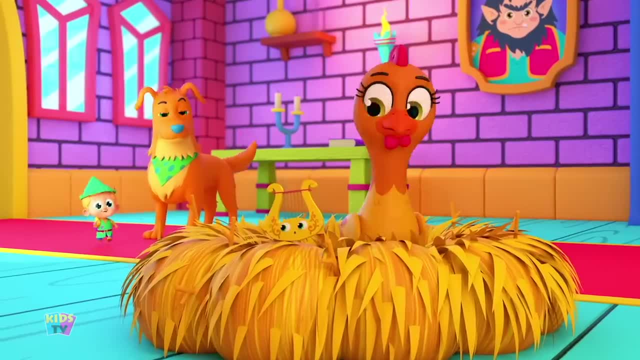 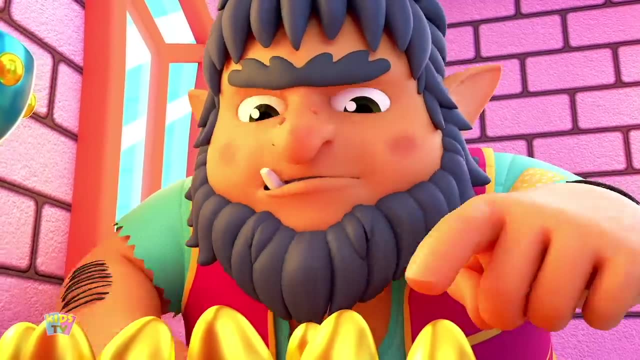 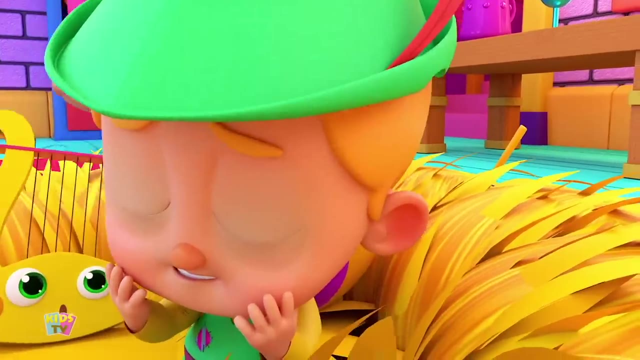 Ah-ha, He said, the giant's pride, Golden eggs from that little hand. The giant counted at least ten, One, two, three, four, five. Uh, what comes after five? Fee-fi-fo-fum, I smell a boy. Yum, yum, yum. 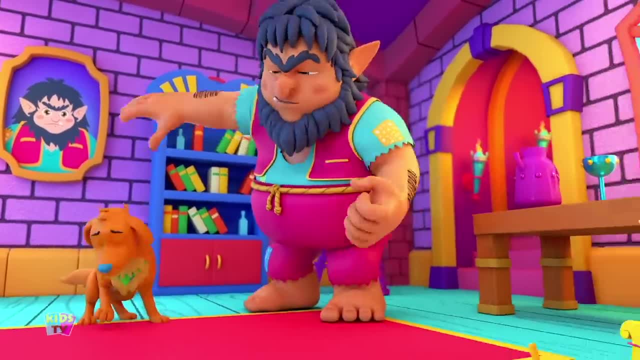 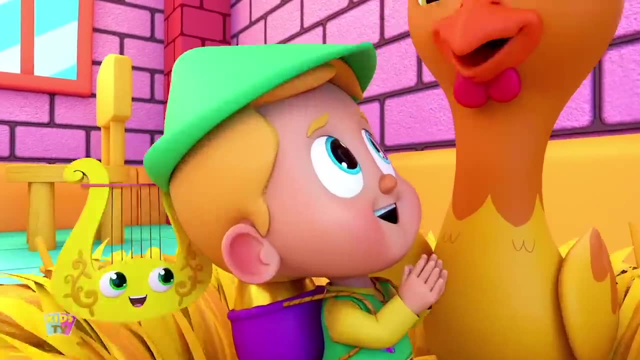 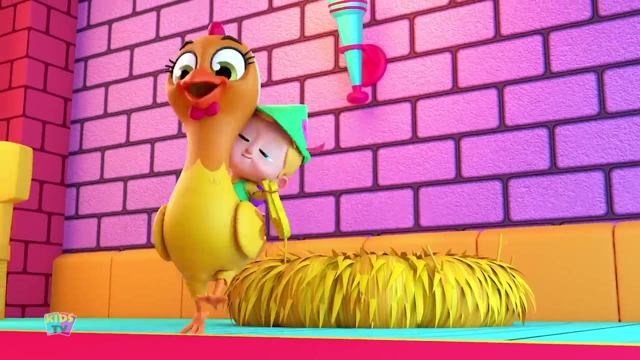 Fee-fi-fo-fum. Ready or not, here I come. Oh yikes, Ah, Jack's being nimble, Jack's being quick. Oops, Wrong story. Jack was fast and acted quick. He grabbed that fine white little hand, Even grabbed a singing harp. 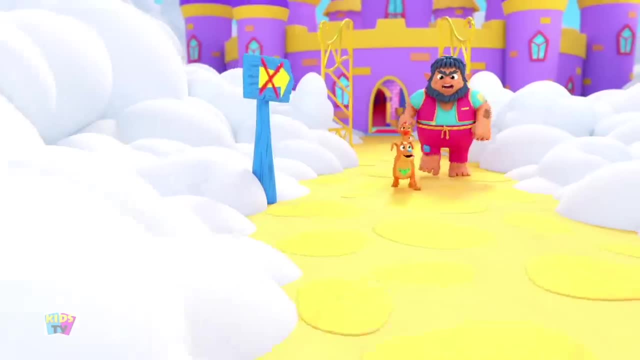 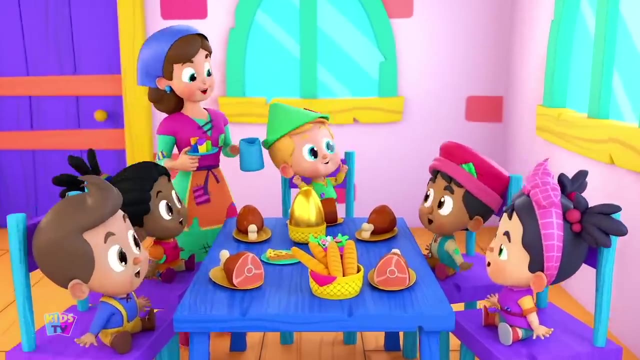 And climbed down that stalk again La-la. But the giant came thudgering after Jack And threw himself on the beanstalk. When I got home I grabbed an axe And chopped that beanstalk all the way down And that big old giant went hurtling off. 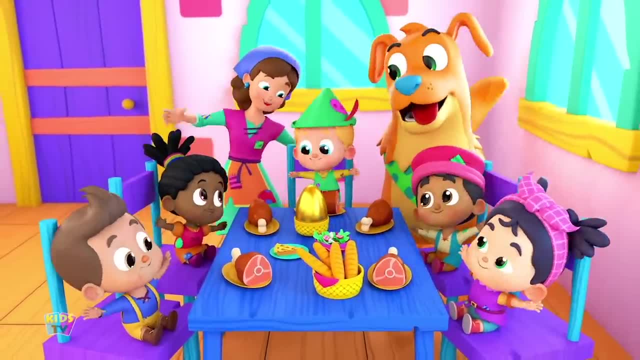 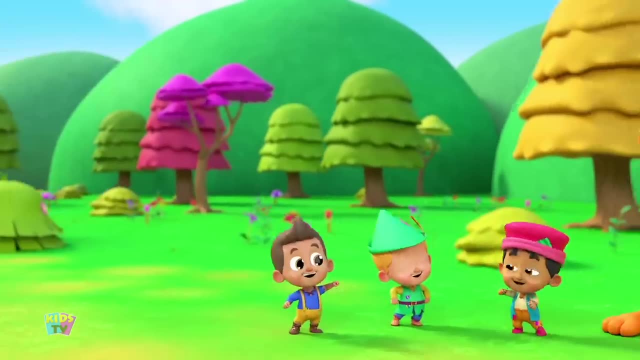 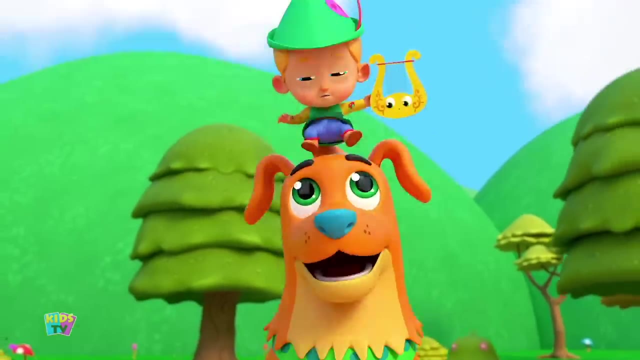 No, Never ever to be found. With the hen's golden eggs, Jack and his mom could now live a good life. Jack's mom was proud and made a feast, And neighbors came from near and far. The harp played songs and sang along. Jack, you are a shining star. 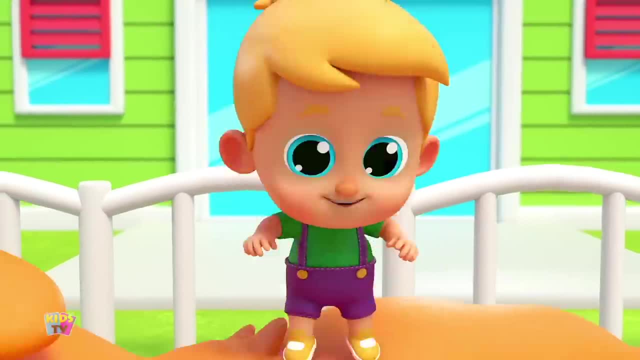 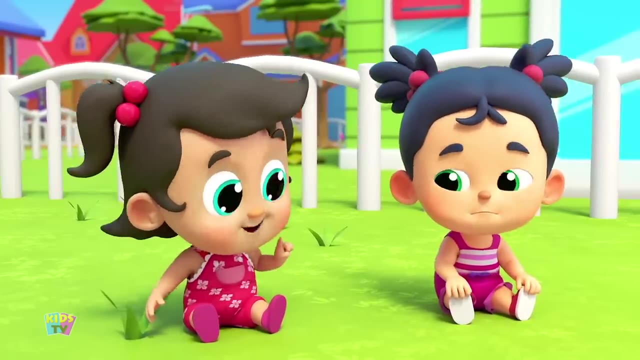 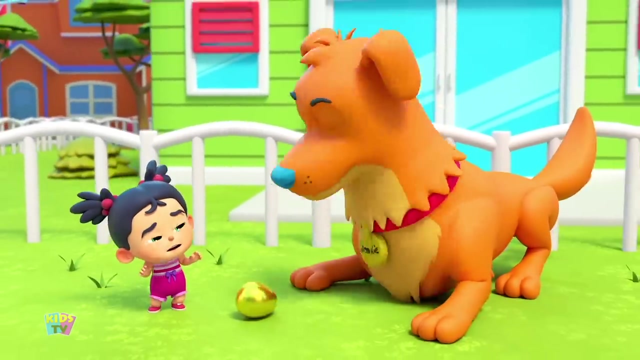 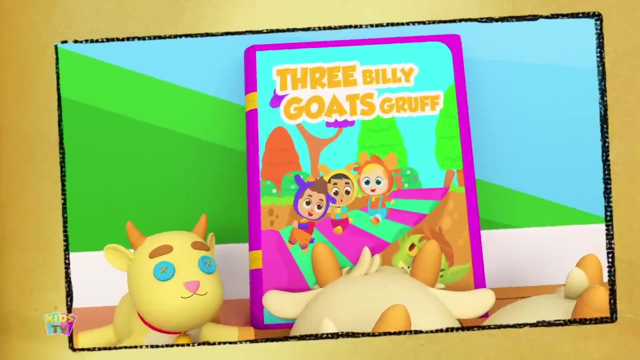 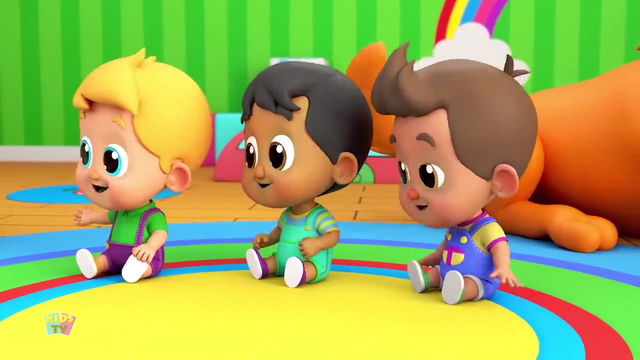 Jack, you are a star. So did they make beanstalk soup? No, but now they had a hen that laid golden eggs. Oh, but you could break your teeth on those. I think it's my turn to tell a story. Okay, but can we be in it? 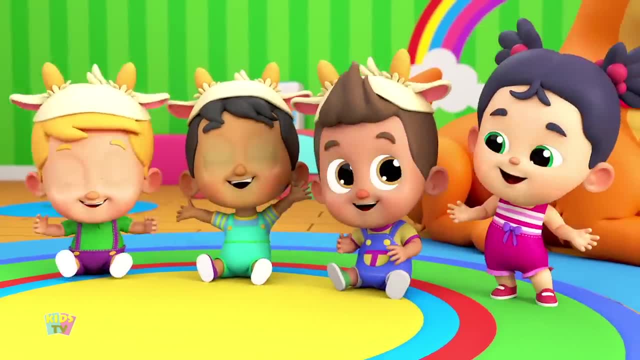 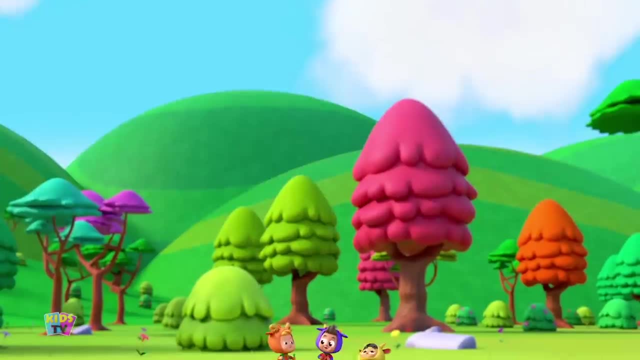 Sure, I need three filly goats. Archie, Luca, you in. Yeah, Tell us the story of the three fillies. Three filly goats gruff Gruff. Three filly goats gruff. Set off to the hills To eat green grass And get their fill. 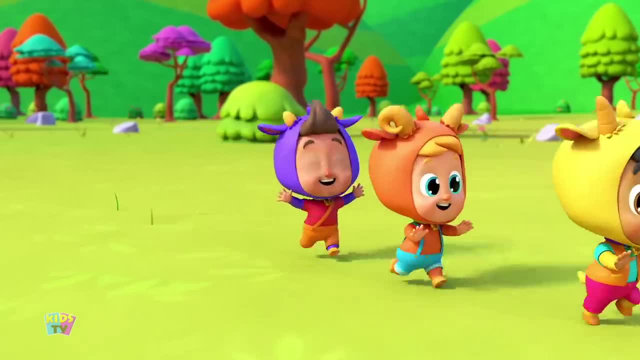 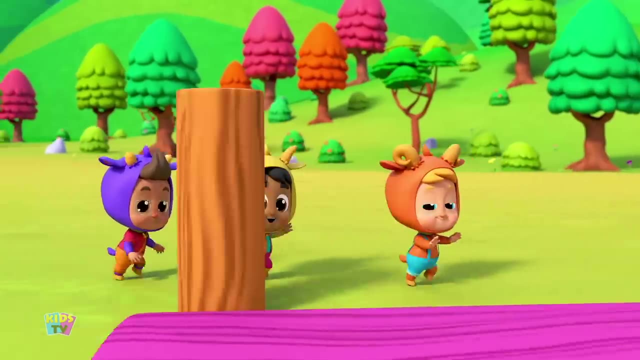 They ate sweet grass All day long. They ate and ate Till it was gone. Oh, look at that, Oh, fresh green grass Across the river. The little goats spied A field of grass on the other side. Cross the bridge and you'd pay a toll. 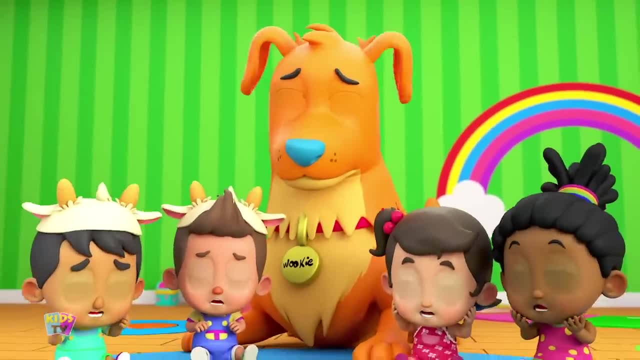 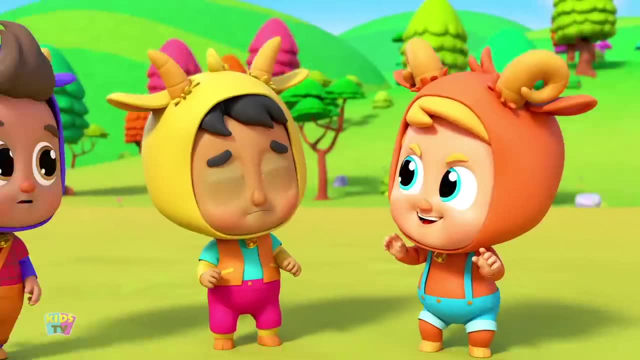 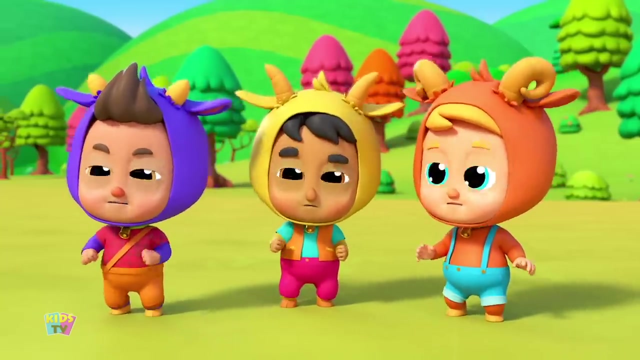 Not with coins. you'd feed the troll. Oh my, The three filly goats gruff were very scared of the troll, But they were also very hungry. Little filly goat gruff just couldn't wait any longer, So off he went. I may be scared, but I'm hungry too. 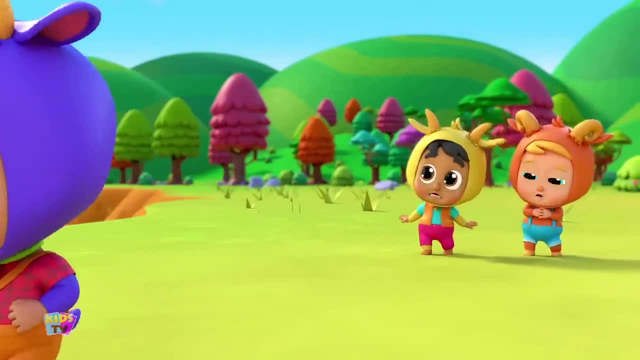 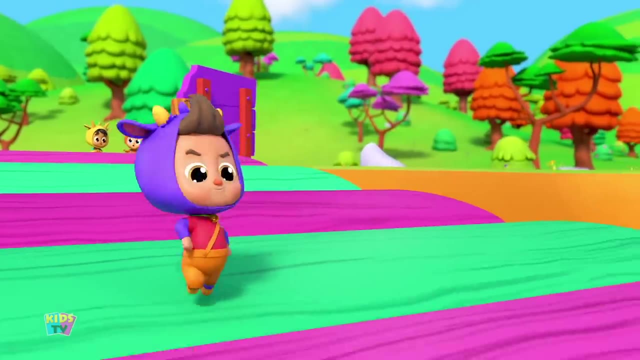 And look at all that grass. that's new. I'll cross the bridge to the other side. He may be small but at least he tries. But as the filly goat, trip-trapped by The troll, popped out of the hole, The troll popped up from under the bridge and said: 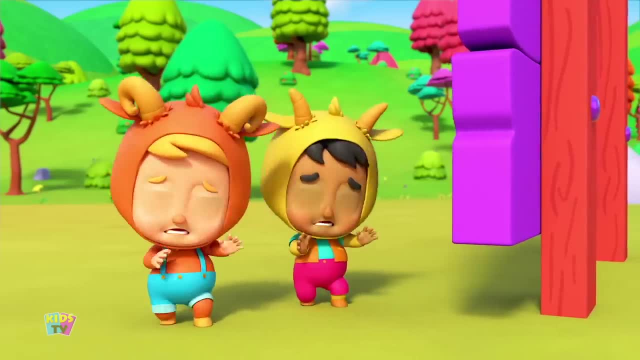 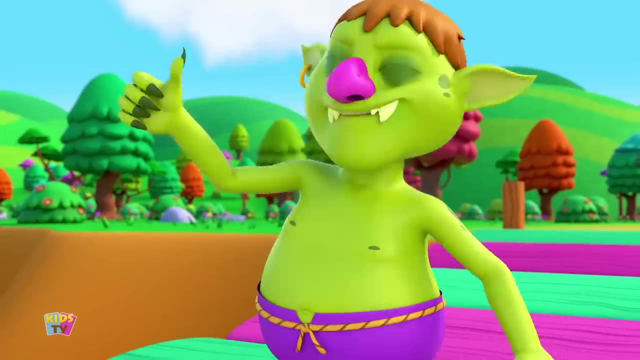 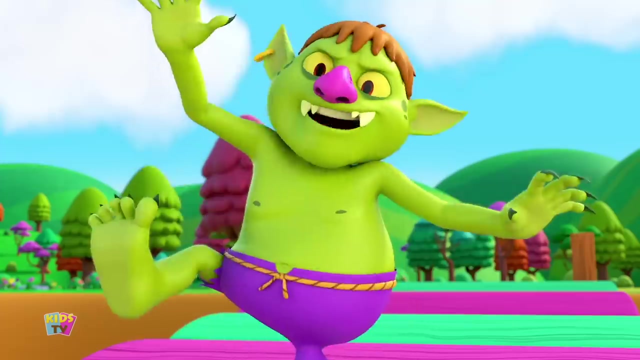 Who's not trip-trapping across my bridge? You won't get by me Because I am going to eat you. I'm a hairy troll with yellow eyes, Horrid teeth and claws. I'll eat you up if you cross my bridge With my rotten jaws. 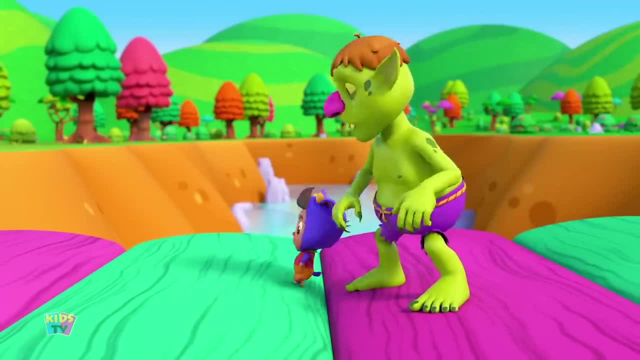 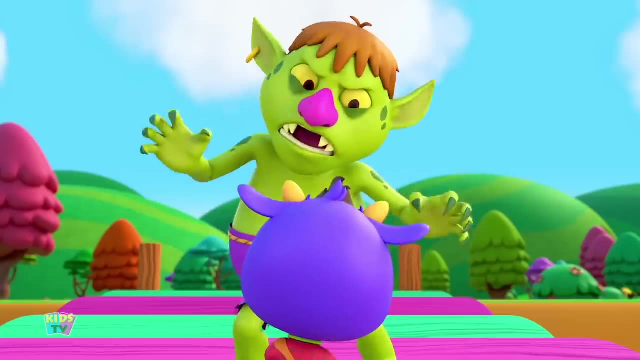 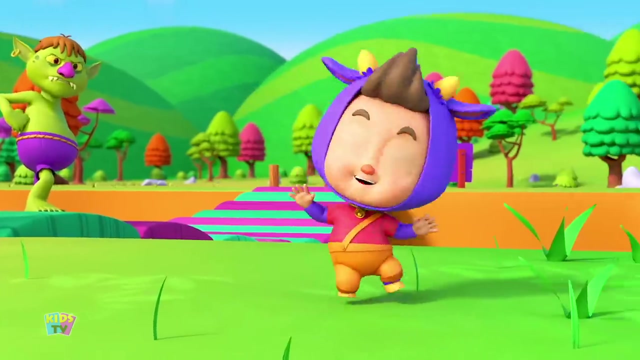 It's only me, a baby goat. I'm skinny as can be. I really wouldn't chase that troll. Good, but Middle Goat, would you see, And he'll be coming along next. Very well, ah, beat it kid Now. Middle Goat was next to cross. 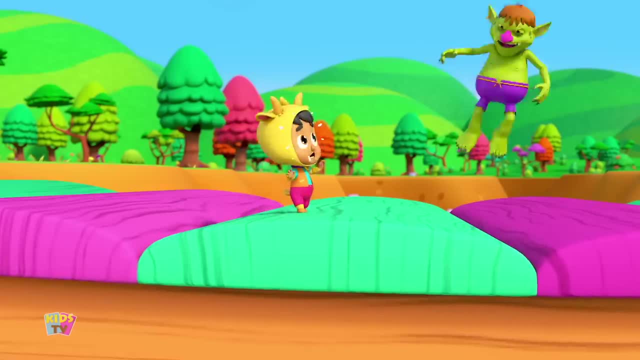 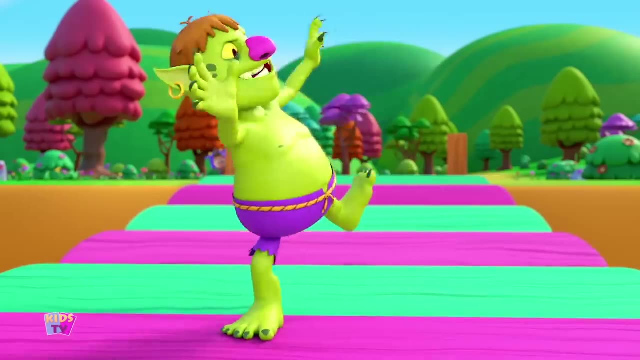 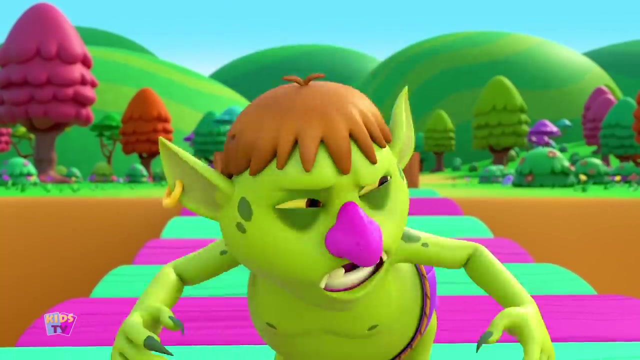 And off he went, trip-trap. But on the bridge the troll appeared. There's a tasty chap. I'm a hairy troll with yellow eyes, Horrid teeth and claws. I'll eat you if you cross my bridge, Just because Who's not trip-trapping across my bridge. 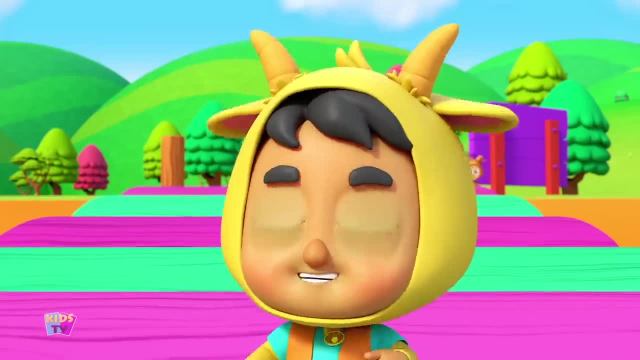 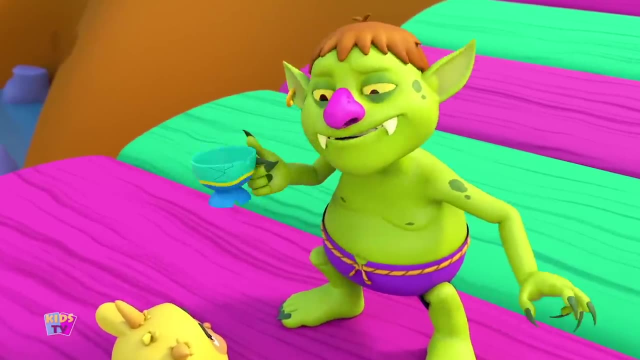 Just me, old troll. I'm off to eat that sweet green grass, Said the Middle Goat of the three. Oh no, you're not, Said the troll. I'll eat you with my teeth, But I'm almost skin and bones. you see No fat on me at all. 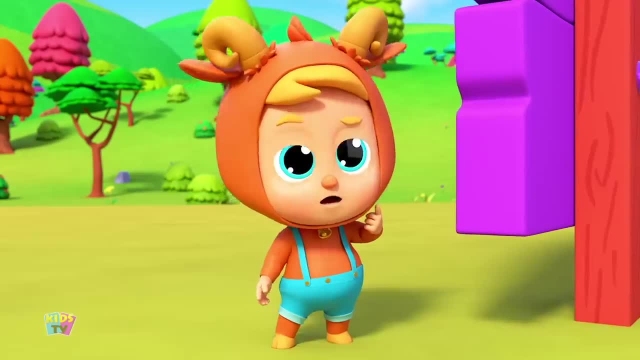 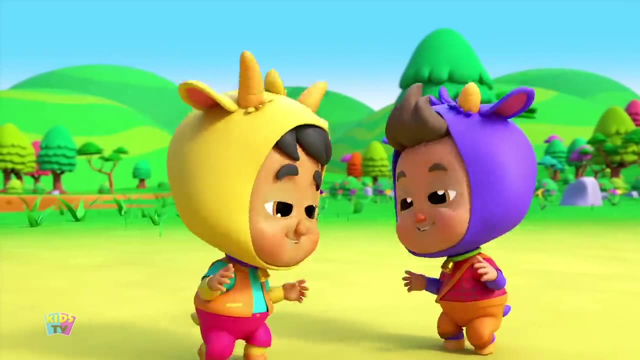 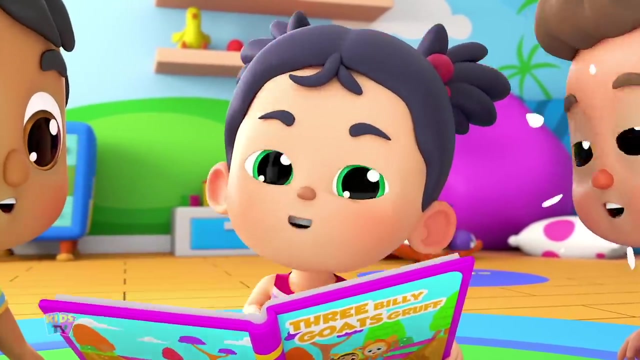 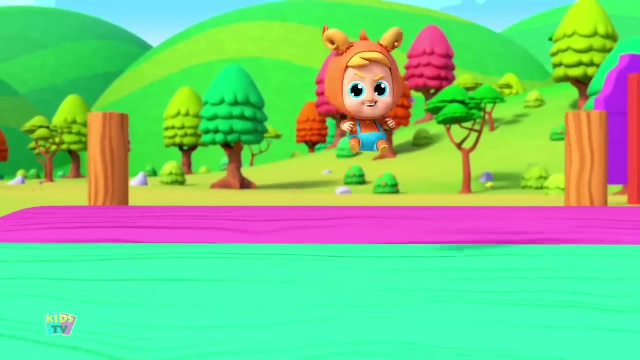 You'd really like my brother. see, He's a butterball. Oh, oh, okay, go, I wait for Big Brother. Ah, So the troll let the Middle Billy Goat gruff Cross the bridge And waited for his tasty big brother. This is not good. So over the bridge the Billy Goat tramped. 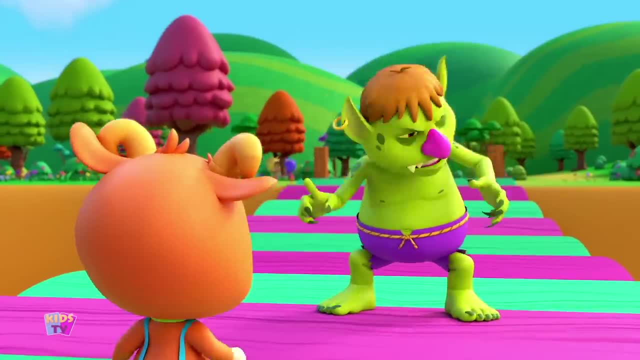 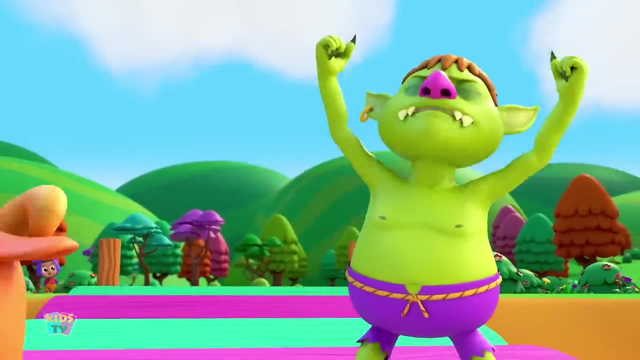 Tramp tramp on the wood. Who's that tramping on my bridge? It's Big Billy Goat, you hairy monster. Hey, that doesn't even rhyme. I'm a hairy troll with yellow eyes, Horrid teeth and claws. I'll eat you up if you cross my bridge. 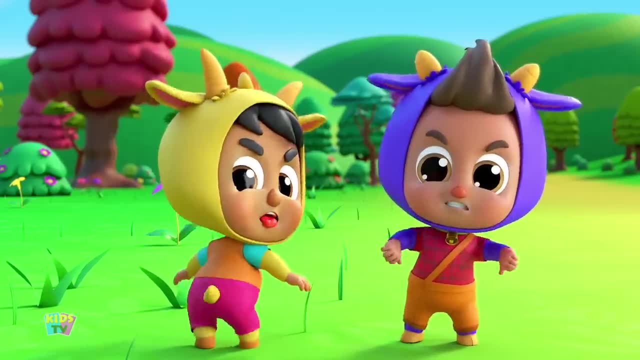 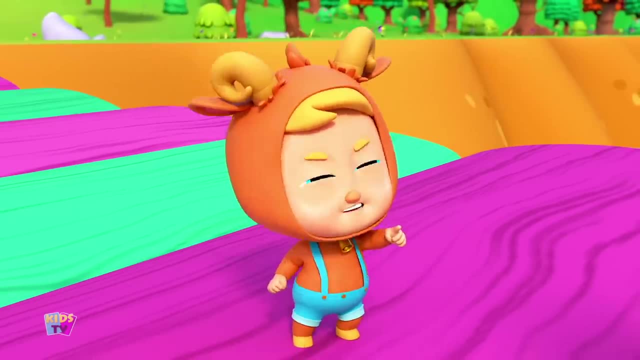 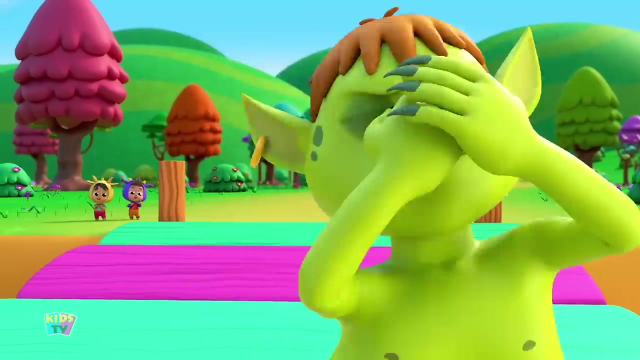 How about some applause? Oh, Be very hungry. I'm on my way to eat green grass And join my brothers too. I dare you goat to cross my path. My horns will charge you shoo. And with that the Big Billy Goat Charged the troll with his big pointy horns. 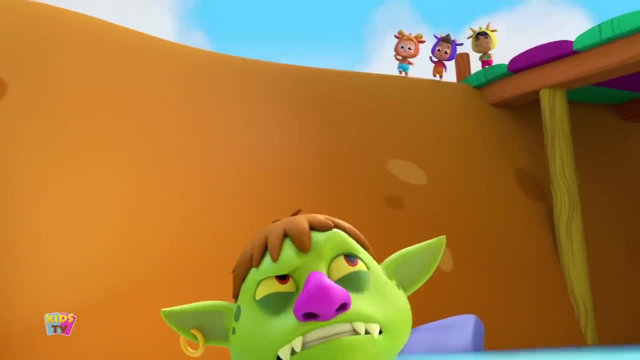 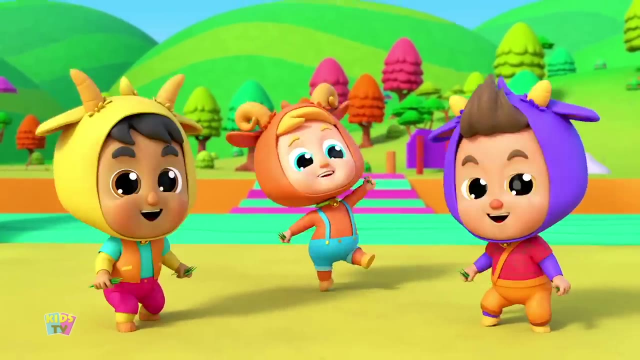 And sent him tumbling backwards over the bridge. Never to be seen again. Never to be seen again. So now I'll see my brothers too, And we'll eat until we're fat. We tricked that troll with a plan, you see, What do you think of that? 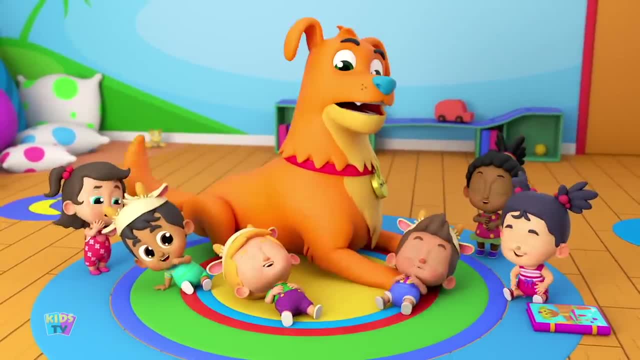 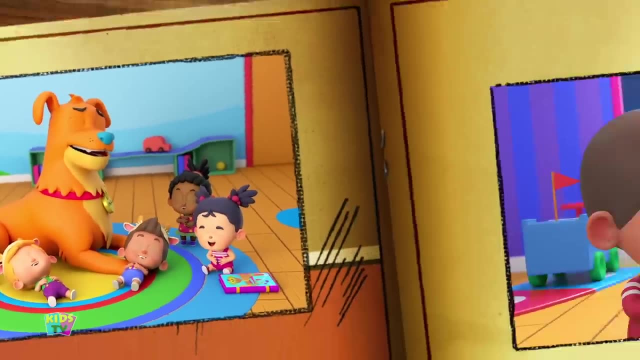 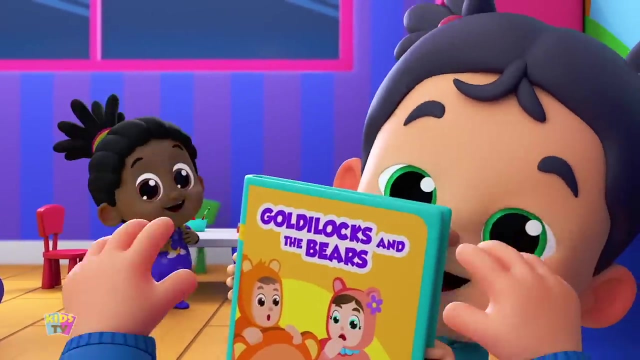 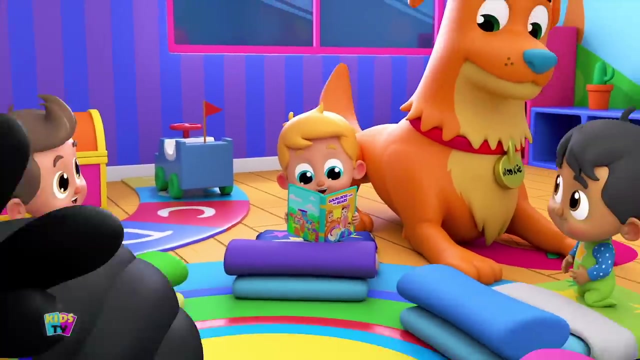 What do you think of that? I like it. Come on, Joey. Tell us the Goldilocks story. Tell us the Goldilocks story again. I want to play Goldilocks this time, Cause cause. Okay, that'll be funny. Out for a walk went Goldilocks. 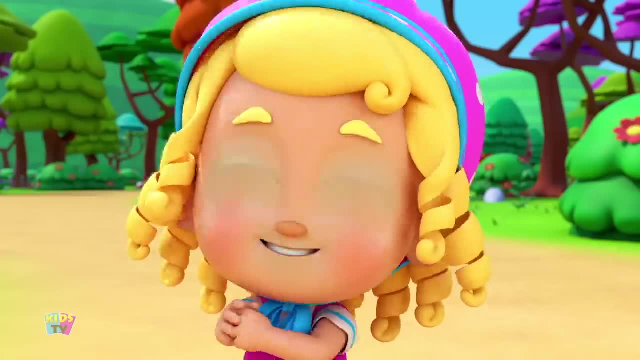 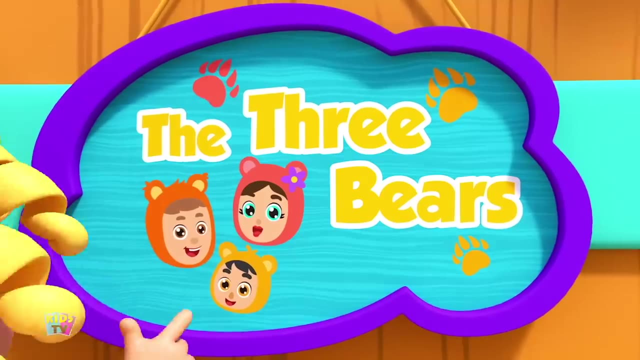 In the woods she saw a house. I'd like to go in and see what's there. I'll be quiet as a mouse. I'd like to go in and see what's there. I'll be quiet as a mouse. Oh, the three bears. Oh the three bears. 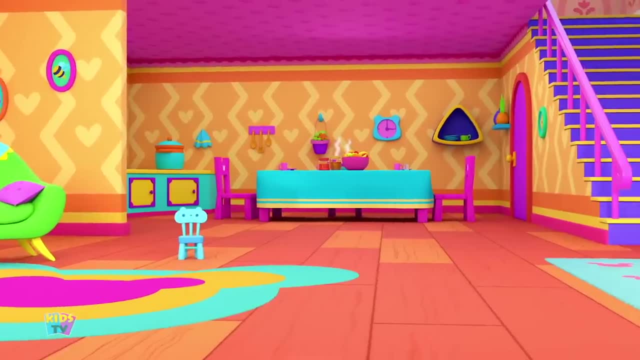 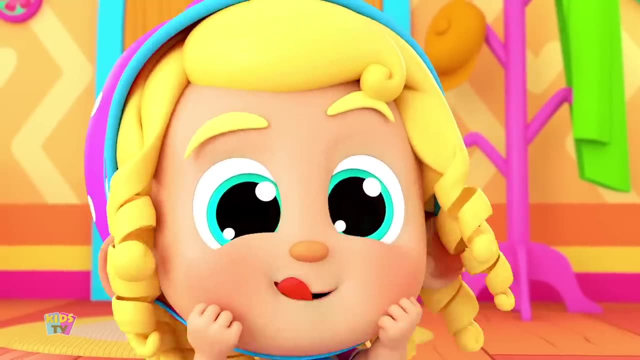 Right through the door went Goldilocks. And what did she first see? And what did she first see? A table full of scrummy food. A table full of scrummy food, Yum, Porridge, One, two, three, Oh, But the first one was too cold. 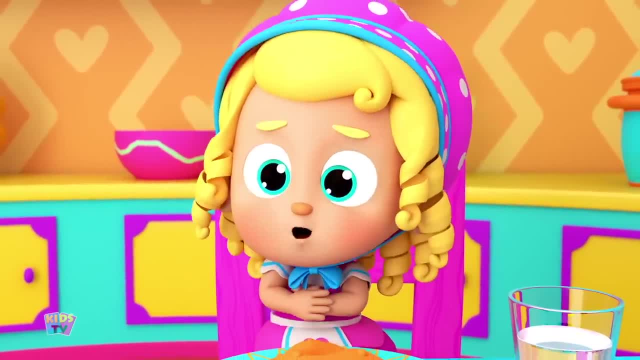 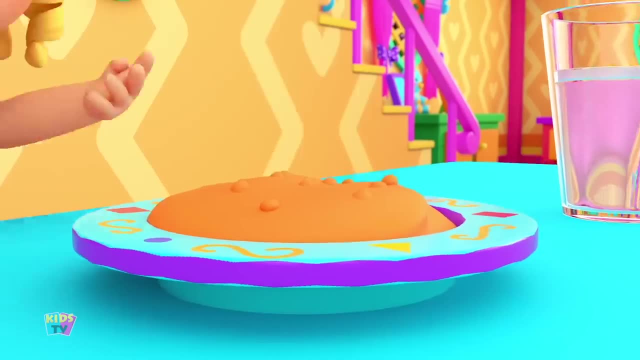 But the first one was too cold. But the first one was too cold And the second one was too hot, And the second one was too hot, But the third one was just right. But the third one was just right, And she ate it all in a shot, Yummy. 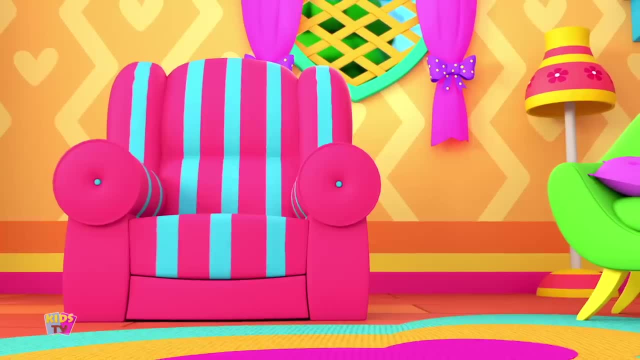 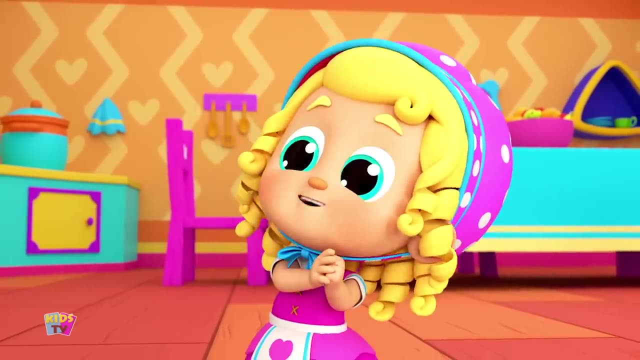 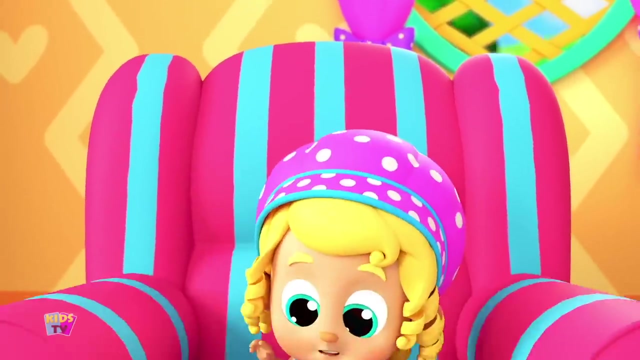 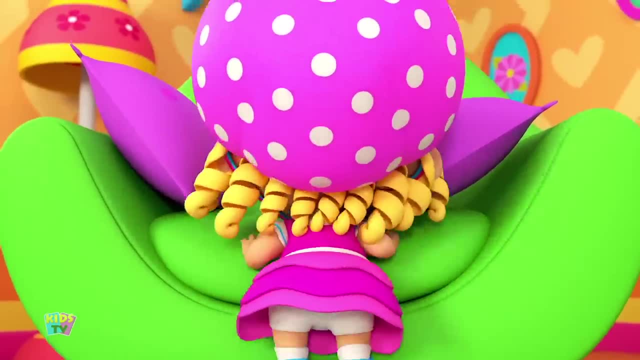 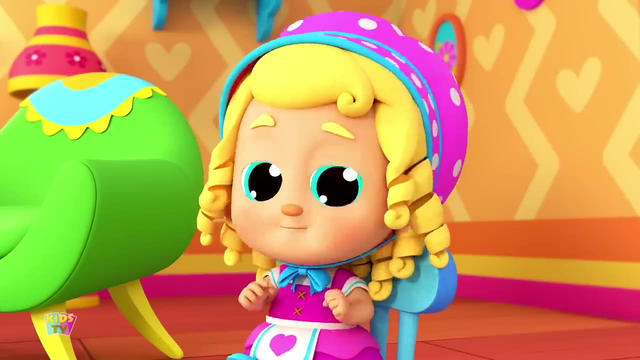 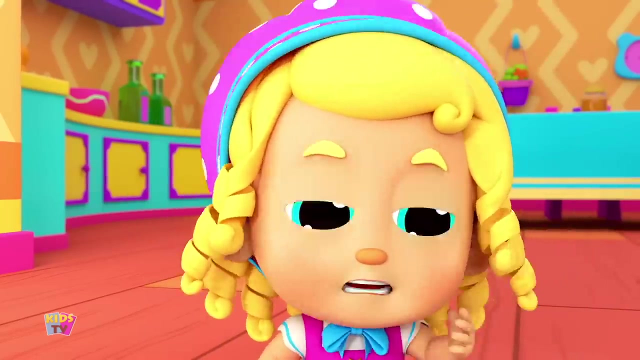 Oh my. And the second one was too small, Oh Too tight. But the third one was just right. But the third one was just right. This is the best of all. Oh Oopsie daisy. Oh my, When she plunked into the chair. 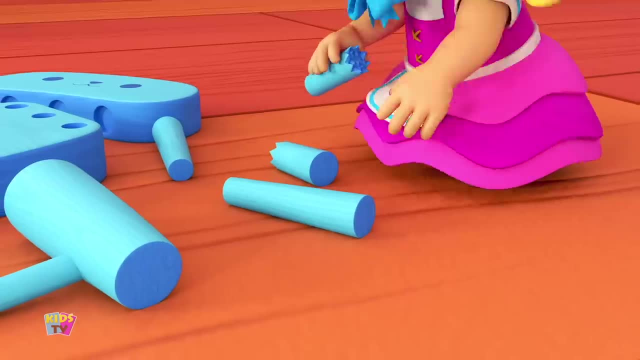 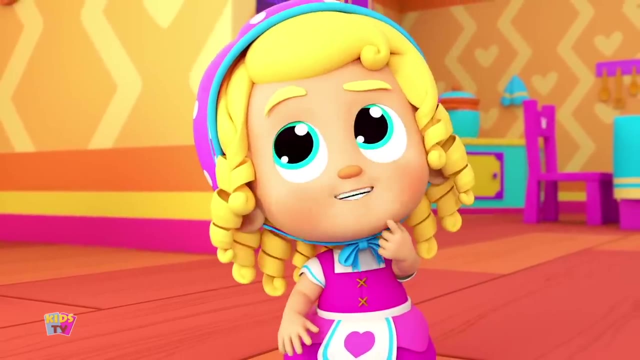 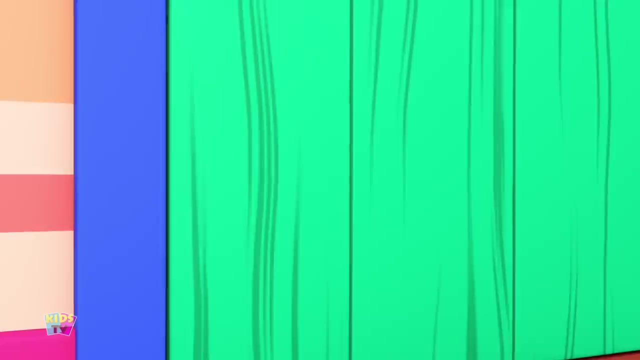 When she plunked into the chair, It broke into a million pieces. Oh my, Look what I did. Oh well, This adventure has made me so sleepy. This adventure has made me so sleepy. I think I need a nap. Goldilocks climbed the stairs. Goldilocks climbed the stairs. 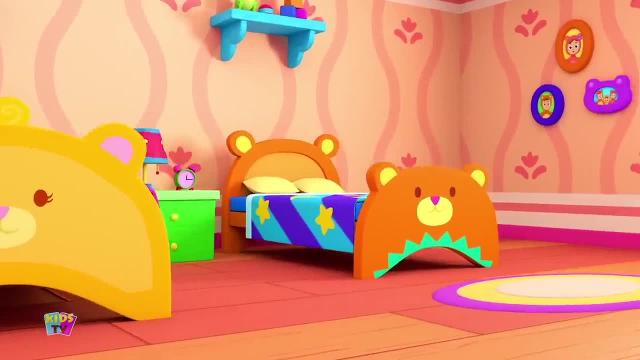 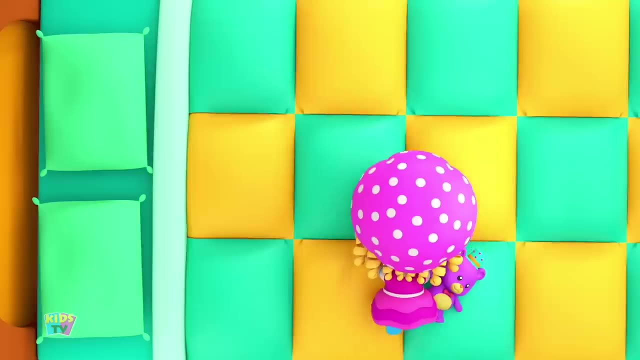 To a bedroom with three beds. Wow, Look at that. I think I'll rest my head. I think I'll rest my head. Don't mind if I do, Don't mind if I do, But the first bed was too lumpy. But the first bed was too lumpy. 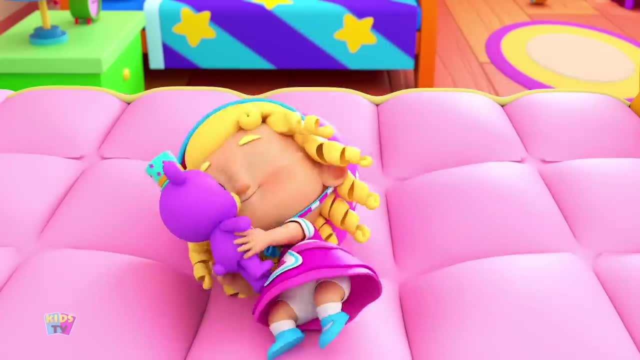 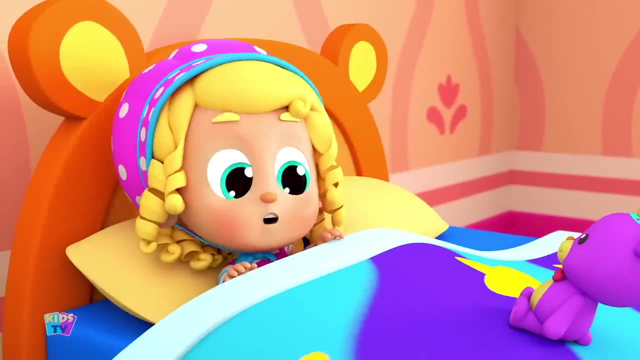 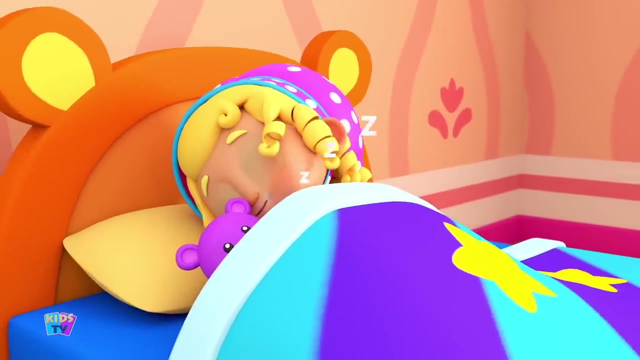 Ow, And the second one's squishy too, And the second one's squishy too. Oh no, But the third one was just right. But the third one was just right. Oh dear, Oh dear, While Goldilocks snored away. While Goldilocks snored away. 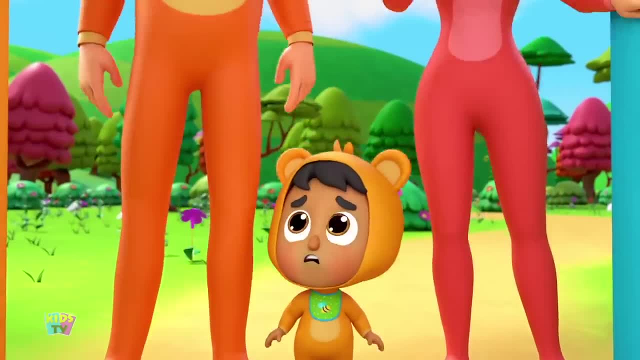 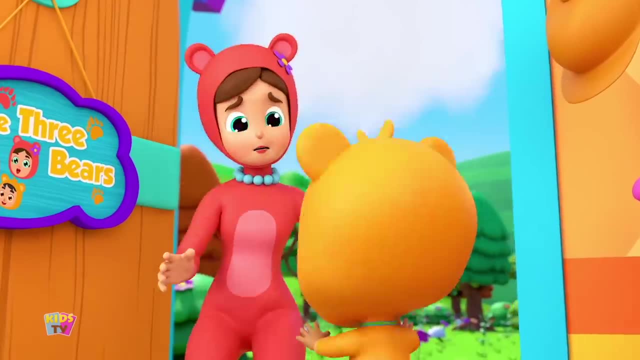 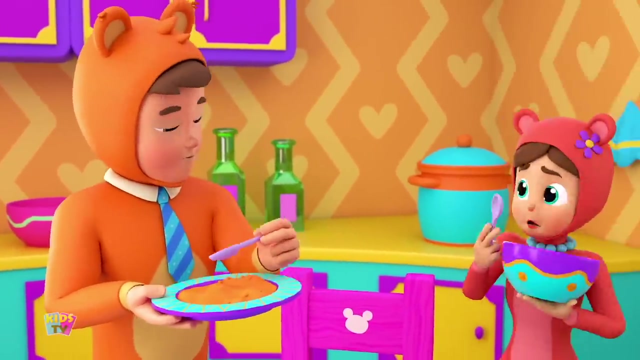 The three bears came back home. The three bears came back home. The front door was wide open. Oh dear, it looks like we're not alone. Oh dear, it looks like we're not alone. Oh my, Hmm, Someone's been eating my porridge. Someone's been eating mine too. 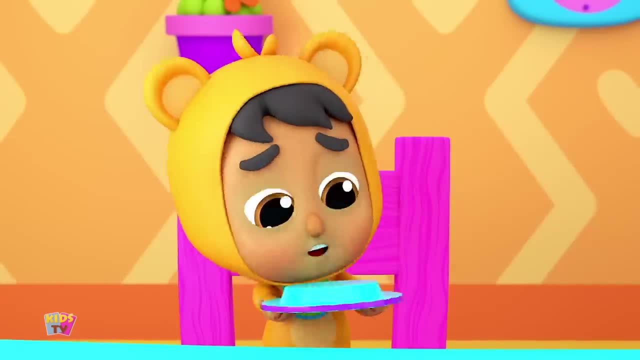 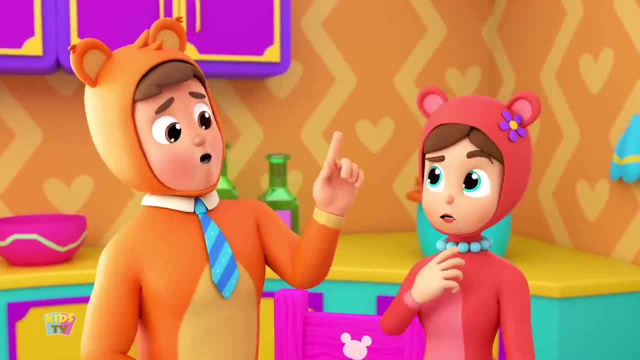 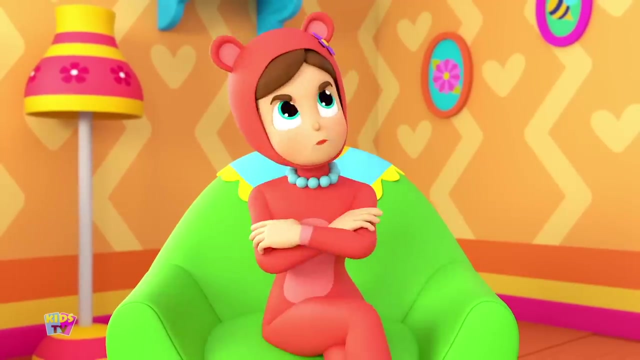 And somebody's finished my every drop. And somebody's finished my every drop. That was mine, thank you, That was mine. thank you, Oh dear. Hmm, Someone's been sitting in my chair. Someone's been sitting in my chair. Someone's been sitting here too. 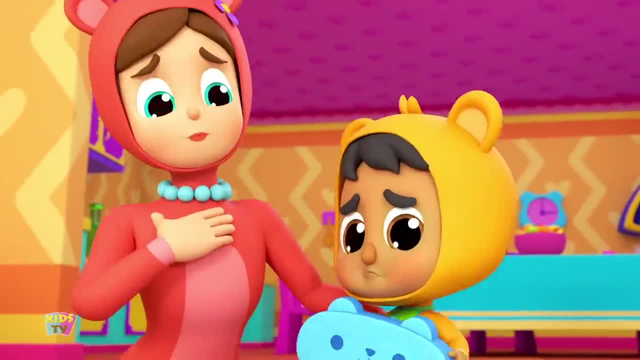 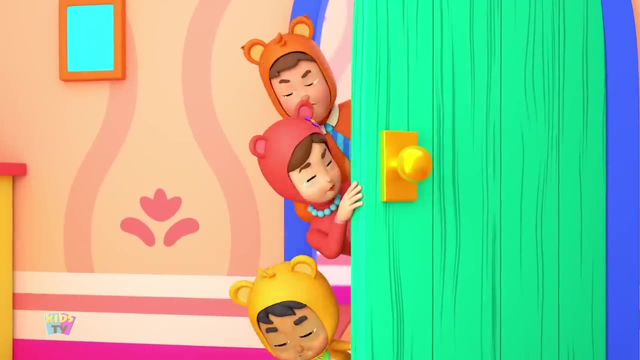 Uh-oh, guess what? My chair is broke, And that was good bamboo. I think I hear something upstairs. I think I hear something upstairs. Someone's been sleeping in my bed, And wouldn't you know it, mine too. And wouldn't you know it, mine too. 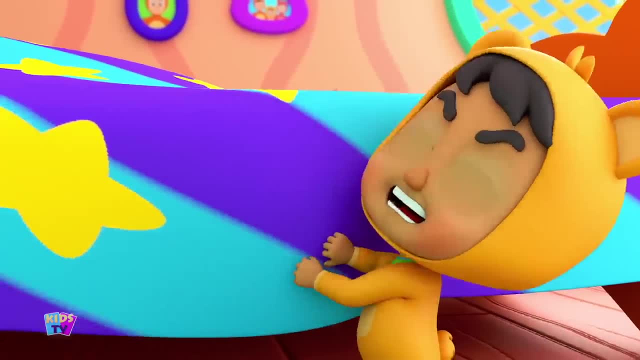 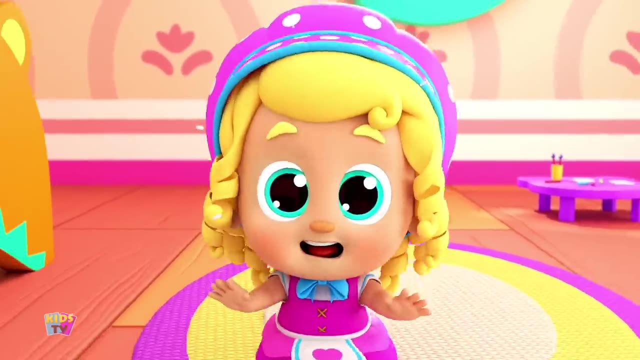 Someone's been. look, She's in my bed. Oh dear, who are you? Oh dear, who are you? Uh, bye-bye, Thanks for everything. Goldie raced into the woods. Goldie raced into the woods And hid from everyone. 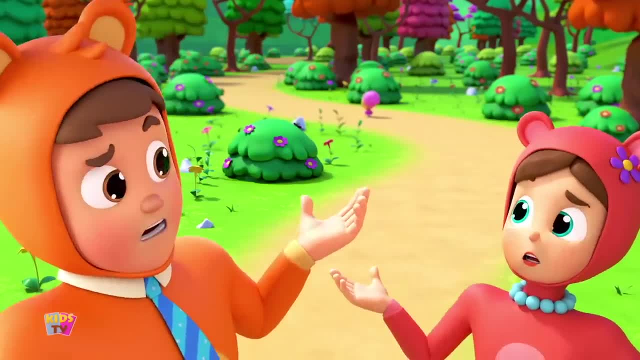 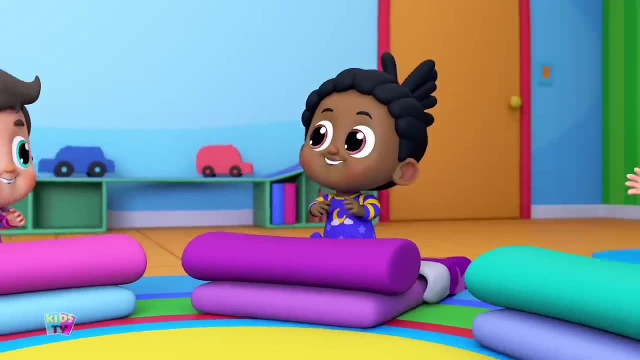 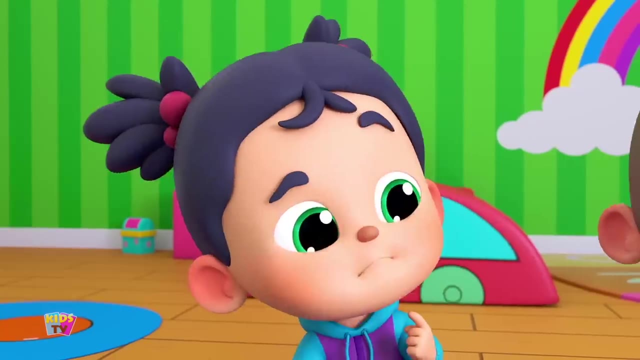 The bears could not believe their eyes. The bears could not believe their eyes. The bears could not believe their eyes. And now the story's done. And now the story's done. Did that really happen? Did that really happen? Just a fairy tale? Oh, but where are the fairies? 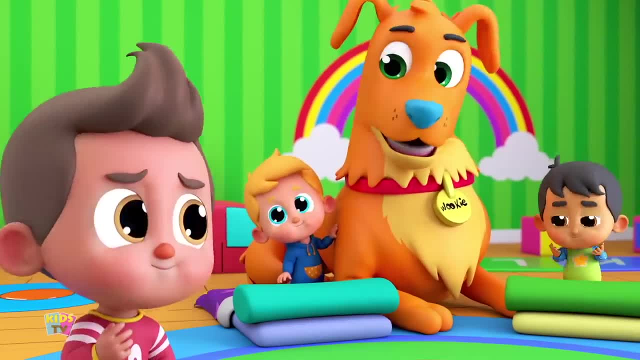 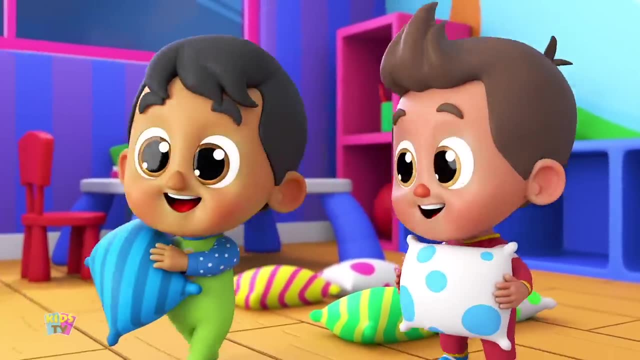 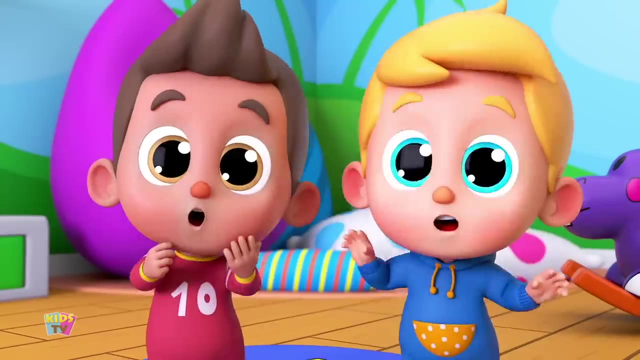 Oh, but where are the fairies? Funny Story time everyone. How about Little Red Riding Hood? How about Little Red Riding Hood? I want to pretend that I'm Little Red. I want to pretend that I'm Little Red And I'll be the Big Bad Wolf. 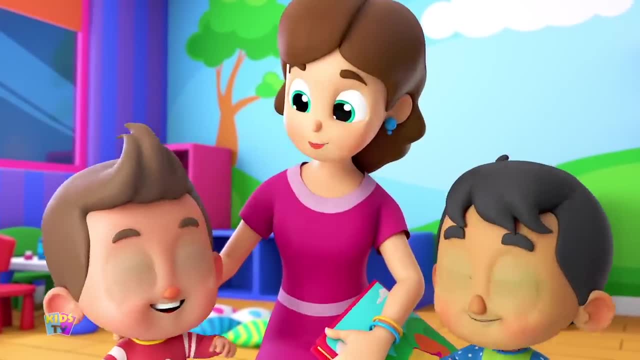 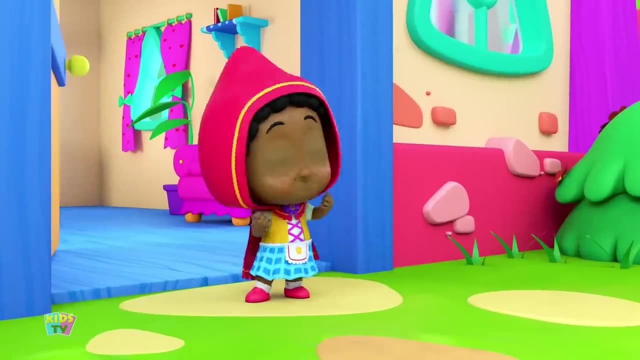 Oh, I'm not sure Wookiee likes that idea. Oh, I'm not sure Wookiee likes that idea. Everyone ready. There once was a girl all dressed in red. There once was a girl all dressed in red Who went to her grandma's sickly bed. 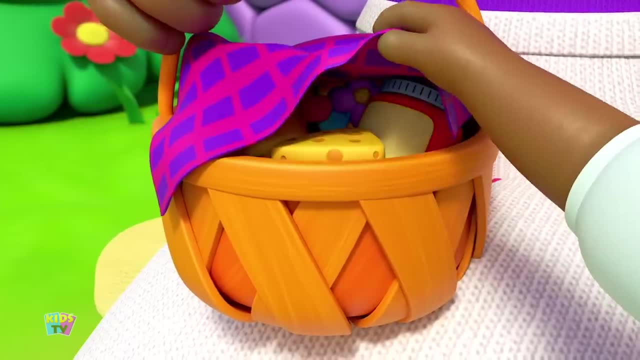 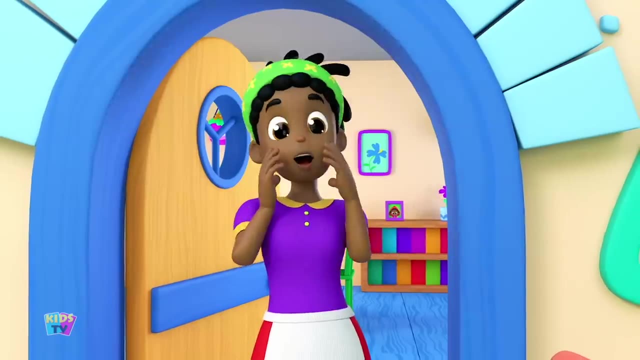 She's not feeling well, So I'll cut through the dell And visit Gran for a short little spell. And visit Gran for a short little spell. Now remember, don't talk to any strangers. Now, remember, don't talk to any strangers. I promise She gave Red some special teas. 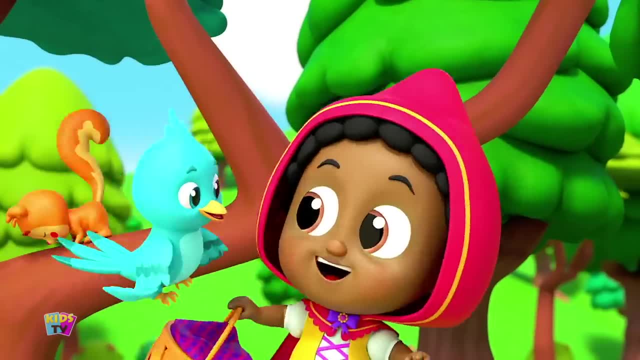 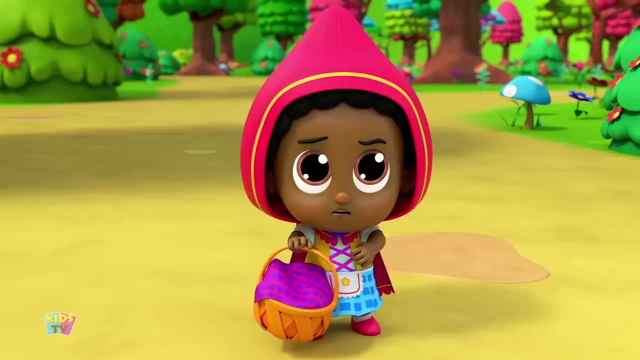 Grandma's very favorite cheese, Grandma's very favorite cheese. But in the woods a wolf stopped Red. But in the woods, a wolf stopped Red. Well, hello, my dear, you're going where. He said: um you're a stranger right. He said: um, you're a stranger right. 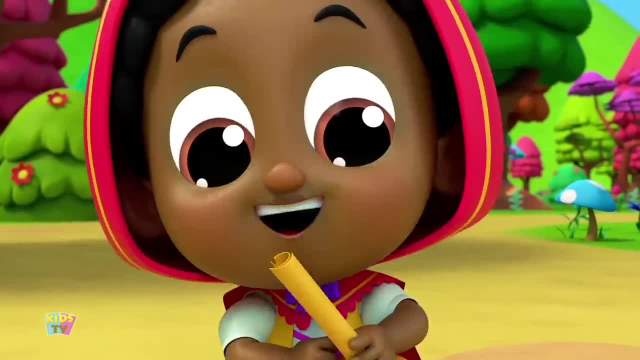 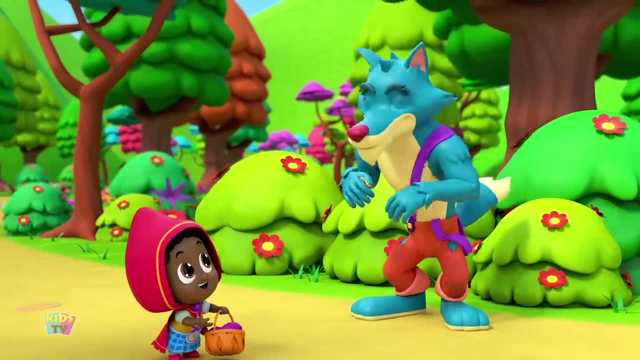 I'm not really supposed to talk to you, But I'm off to Gran. she's sick in bed. But I'm off to Gran, she's sick in bed. I've brought some cheese and fresh baked bread. Then Red took off. But the wolf was smart. 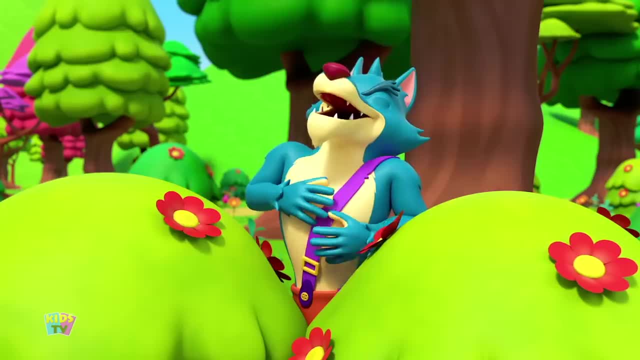 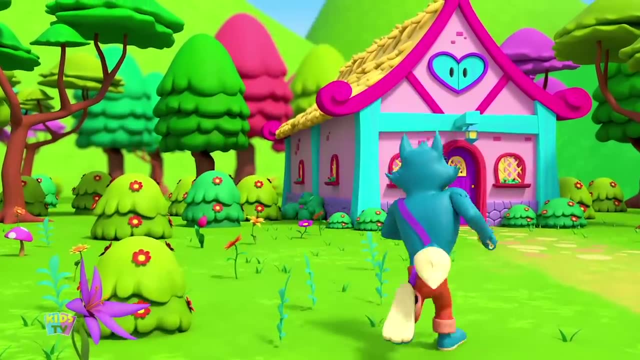 He knew the way to Gran. He knew the way to Gran. He knew the way to Gran. The wolf sneaked into Gran's place. The wolf sneaked into Gran's place. I'll hide you, so there's not a trace. I'll hide you, so there's not a trace. 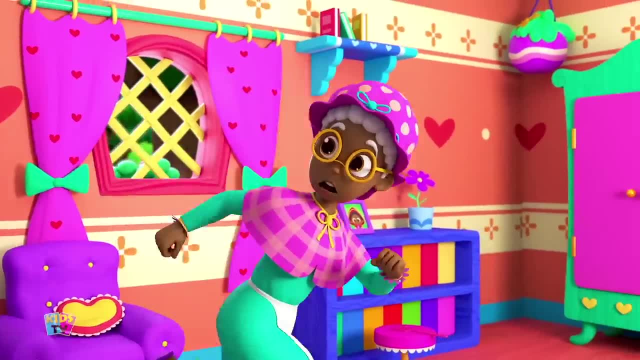 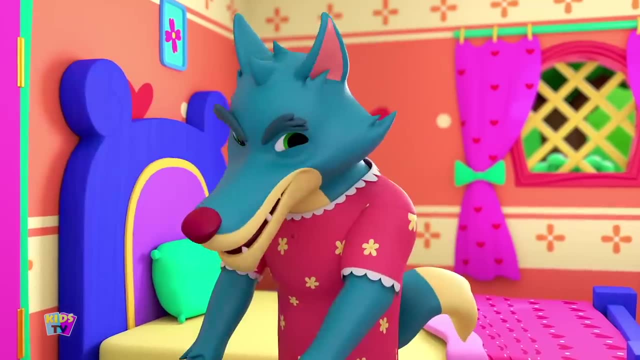 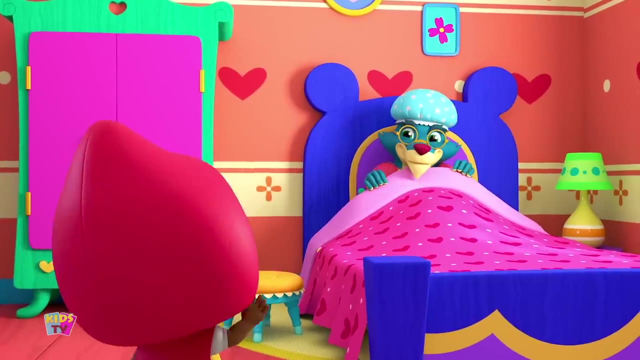 He locked her in, got into bed. He locked her in, got into bed With Granny's nightcap on his head. With Granny's nightcap on his head, Help me, Poor Granny cried. Why come in dear, Why? Gran Said Red and she walked right in. 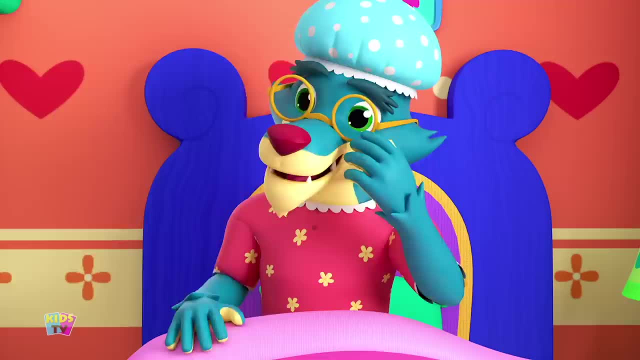 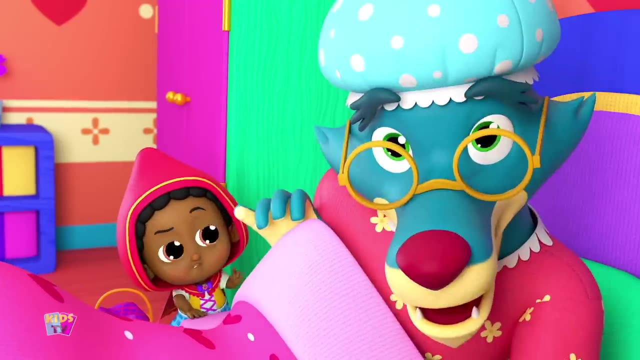 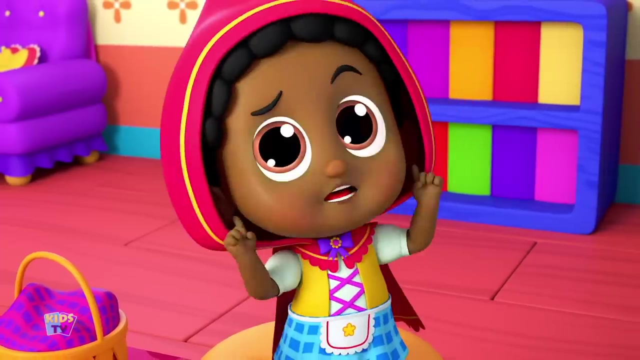 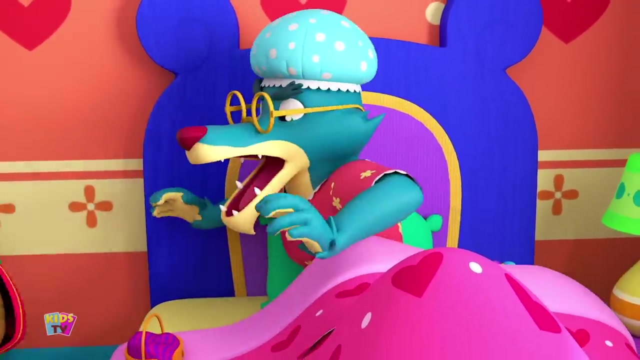 I've been wondering how you've been. I'm okay, But she sounded weird, Granny, since when do you have a beard? Granny has a beard, Uh-oh, Why? Granny, what big ears you have. And, Granny, what big eyes you have. And, Granny, what big teeth you have. 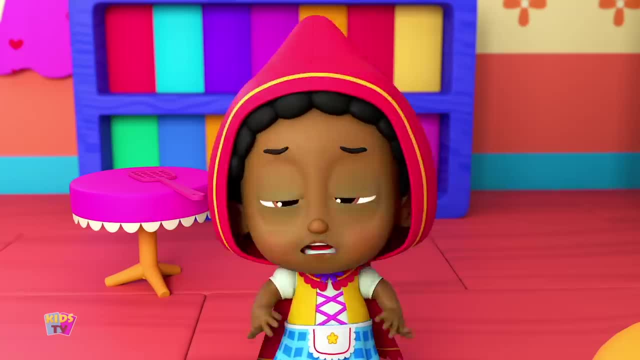 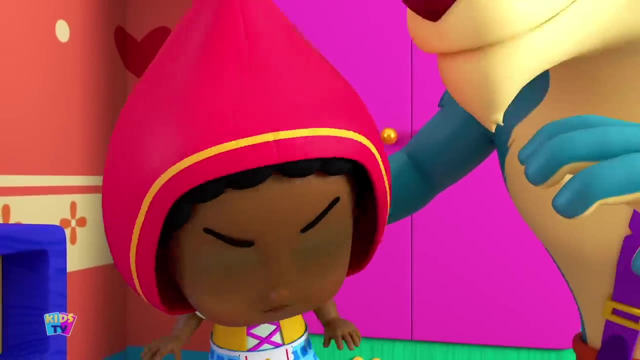 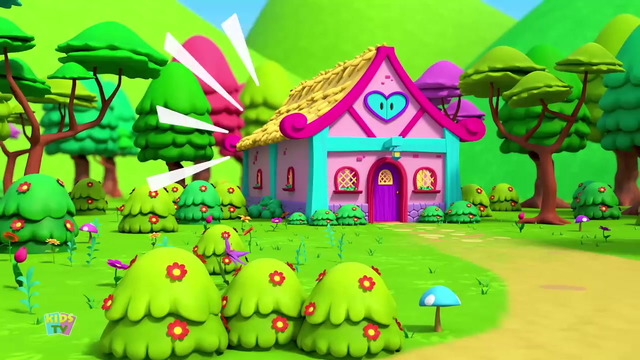 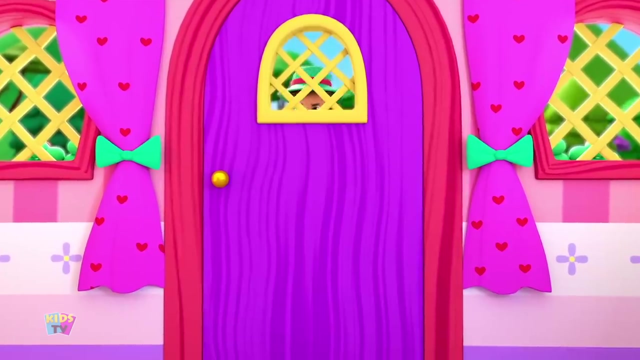 The better, my dear, to eat you is. No, no, no, Say that to my face. The better to eat you is On second thought, no, no, Cried Little Red Riding Hood, And a huntsman burst in from the woods. He broke the door and he grabbed that beast. 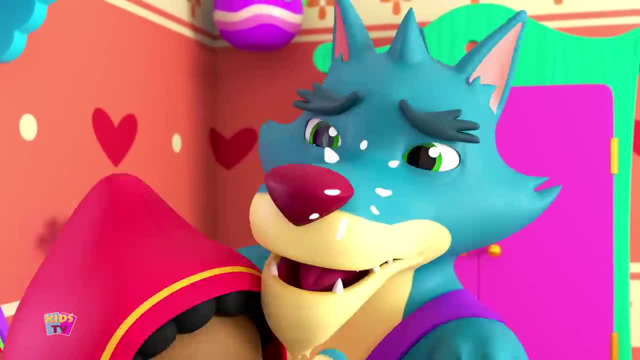 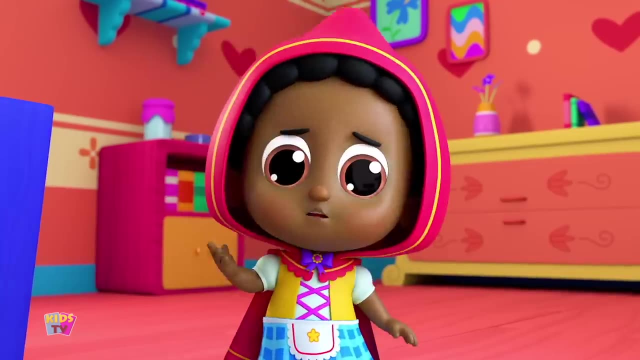 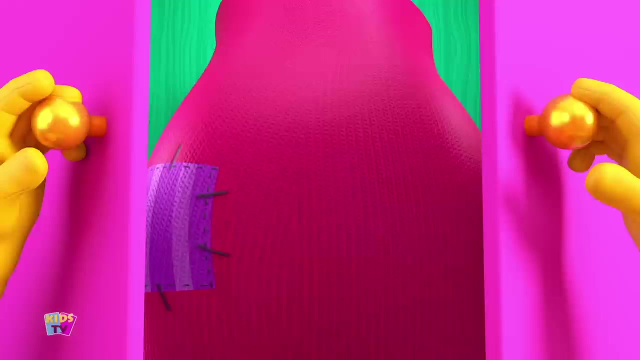 Why I'll give you a pow, To say the least. You're a big, bad, hairy wolf. And you're a big, bad, hairy wolf And you better stop being a bully Or you won't have any friends. Well, the huntsman, let poor Granny out. 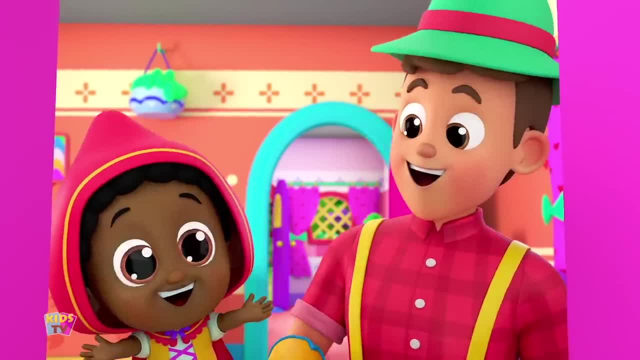 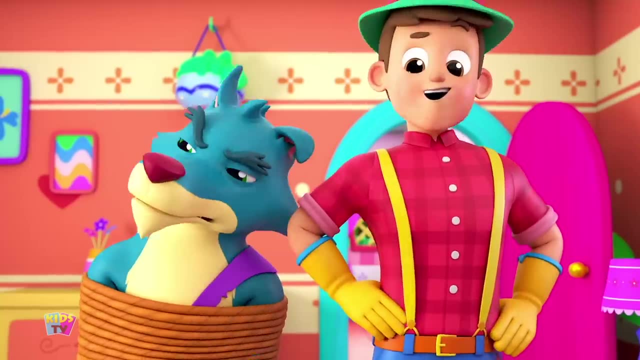 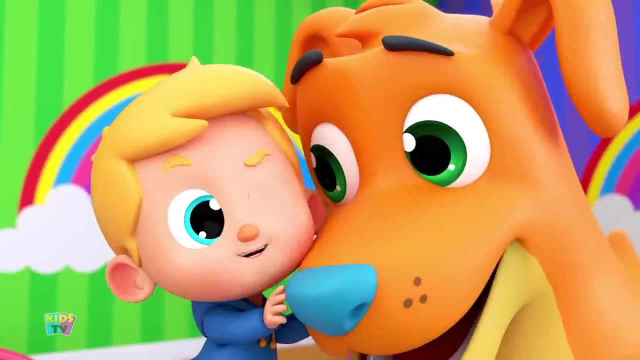 And Little Red just blurted out. I talked to a stranger, Confessed: Little Red, I've learned my lesson now. She said She learned her lesson now. she said: Wow, that big bad wolf sure learned his lesson. Huh, He sure did. And I sent him away. 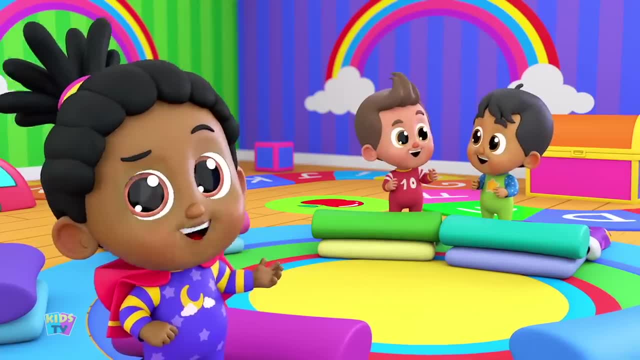 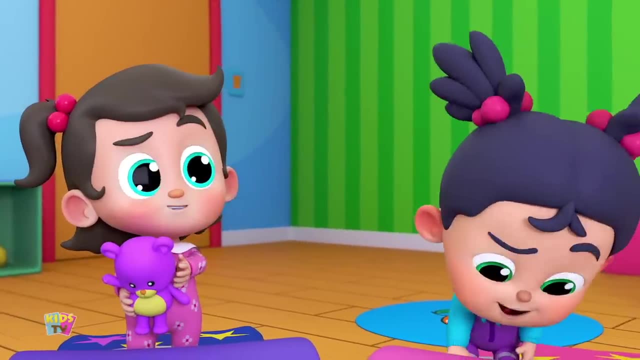 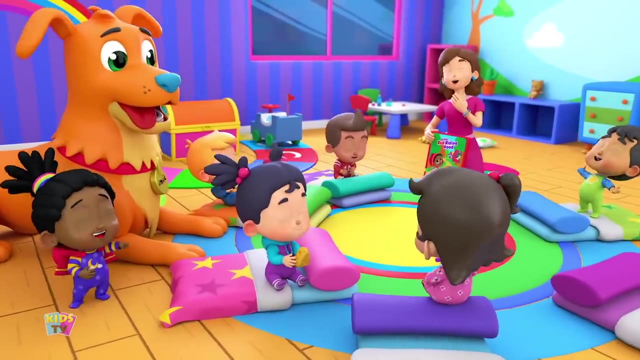 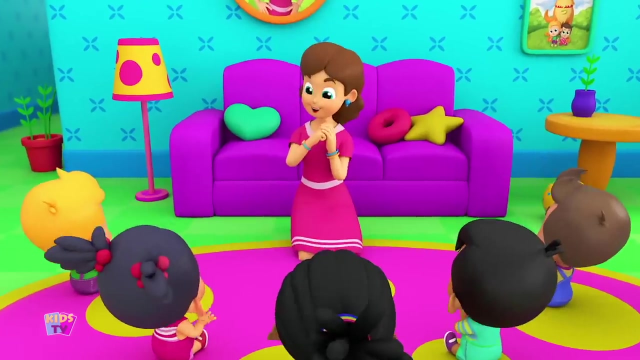 And he never came back. See what happens to big bad bullies Indeed. Now what's the moral of the story? Never let a wolf know if you have Fresh-baked bread and special cheese. Okay, whose turn is it to tell a story? 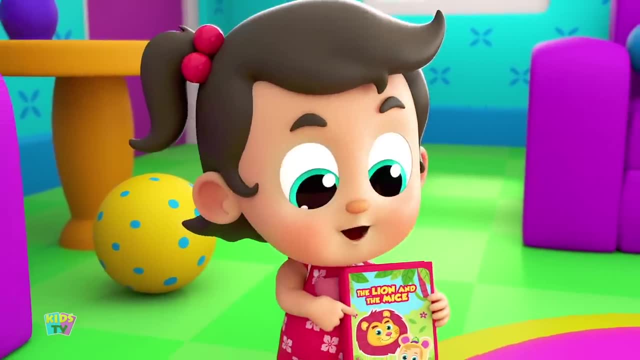 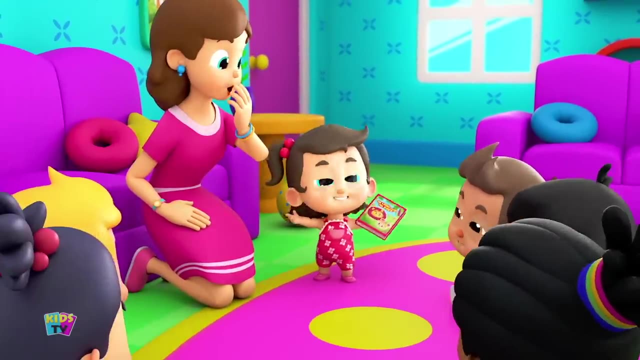 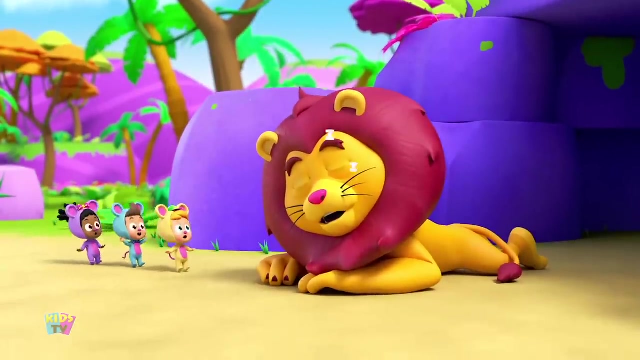 It's my turn and I'm going to tell the story of the lion and the mice. Don't you mean mouse? Not this time, because you're all going to be the little mice. A mighty, mighty lion lay sleeping in his lair. Three little mice came creeping by and stared. 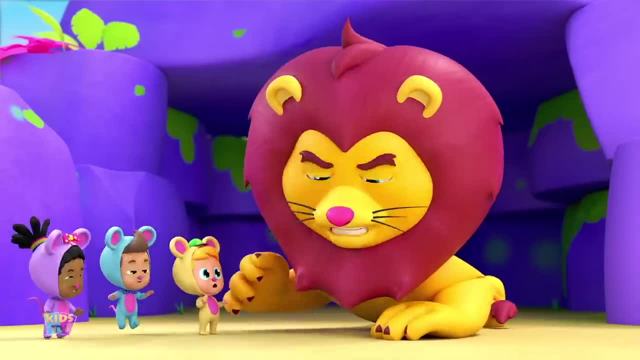 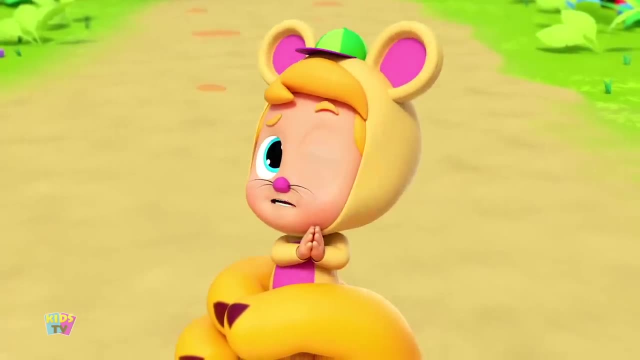 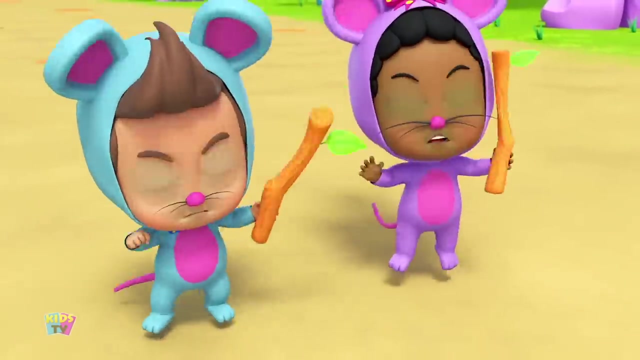 One accidentally brushed up against the lion's paw. Yikes, sorry, Mr Lion. There ought to be a law. Oh sorry, I hope I didn't hurt you. The lion drew his paw back and dropped it on the moose. The other mice were frightened and squealed. 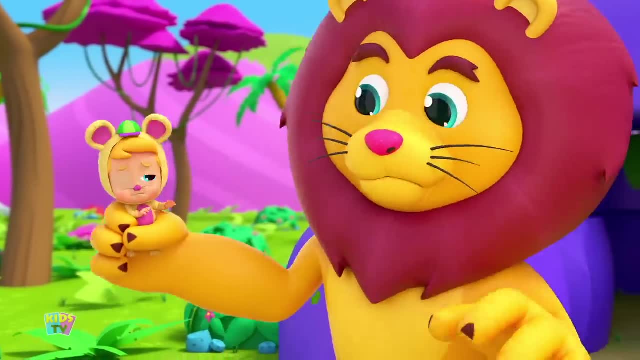 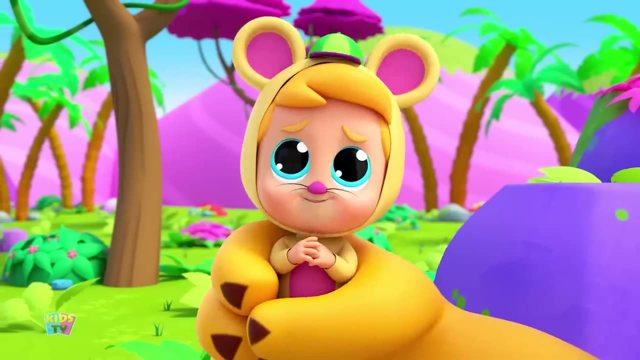 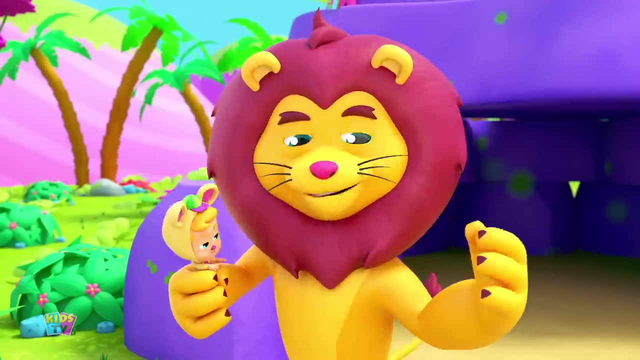 You louse. I beg you, Mr Lion, kindly hear my plea. I promise to repay you if you'll only set me free. Oh, please, I'll be your best friend. Well, I guess I could say yes, But only just a little bit. 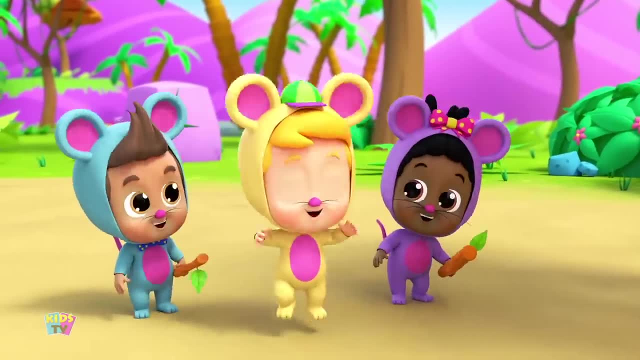 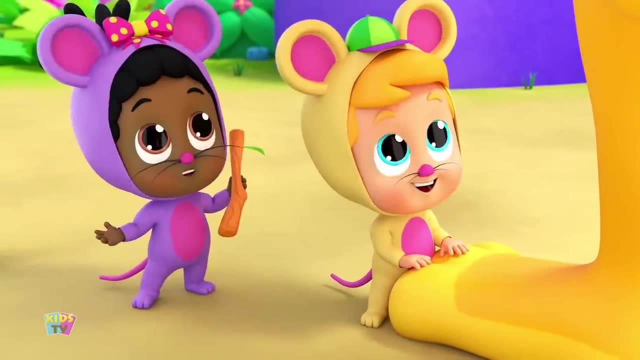 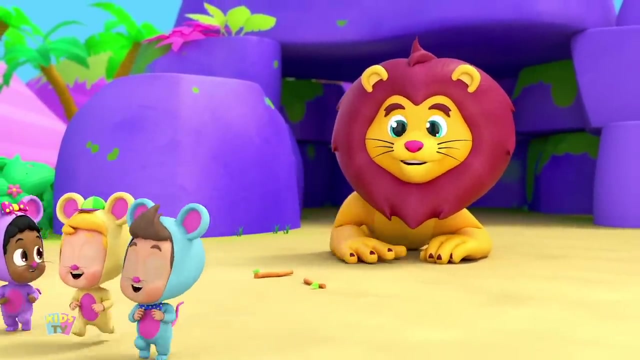 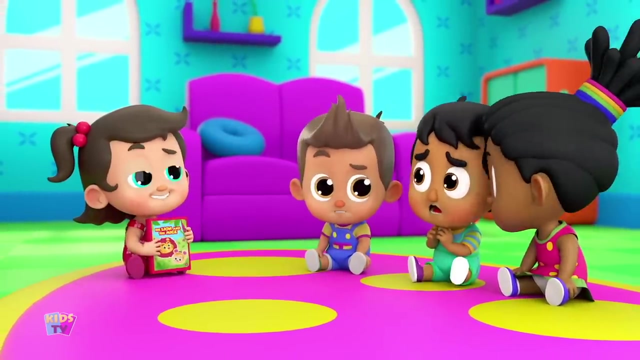 Just this time. Now, scatter with your friends and I'll pay you no mind. Oh, thank you, Mr Lion, I'm forever in your debt. I guess not every lion is really such a threat. Ah, Go away, You're swell. So the great big lion, let the little mouse go. 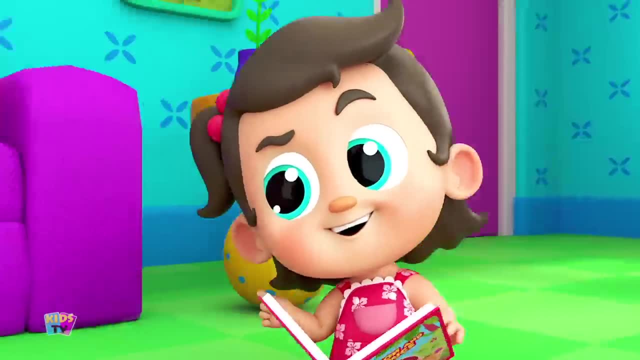 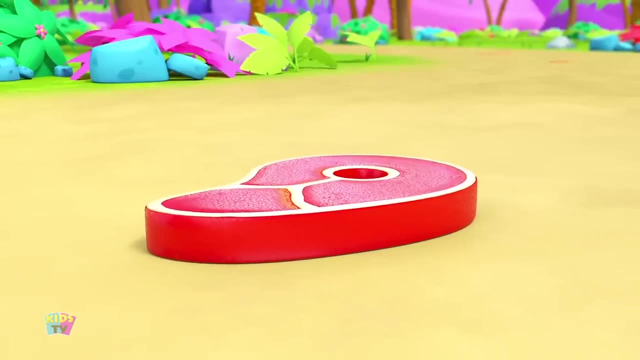 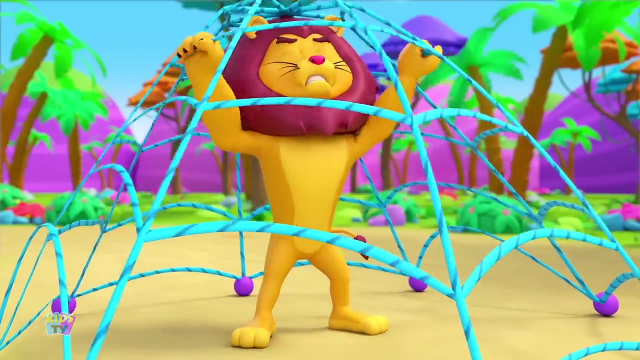 Phew, that was scary, But that wasn't the end of the story. Whoa, Oh, do tell Mr Lion. Yeah, go on. Well, the lion went a-hunting and wound up in a net. He paced and paced and growled and then began to fret. 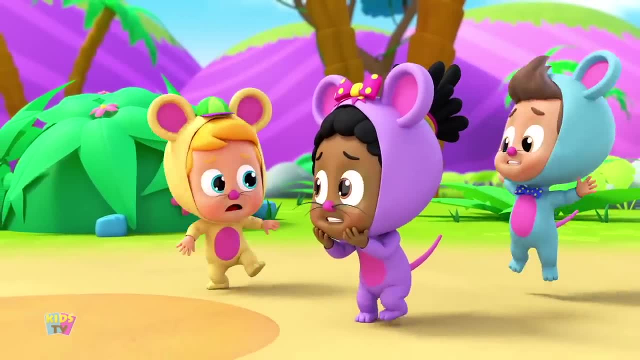 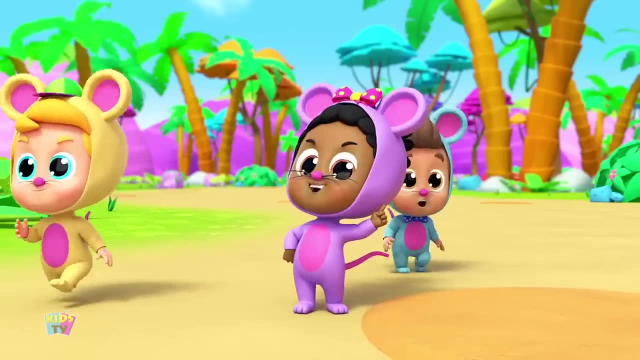 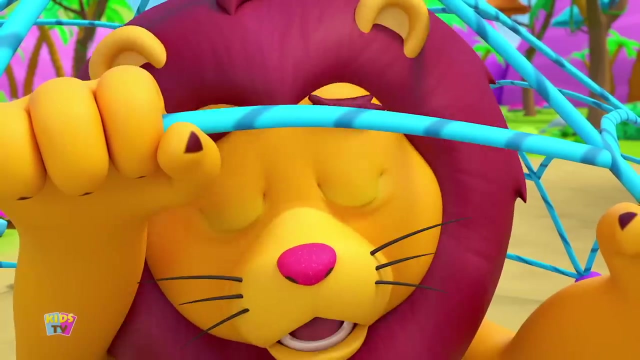 He roared so very loud that the three mice heard his cry. Is that your friend the lion? He's in trouble me. oh my, Hold on to your horses, I mean lions. We're coming to the rescue. Captured in the net, the lion paced and cried. 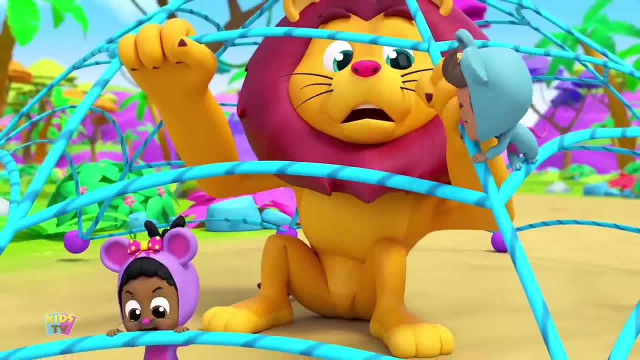 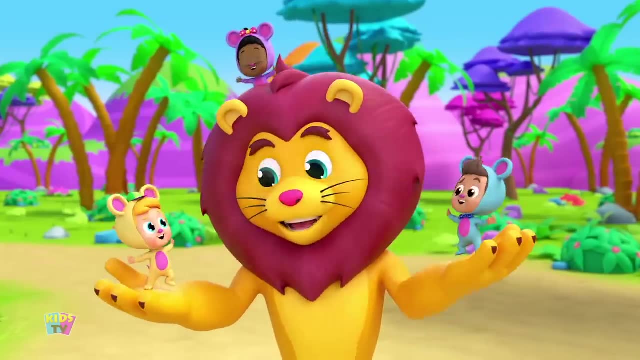 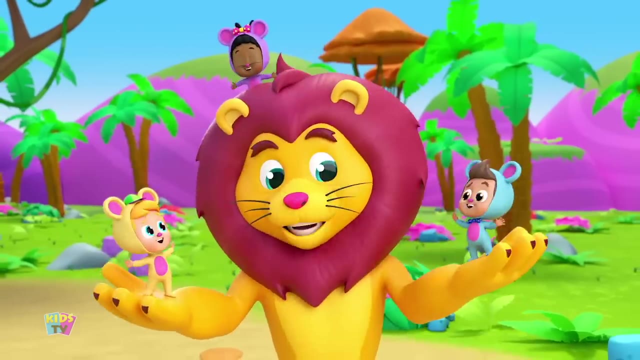 Unafraid, the little mice clambered to his side. They nibbled a big hole and became the lion's guide. Well, what do you know, these little mice have now become my pride. They're friends, Friends to the end. Nice Mousy. 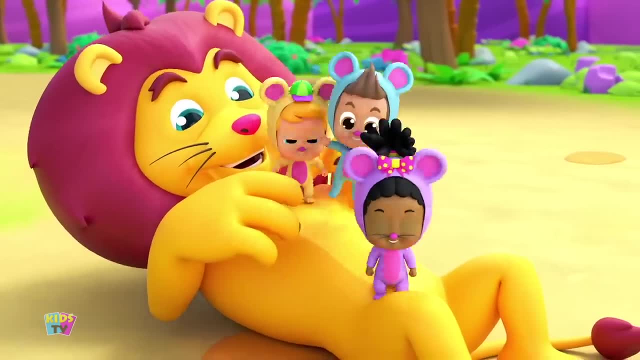 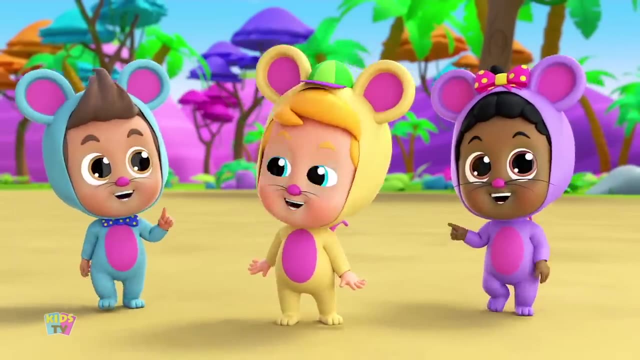 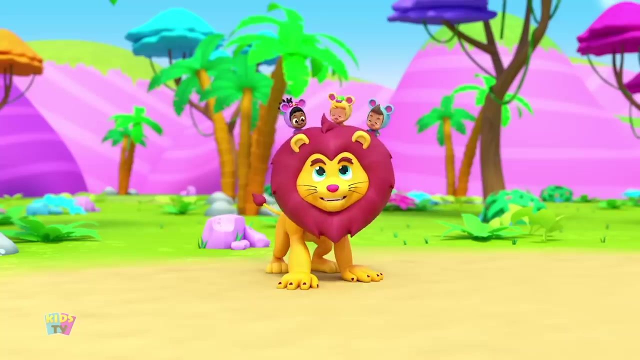 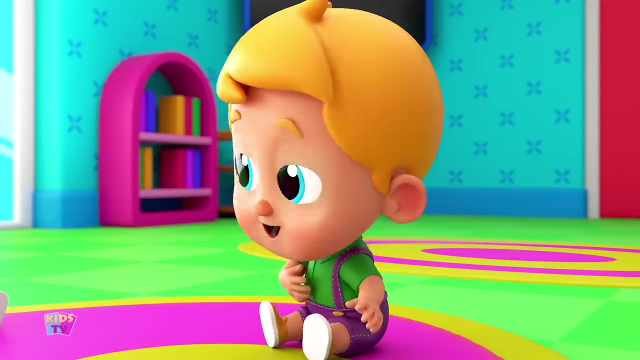 Friends are just like family, and family just like friends. I always keep my promises, Promises on that you can depend. The lesson here is friendship, Mr Lion. see, Friendship is a gift that always sets you free, So so is this a story about lions that get trapped? 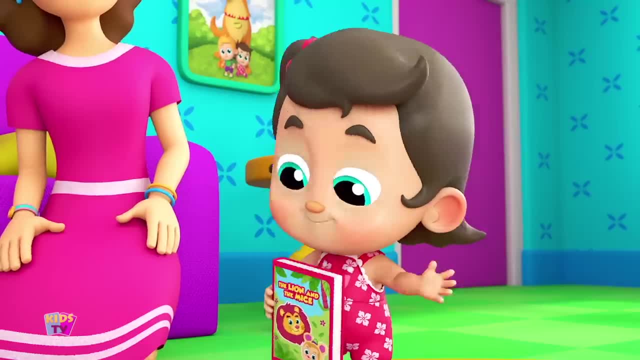 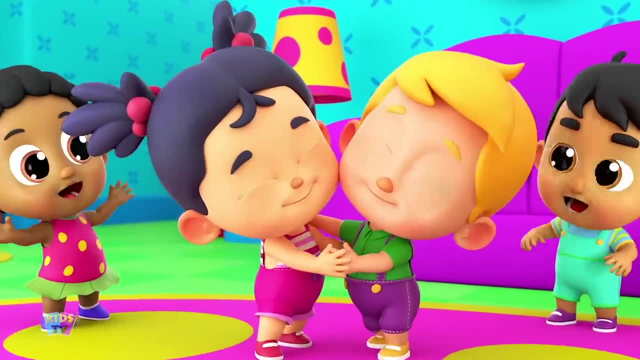 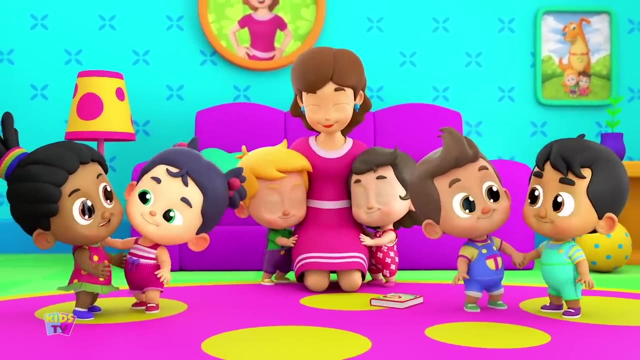 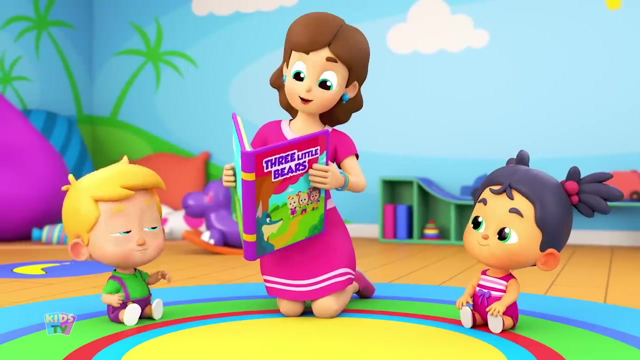 No, silly, it's about friendship and kindness, It sure is. It's about always being there for your friends. Yay, I like that. That's sweet Once upon a time. No wait, Okay, do you want to tell the story? 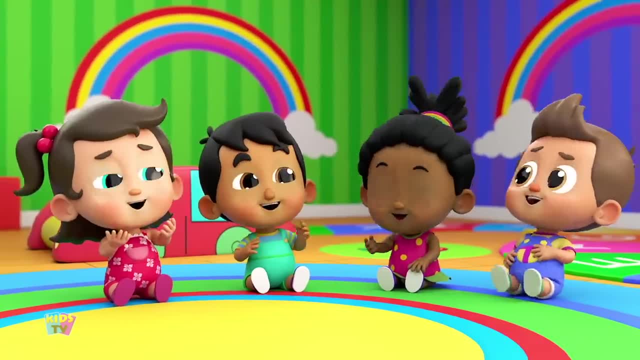 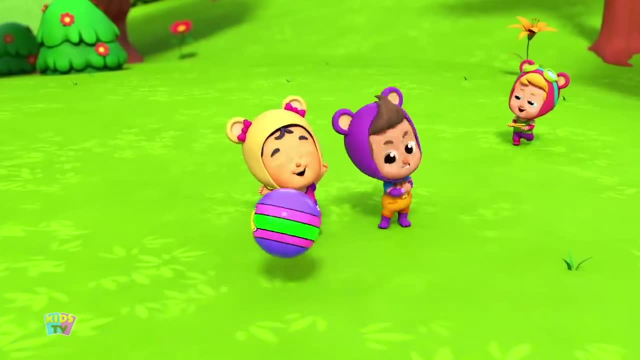 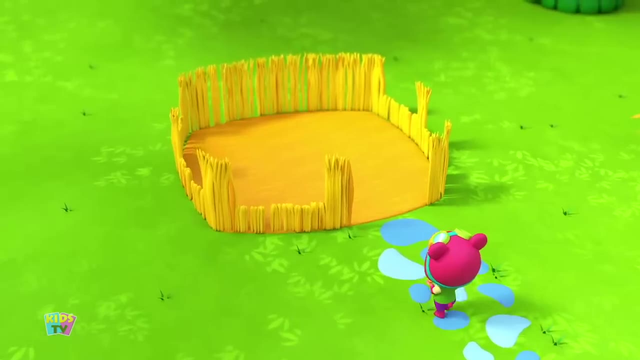 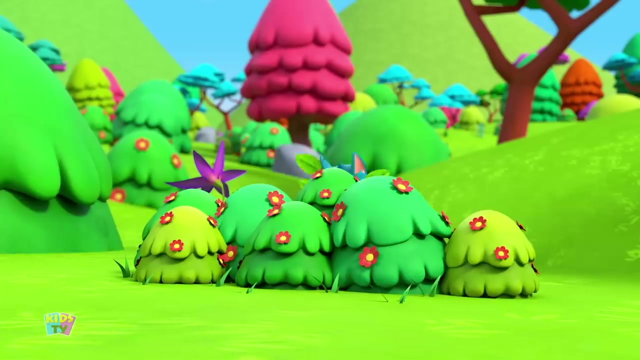 No, I just like saying that Once upon a time Three little bears went out to play. I'll build a house of straw today, Said one little bear, and just like that He built that house. and then he took a nap. But a mean old wolf woke him up. 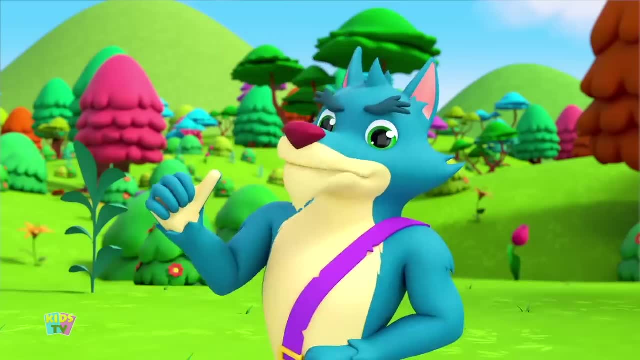 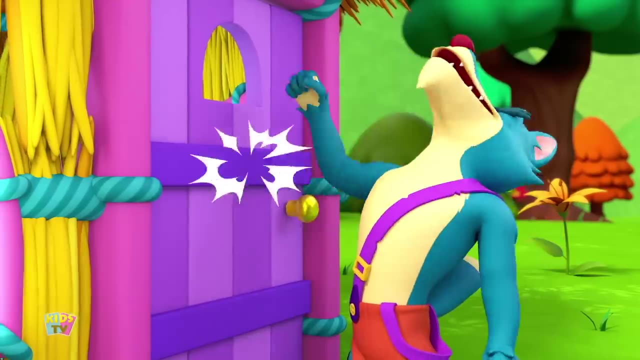 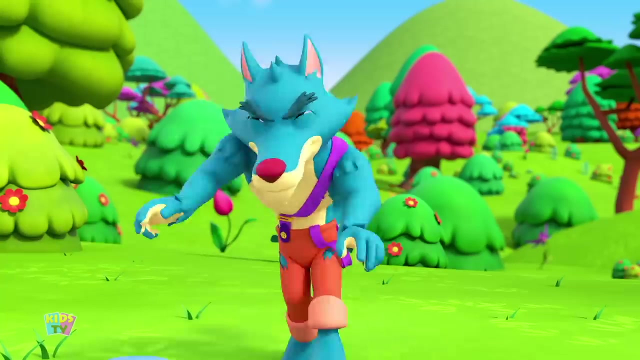 Oh no, I'm a big bad wolf and I see you in there. Open the door, little bear, beware. Ow, He pounded the door. Let me come in, Not by the hairs of my berry chin-chin, Then I'll huff and I'll puff and I'll blow your house in. 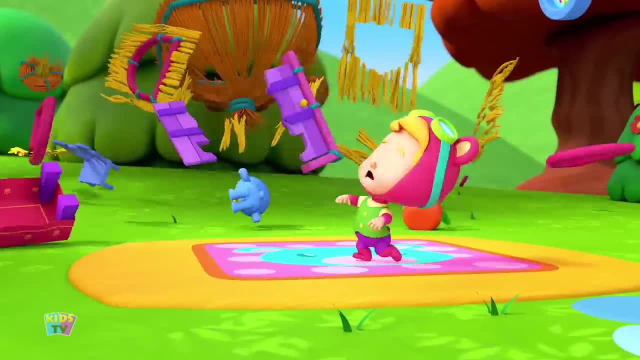 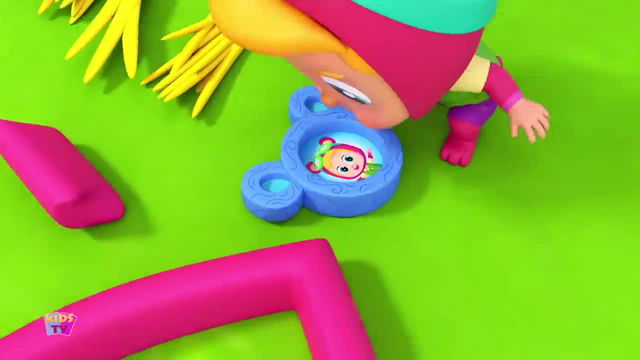 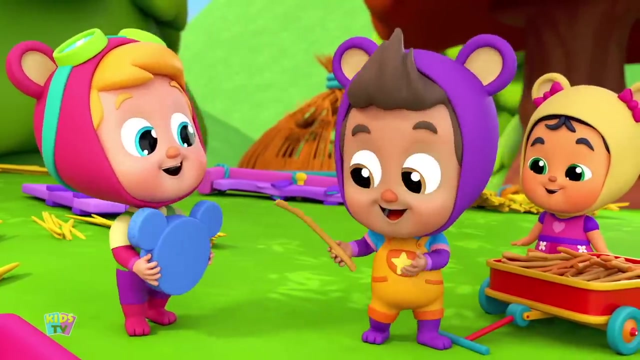 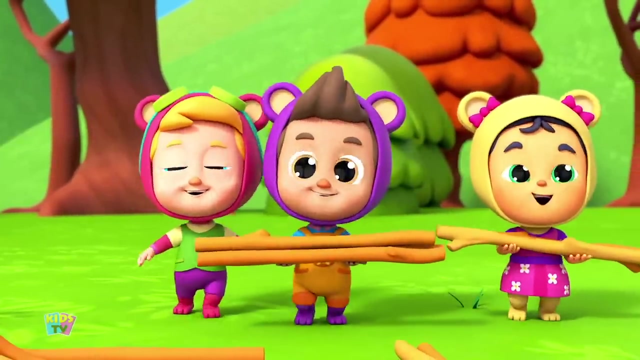 And he did. and he laughed with the worst laugh there's ever been. Oh no, Maybe I should have used twigs instead of straw. Out to play went two little bears. My house will be made of twigs. see there, Said the second little bear. and just like that. 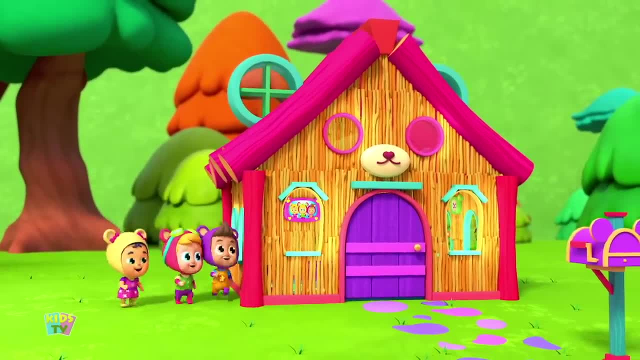 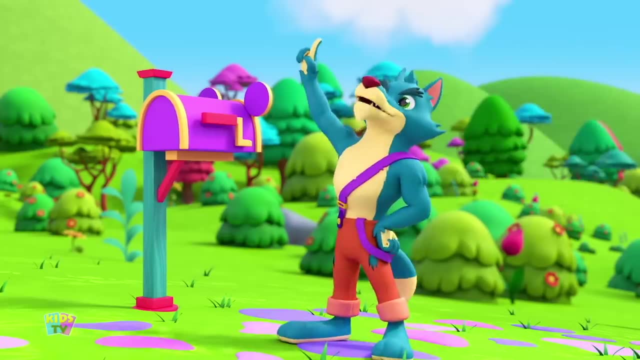 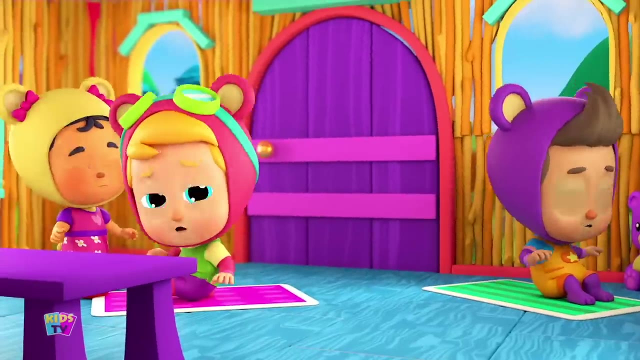 He built that house and then he took a nap. But once again that mean old wolf woke him up. I'm a big, bad wolf and I see you there. Open the door, little bear beware. Oh dang, He pounded the door, Let me come in. 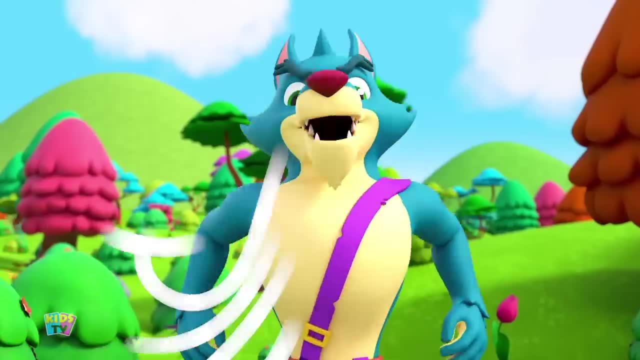 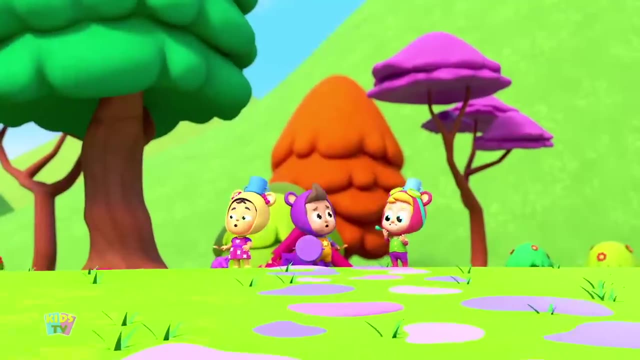 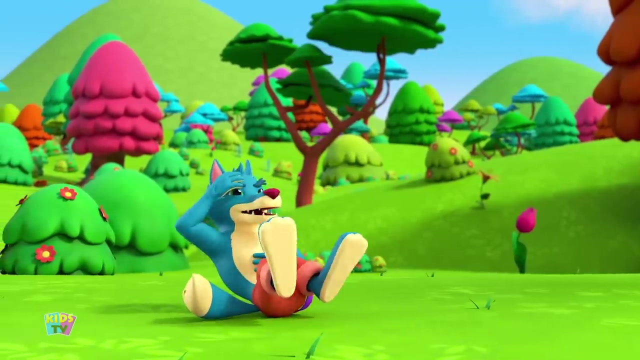 Not by the hairs of my berry chin-chin. Then I'll huff and I'll puff and I'll blow your house in. And he did, and he laughed with the worst laugh there's ever been. Oh, no, Oh, I guess we're gonna have to build something. 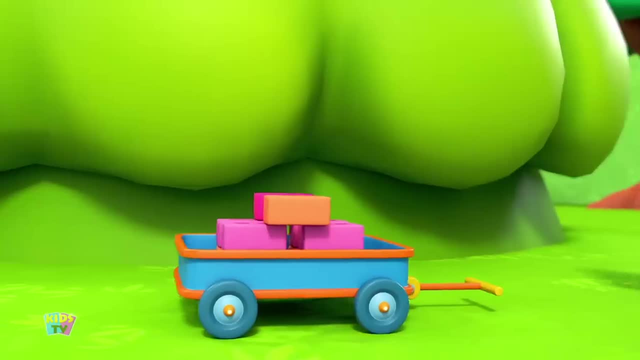 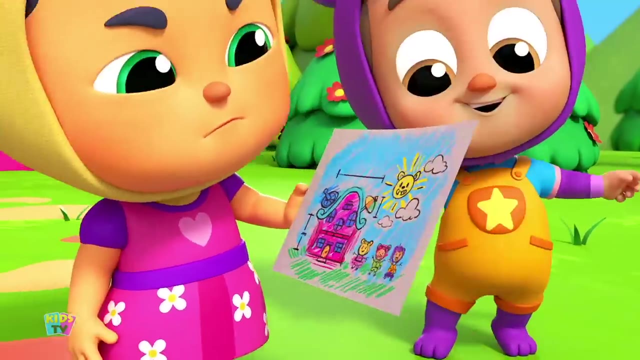 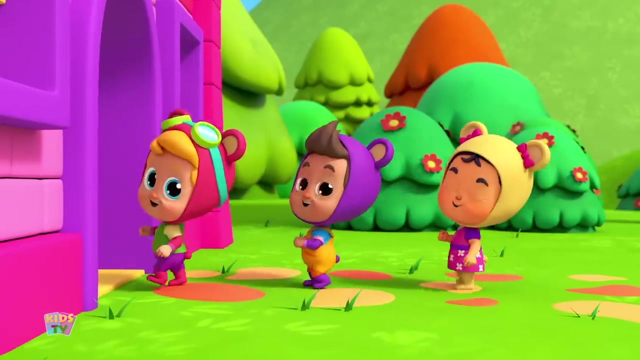 That that mean old wolf can't blow down Just one little bear. and she had to think: quick, I'll make my house out of sturdy bricks, Said the third little bear. and just like that She built that house. and then she took a nap. And can you believe it? 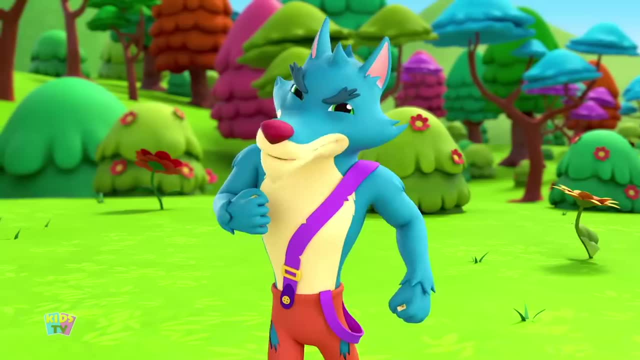 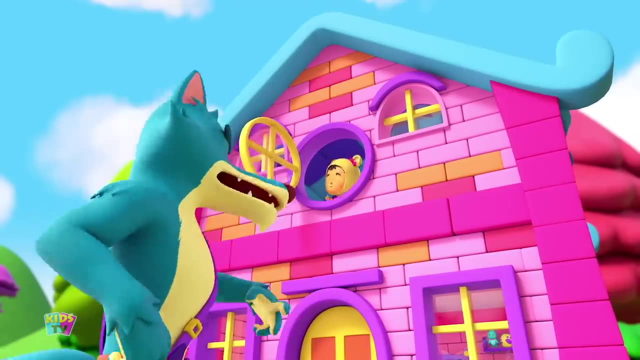 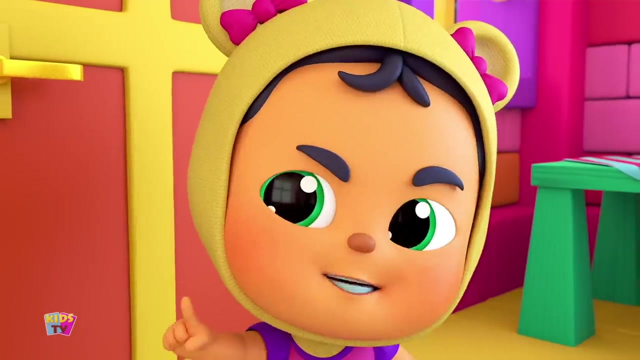 That nasty old wolf woke her up. I'm a big bad wolf and I see you in there. Open the door, little bear beware. No, Oh, He pounded the door. Let me come in, Not by the hairs of his berry chin-chin. 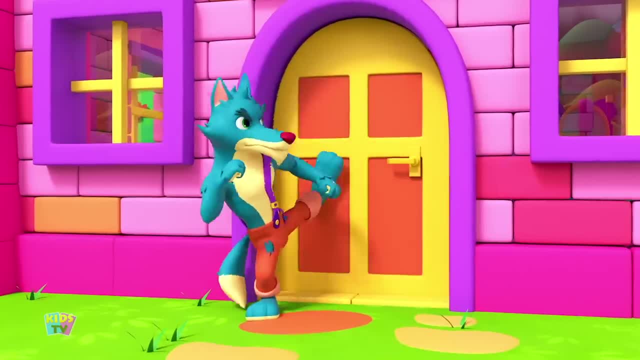 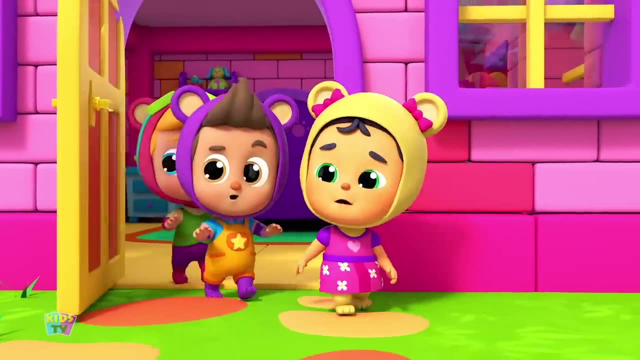 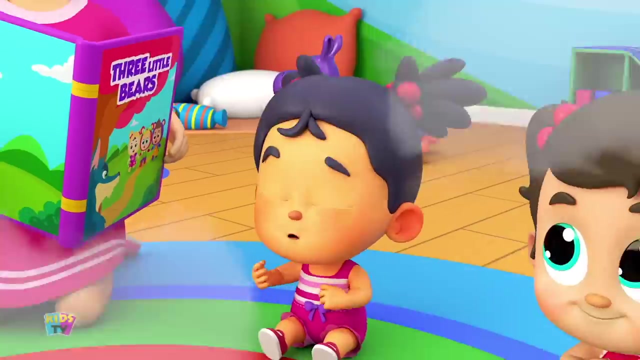 Then I'll huff and I'll puff and I'll blow your house in. And he tried, and he tried, and he tried again. Sheesh, Get a hold of yourself. So did he blow the house in, Not by the hairs of his chinny-chin-chin. 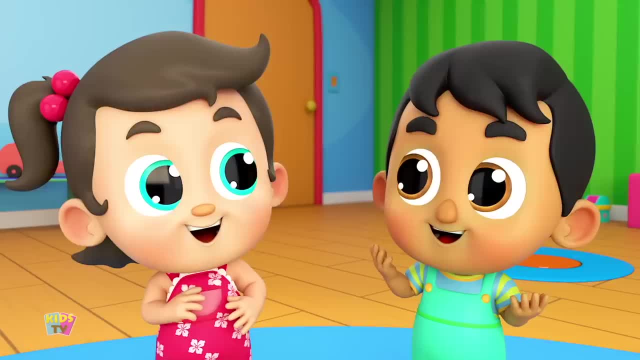 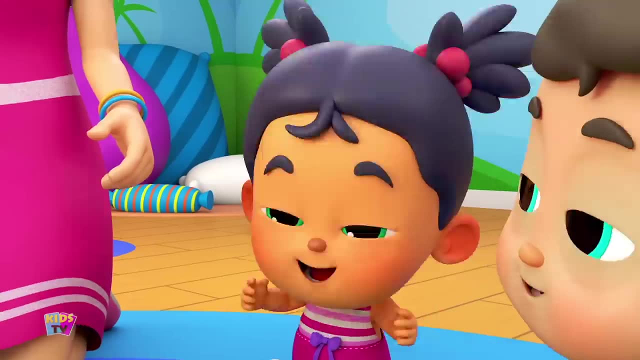 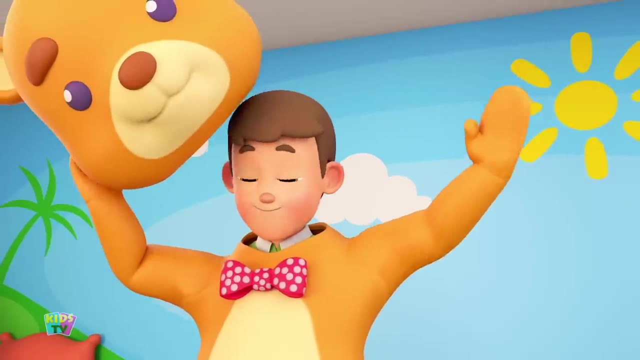 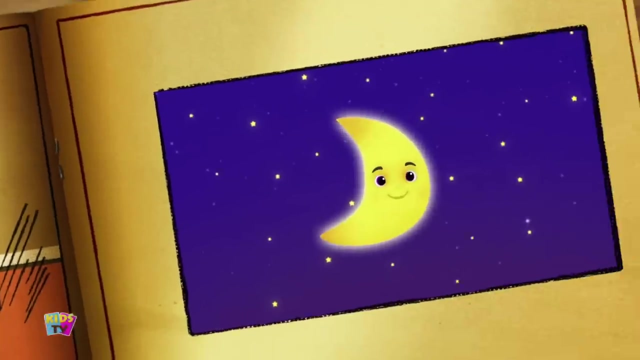 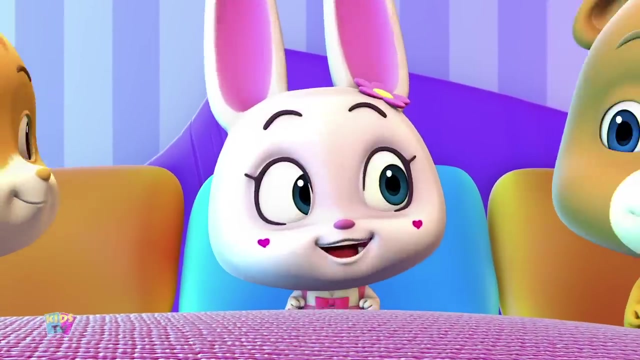 The bricks were too strong. So what happened to the mean old wolf? He was never to be seen again. Wolves are like that. Yeah, they are Boo, Oh, Oh, Daddy. I'm sorry, Mama, let's read the one about Goldilocks. 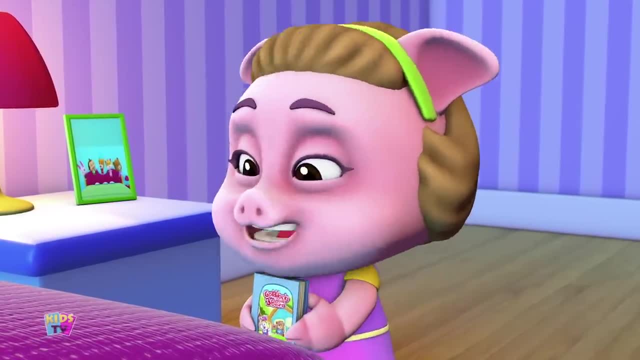 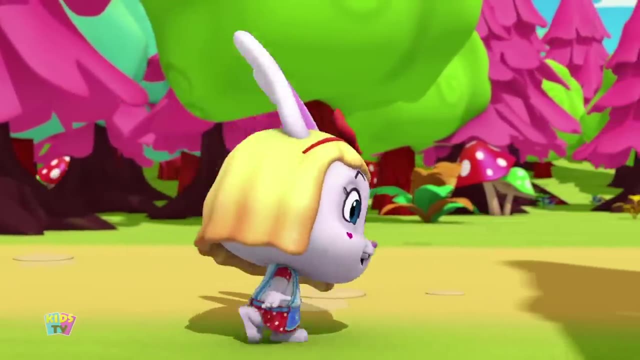 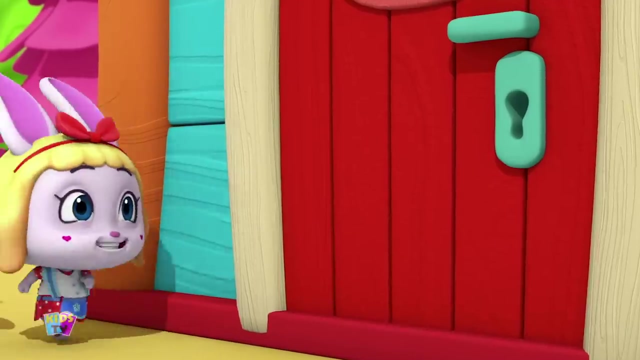 Yeah, Oh yes, Goldilocks and the Three Bears. Well, once upon a time Goldilocks went for a walk And came upon a house in the woods. The house belonged to three bears. I'd like to go in if I could. Well, you don't say. 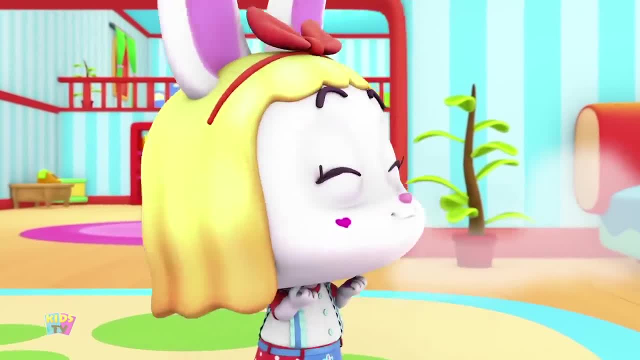 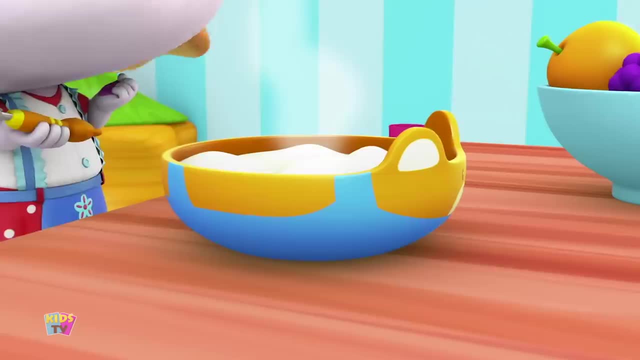 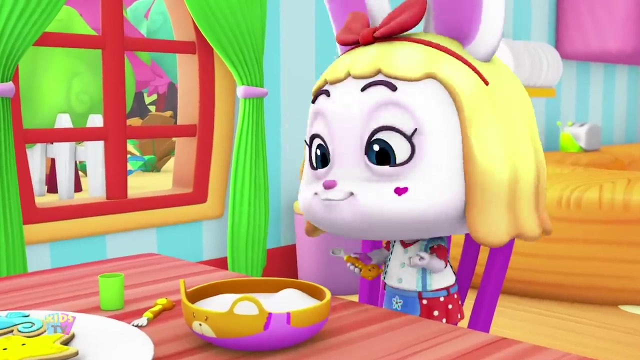 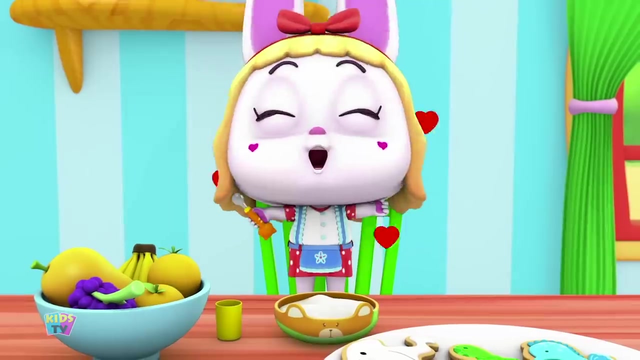 Goldilocks walked right in And found three bowls full of food Porridge. She said: How nice, That's really good. But the first one was too hot, The second one was too cold, The third one, well Behold, Now this one is just right. 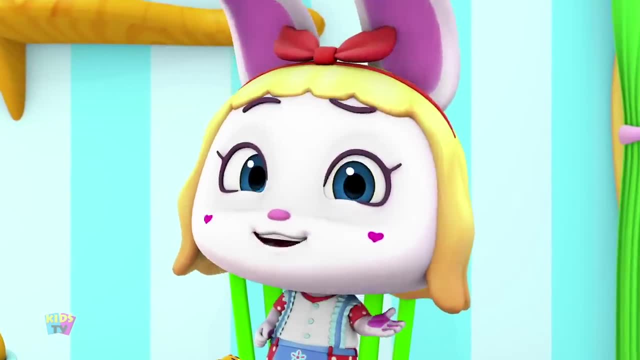 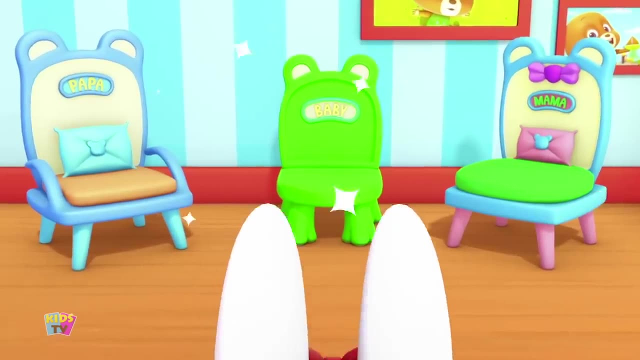 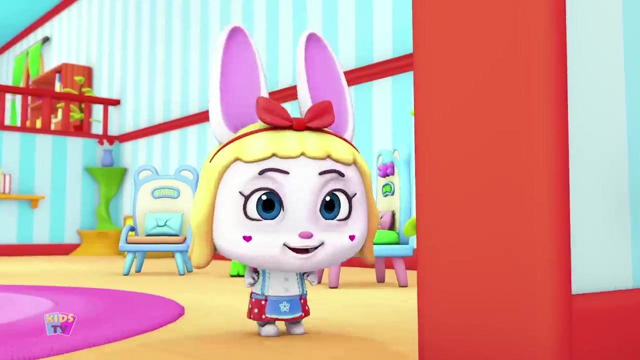 That porridge was yummy. I think I'll go get coffee. Coffee in the living room. Goldilocks went to the living room Where she found three very nice chairs. She had to try them out, of course, But they belonged to three bears. Hmm, this one looks cozy. 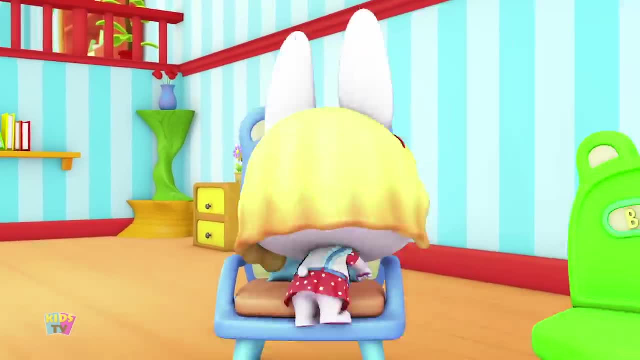 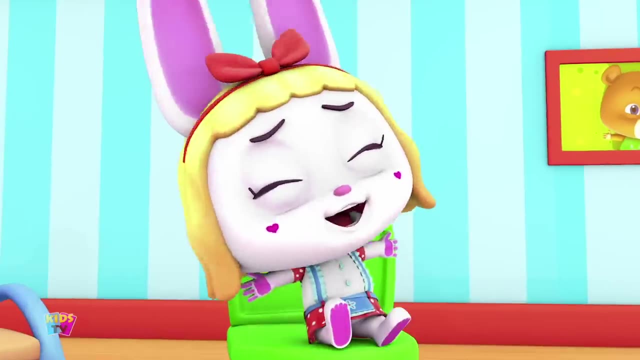 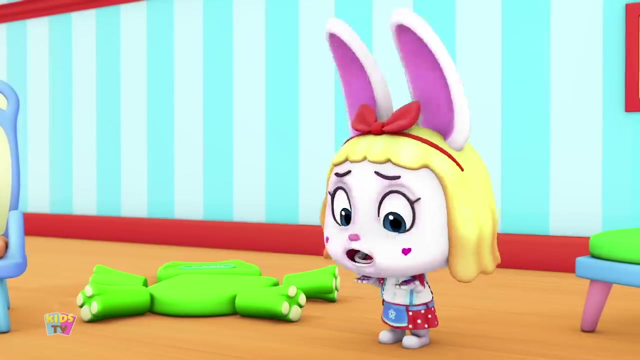 Well, the first one was too big, Oops. The second one was big too, Oh my. The third one was just right, But when she sat it came unglued. Oopsie daisy, Oh dear. Perhaps I just need to go lay down. 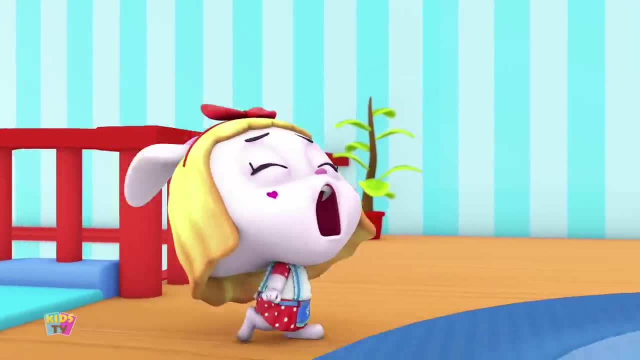 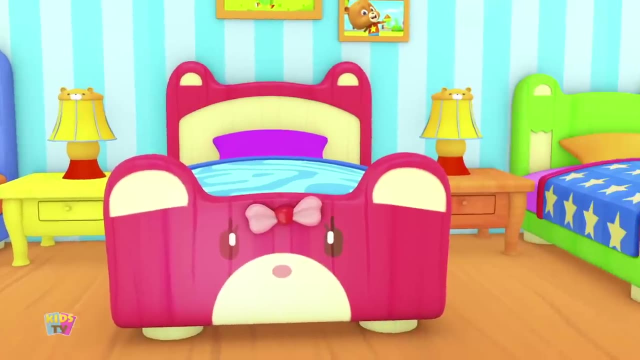 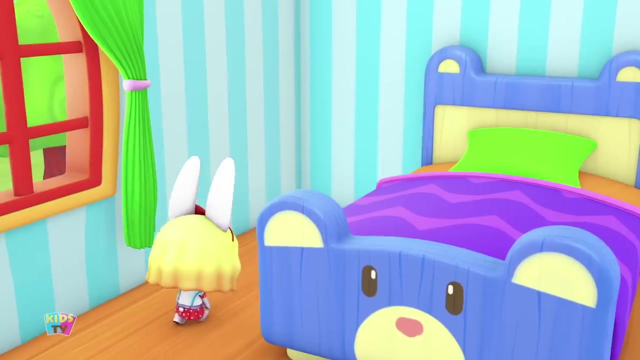 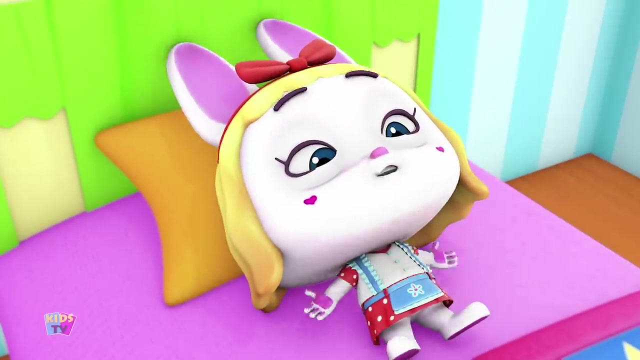 Oh, my Goldilocks went upstairs And there she found three beds. So many choices Where to sleep. I want to rest my weary head, But the first bed was too hard, Ouch, And the second Too soft for me, But this third bed is just right. 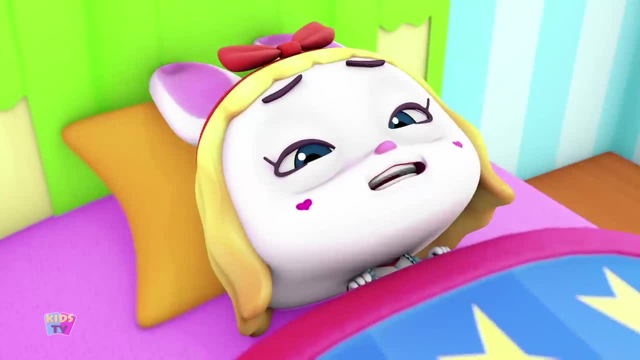 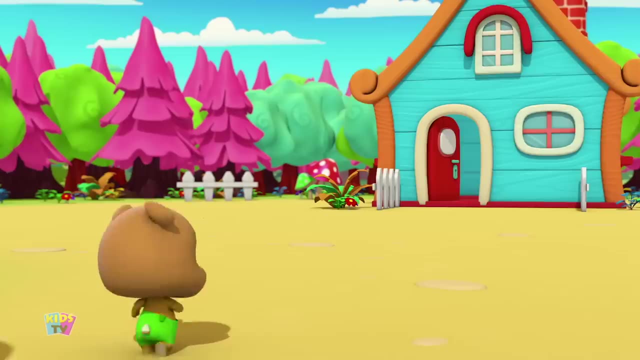 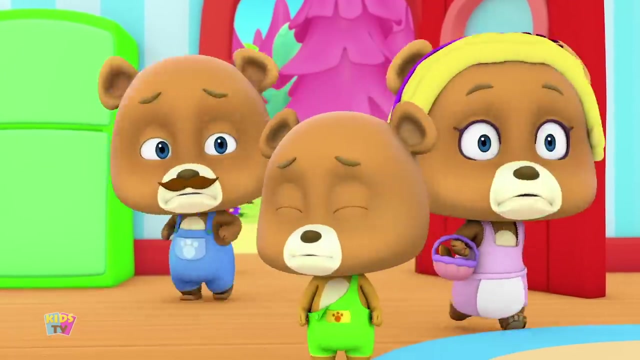 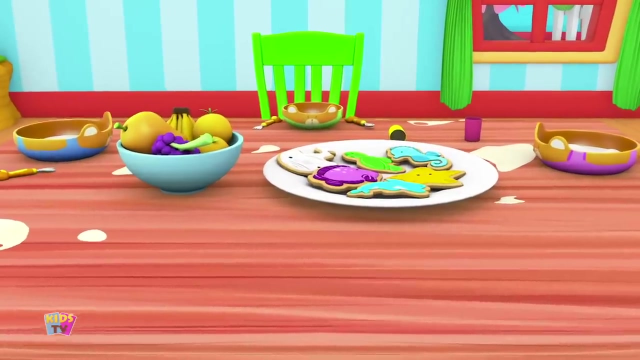 I think I'll just fall asleep. While Goldie slept, the three bears came home And they could not believe their eyes. Oh, And the third bed was open Was someone's bed. What a strange surprise. Oh, my, Someone's been eating my porridge. 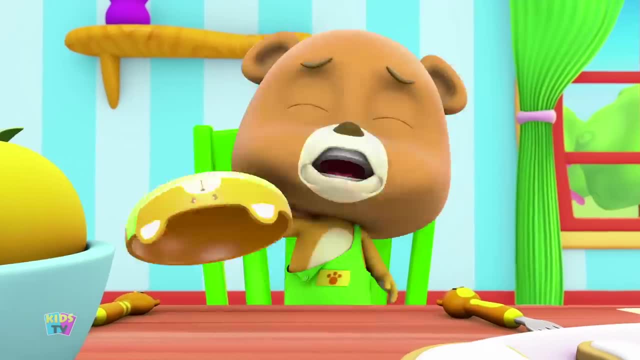 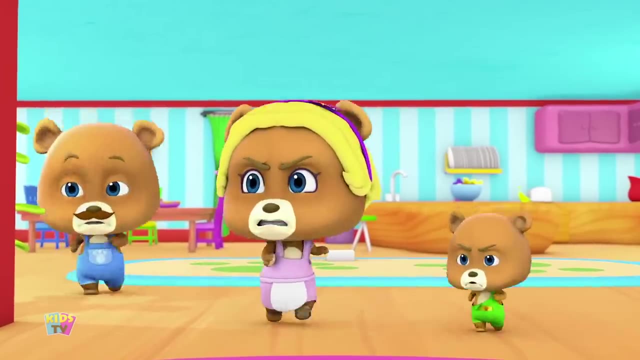 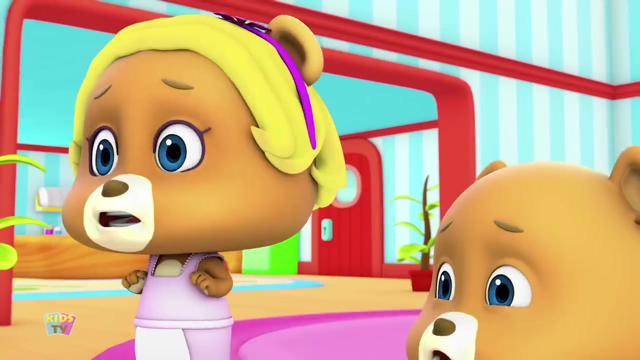 Someone's been tasting mine too, And mine's all gone. Oh goodness me, What's a baby bear to do? Oh dear, Have a look in the living room. Oh, Oh, You see what I mean. Uh-huh, Someone's been sitting in my chair. 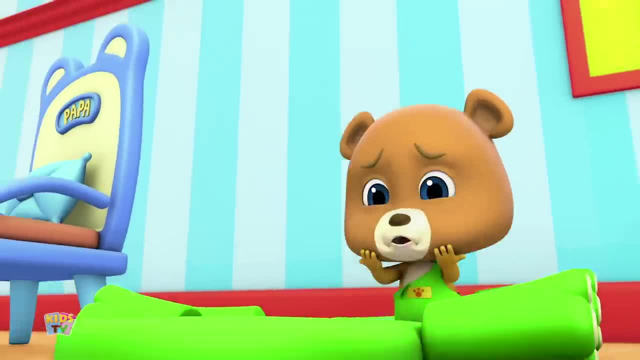 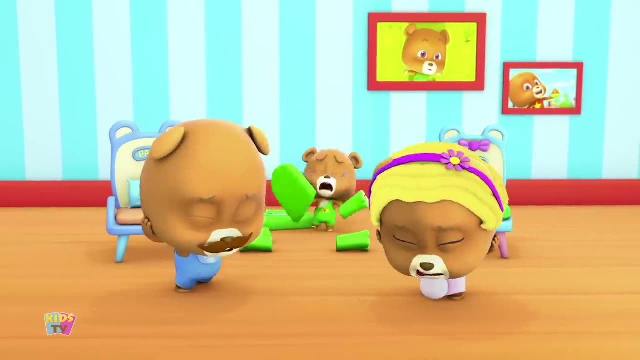 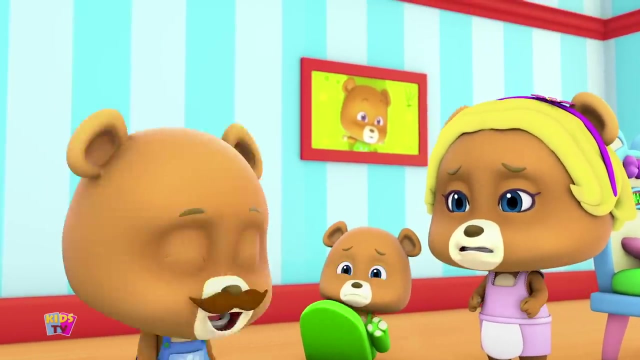 And someone sat in my chair too. Uh-oh And oh, my dear, What's happened here? My chair has come unglued. I think we better go upstairs And see if there's someone up there. Okay, Follow me. Someone's tried out my bed. 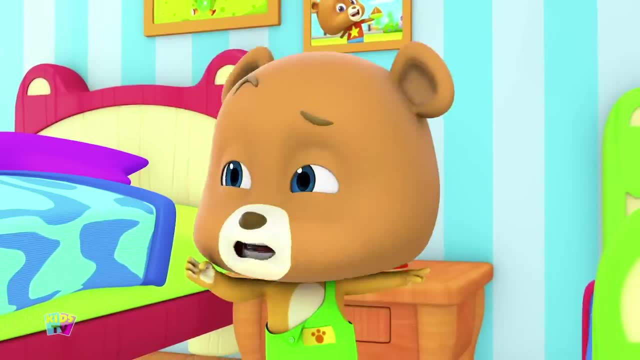 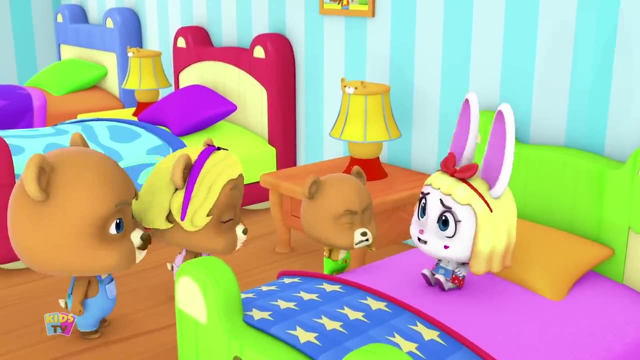 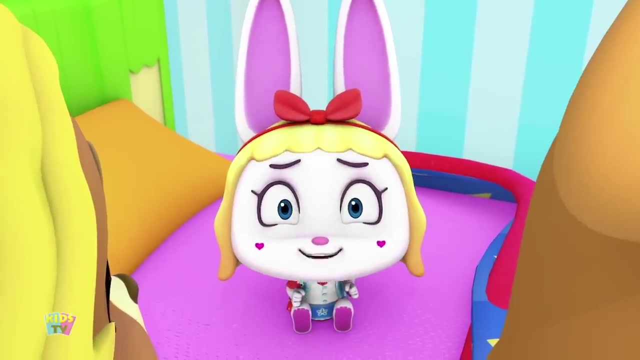 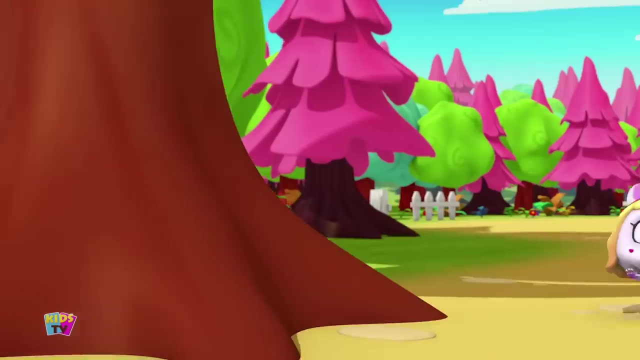 This isn't your average bed. Uh-oh, Someone's been sleeping in my bed And uh-oh She's still there. Look, Ah, I was just on my way out. Bye-bye. Goldilocks ran to the woods And hid in the deep green glen. 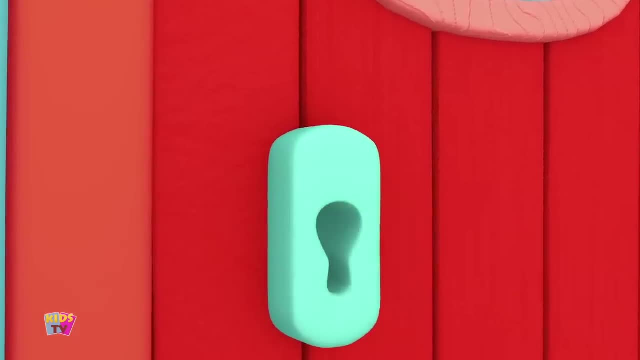 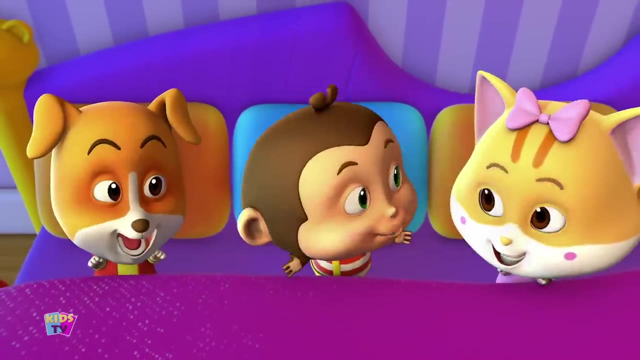 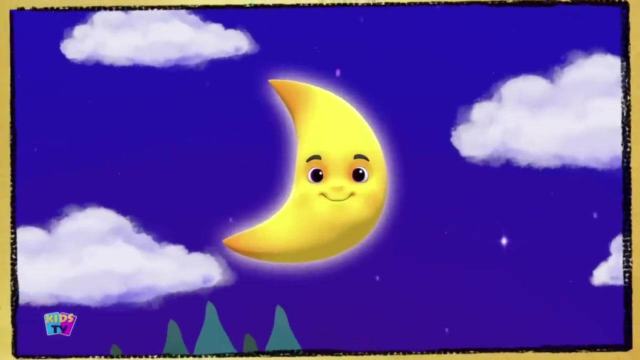 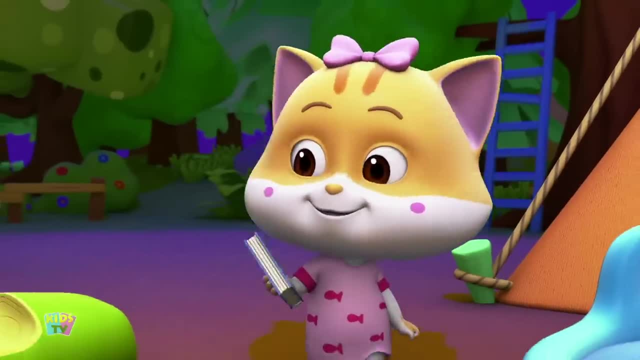 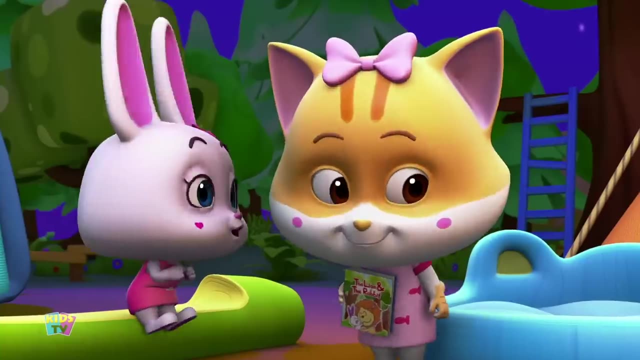 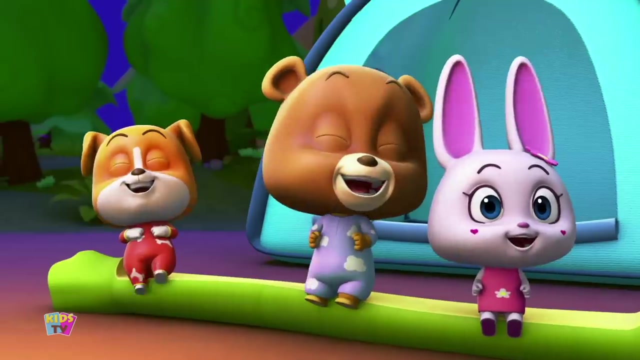 Pfft, Pfft, Pfft, Pfft, Pfft. Hey, Let's hear the story of the lion and the rabbit. Me, I do, I do. Can I pretend to play the rabbit? Well, of course, I want to be the big, bad lion. 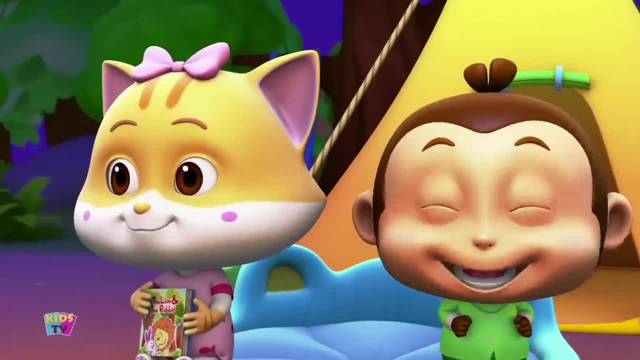 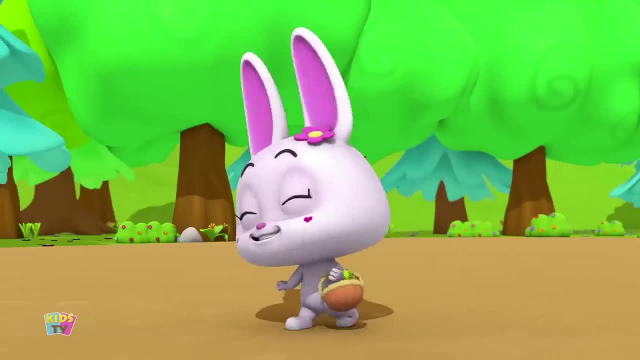 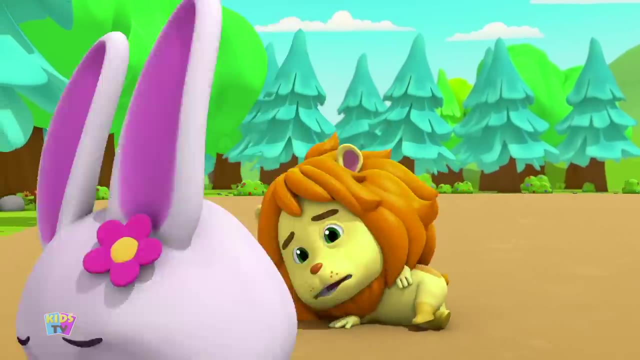 Of course you do. Okay, Here we go. A mighty, mighty lion Lay sleeping in the woods. Along came a bunny From the neighborhood. She accidentally brushed up Against the lion's toes. Oops, Sorry, Mr Lion, She said, and then she froze. 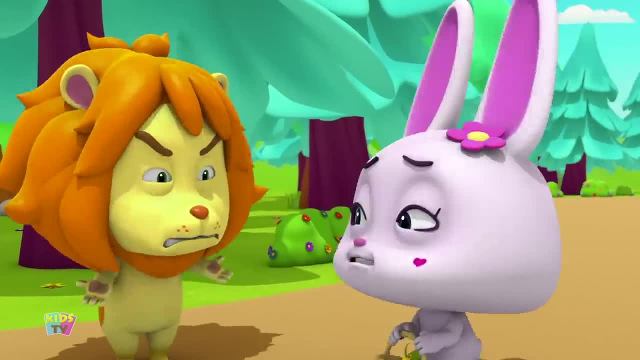 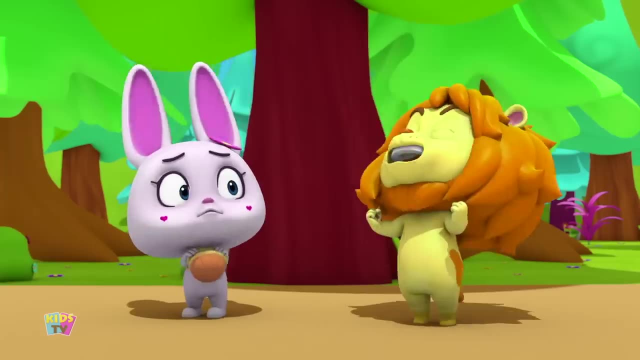 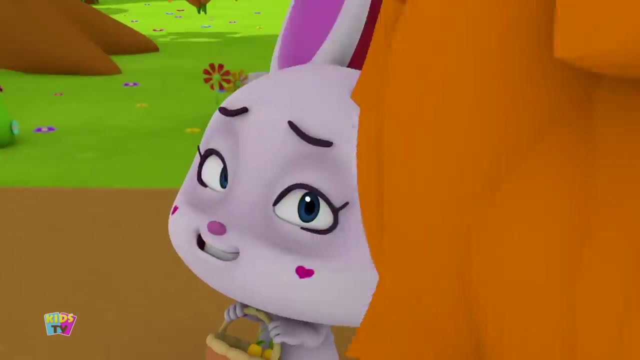 It was just an accident. The lion dropped his paw Smack on the bunny's tail. Oh, Ha-ha-ha-ha, I caught ya. Now you're in lion's jail. Oh please, Mr Lion, Spare me, just this time. 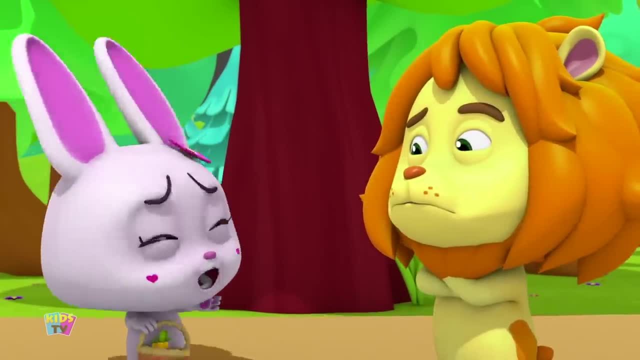 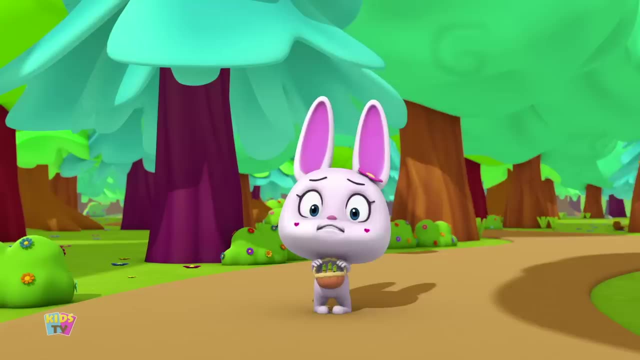 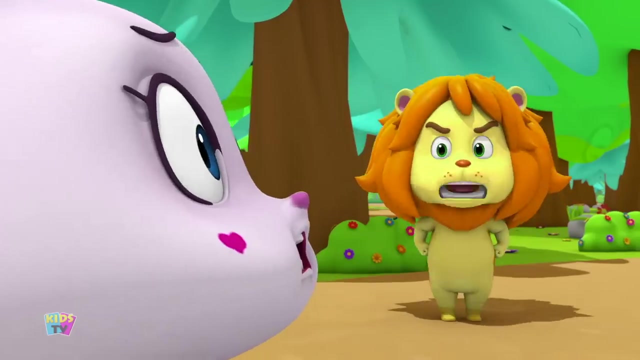 And I promise To repay you Just for being kind. I will, you know. Ha-ha-ha, That's pretty funny, A little bunny Helping me. Well, perhaps I'll let you go, But only just this time. You're just a little bunny With a feeble little mind. 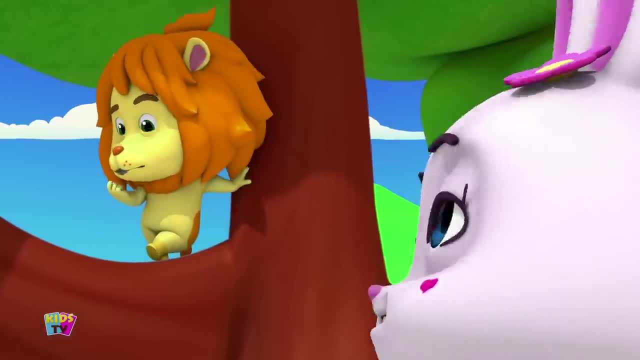 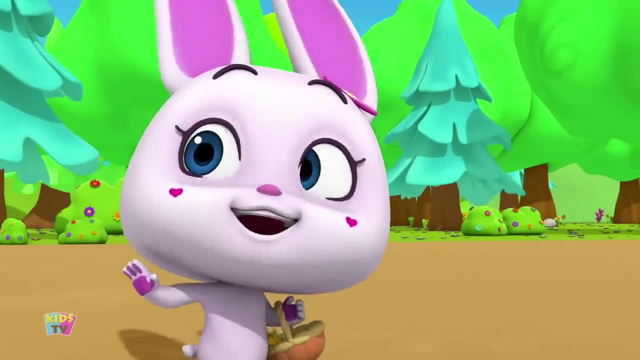 Oh, thank you, Mr Lion. See the smile up on my face. Every act of pride, Kindness, makes the world A better place. You see It already is, And with that The great big lion. Let the little bunny go. That was nice of the lion. 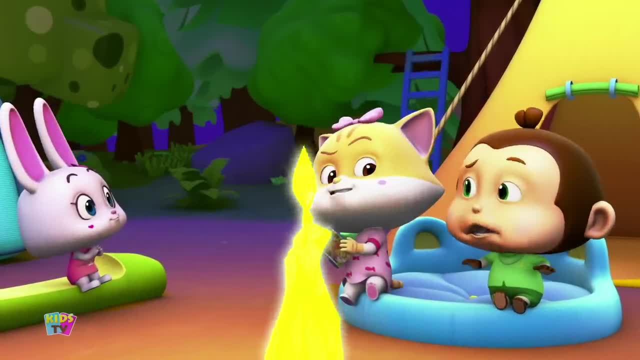 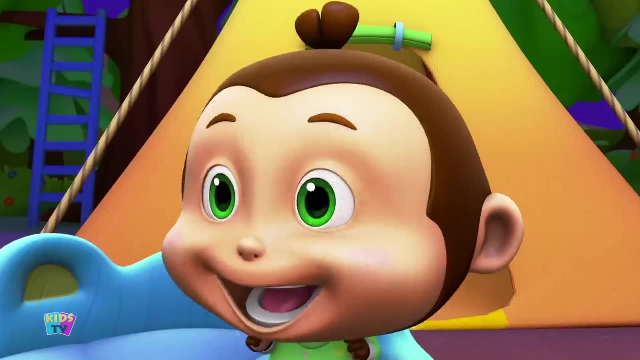 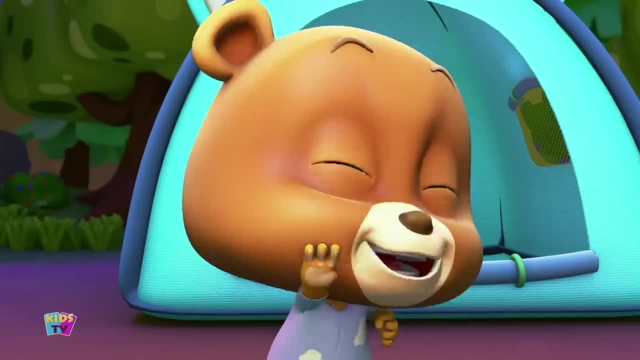 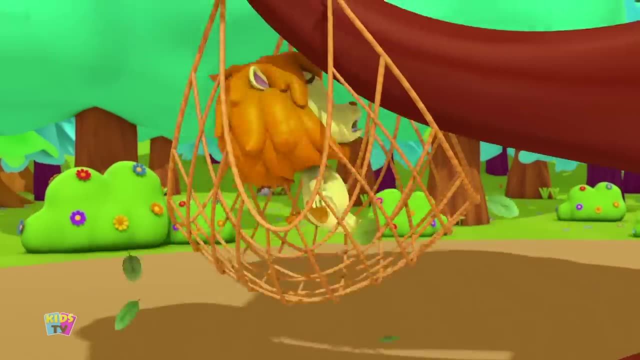 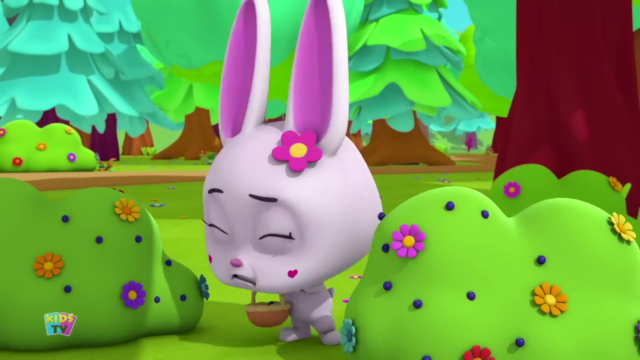 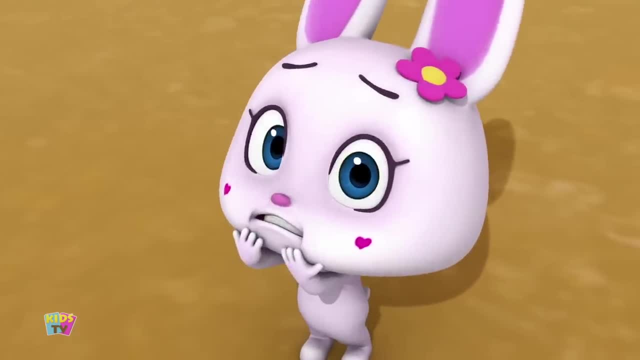 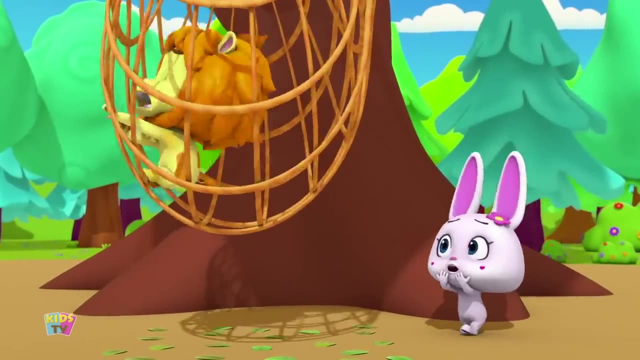 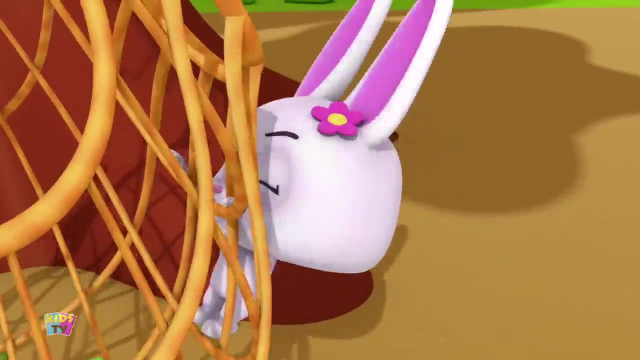 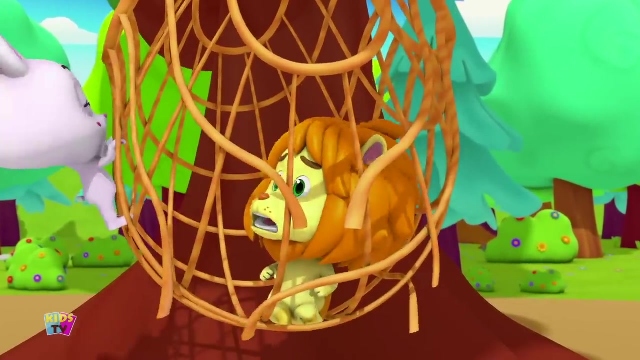 The lion. Oh goodness me, Oh my Poor thing. The little bunny saw the lion in the net And ripped a little hole, and that began to stretch. The hole became so big that the lion made it out. He looked at her in shock and said: 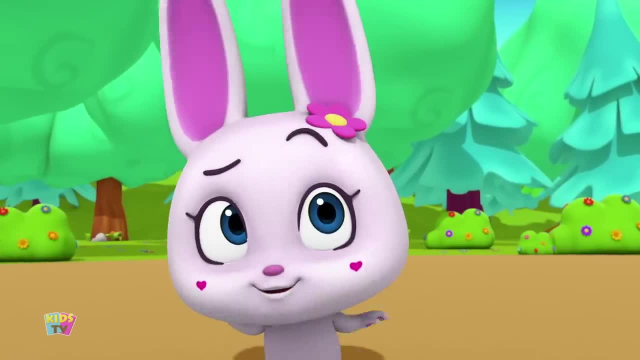 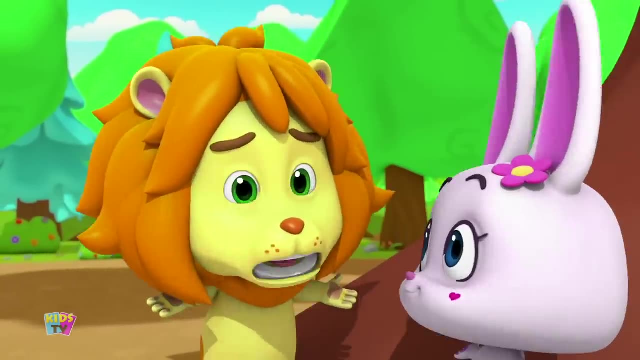 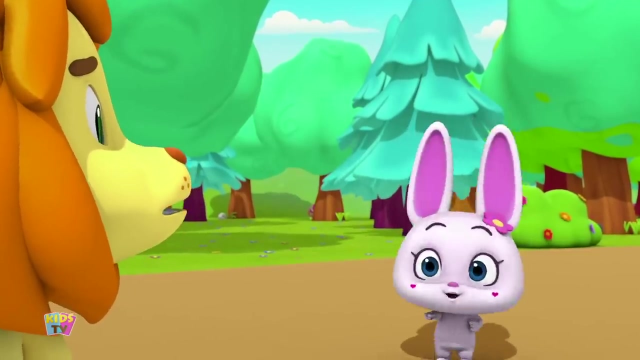 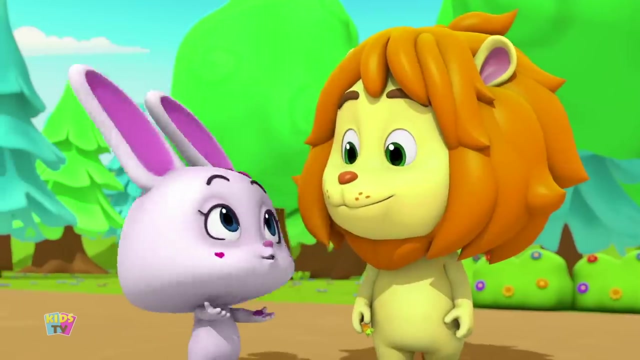 What's this all about? Oh well, that's what friends are for. Whatever do you mean, It's good to help a friend. I always keep my promises to the very end. I told you I'd repay you. Mr Lion see, Kindness is a gift that always sets you free. 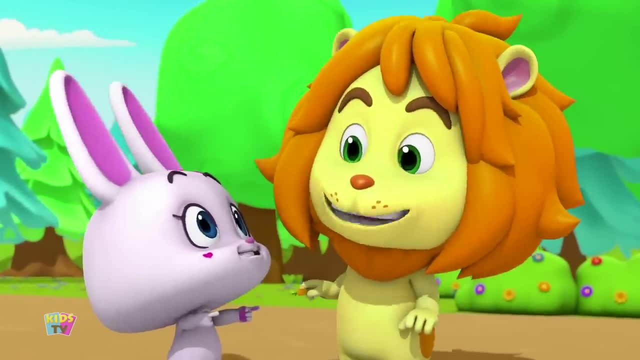 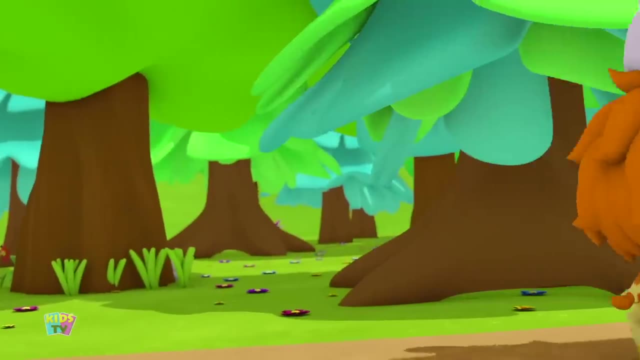 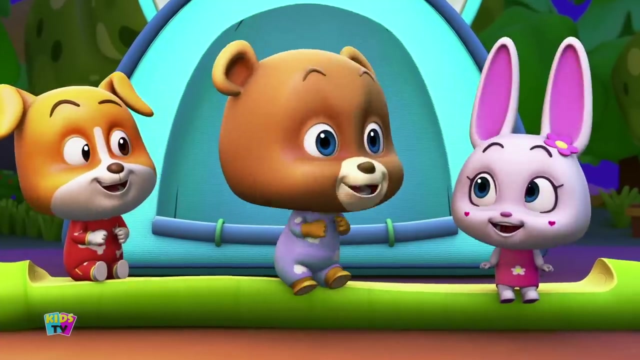 See, you're free. The lion purred And they lived happily ever after Like best friends. Yes, indeedy-do.